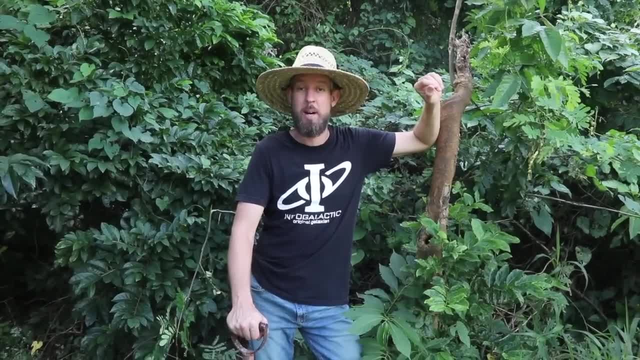 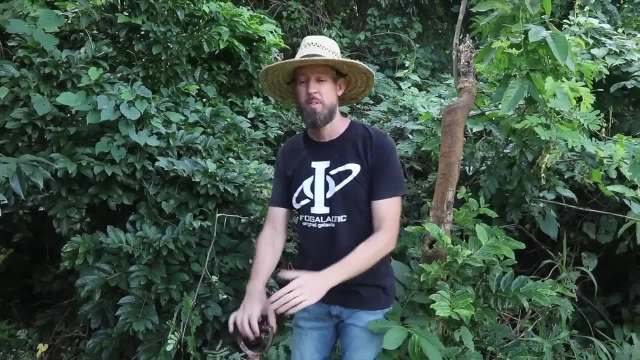 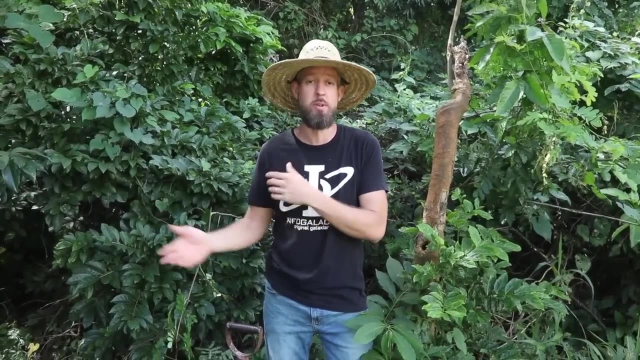 I'm just going to tell you you don't really need to get caught up in buying this and buying that and doing this or that complicated system. You don't need to have cedar boards for the side, You don't need special containers or self-watering doodads, You don't need to even you know. 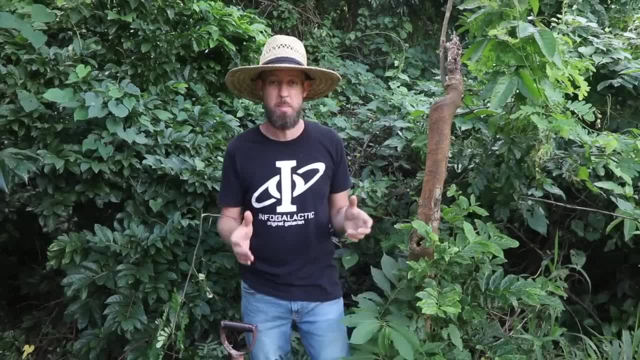 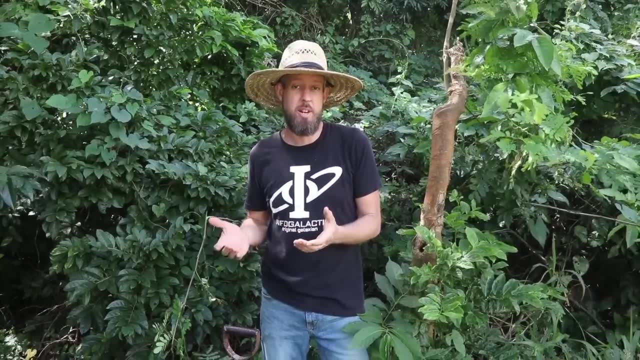 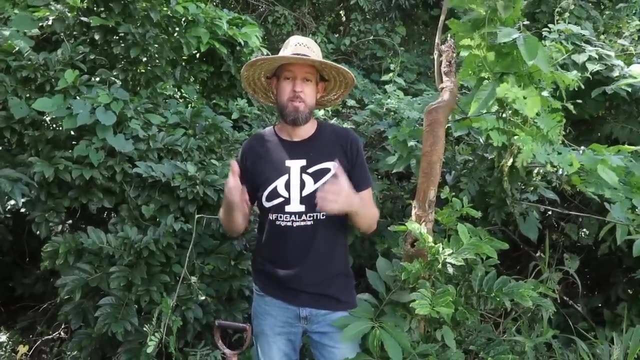 get block or pressure treated and be a carpenter to build a bed. And you especially don't need some sort of big, complicated aquaponics system. All you really need to garden is a patch of soil, got some sunshine, got some water, got your seeds. 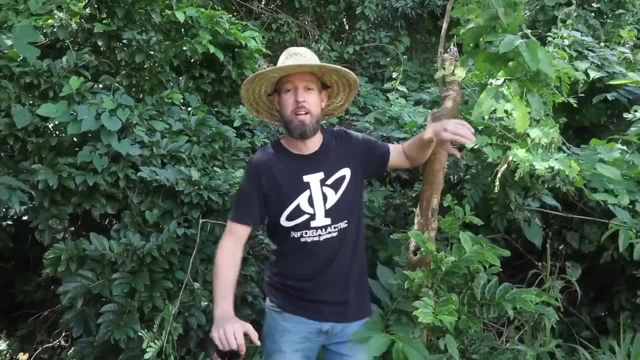 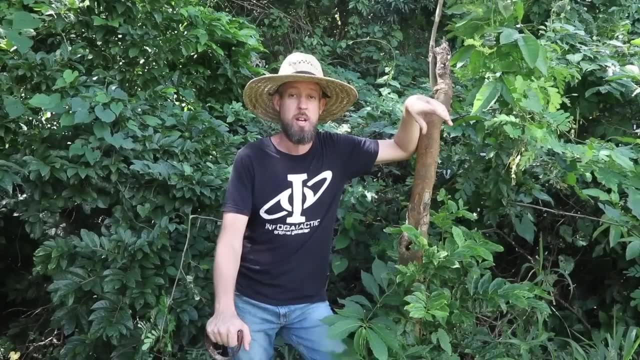 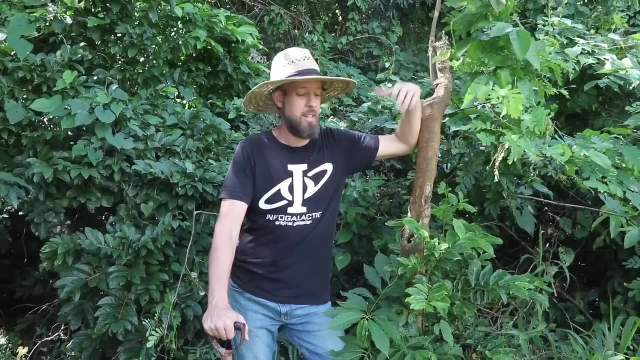 and you just have to feed it with something along the way. So nature does all of that. as you can see behind me, This is an uncut piece of tropical rainforest. Some time ago this was probably all sugarcane in here. This is part of a big plantation- lots of sugarcane, And then, you know, the farmers moved on and guess what? 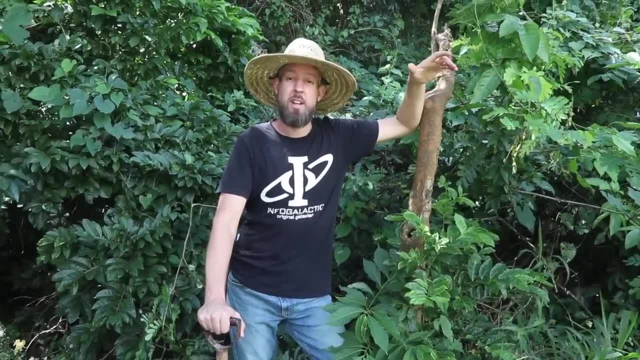 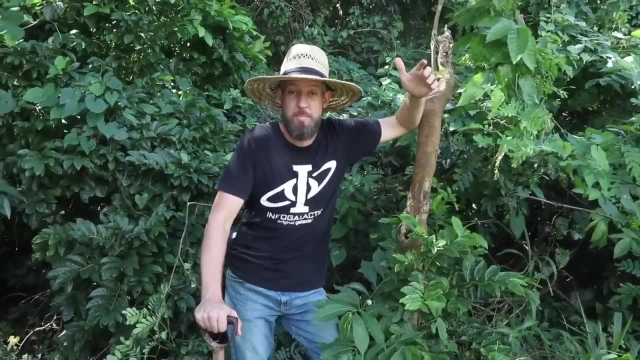 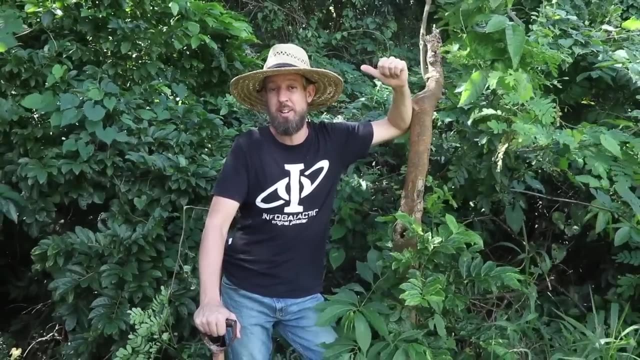 It all grew back. Why is it that our gardens are so complicated and hard and we think we need all kinds of things, But plants grow right on their own. There's a few reasons for it. obviously Our vegetables are more high maintenance than a lot of things growing back here in the jungle. But even with that we can kind of short circuit the process a little bit. 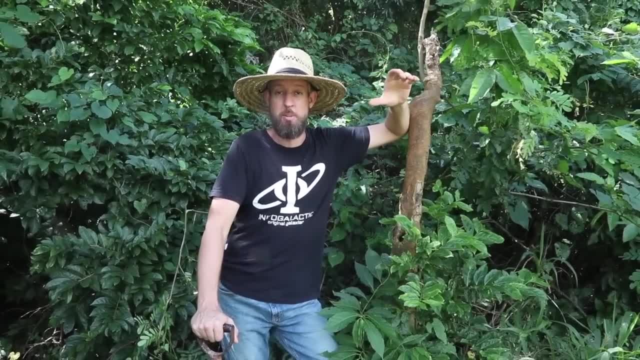 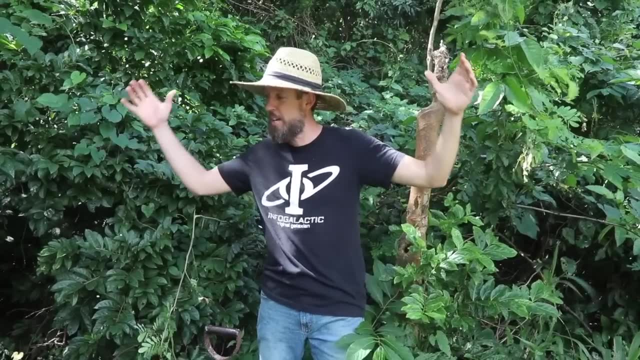 We can make some little shortcuts to do things affordably And in a very non-complicated and simple way. I always like to take something big and complicated and say: what can we get rid of? How can we simplify this big mess? So that's what we're going to do. 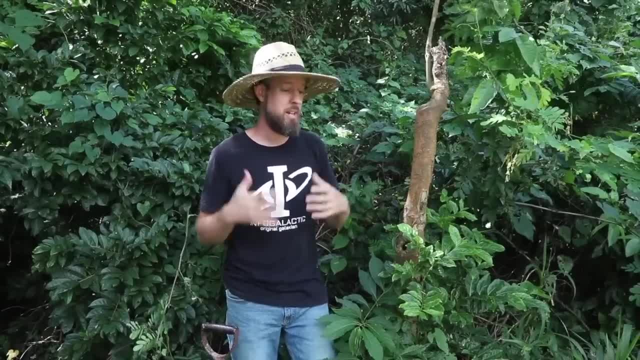 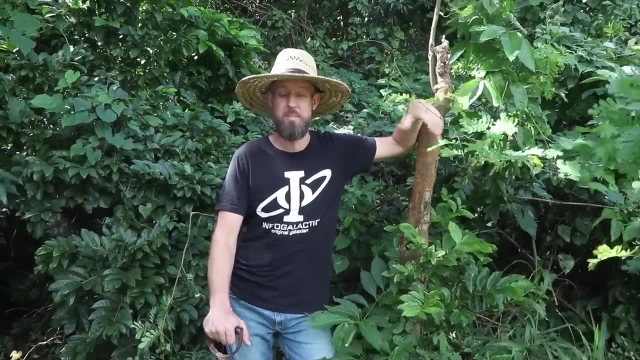 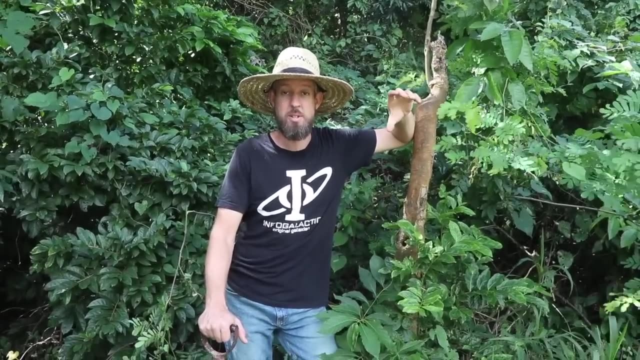 Today we're going to simplify this big mess, And this is a perfect time because I just moved to my own land. After years of renting and being stuck borrowing land and, you know, farming on other people's plots, I finally have my own piece, So I'm going to put in some permanent garden beds. 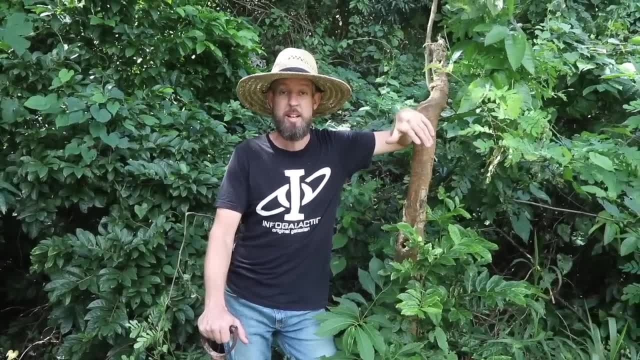 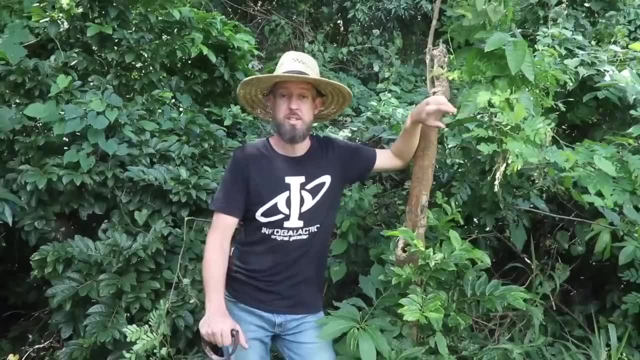 where I'm going to grow my own food to feed my family, And so this is a time I think it would be perfect to take you guys along and show you how do I start this thing from scratch. So let's walk through it right now. 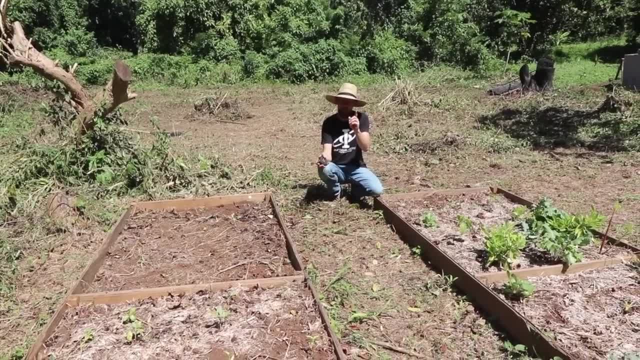 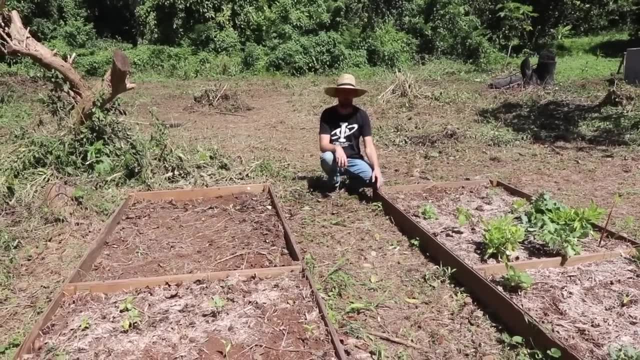 These two beds that are right here Now. I told you, guys, you don't have to put any borders on the beds. I made these out of scrap wood, I don't know. six months ago or so, We stuck a couple of beds in here and put a few vegetables on them. 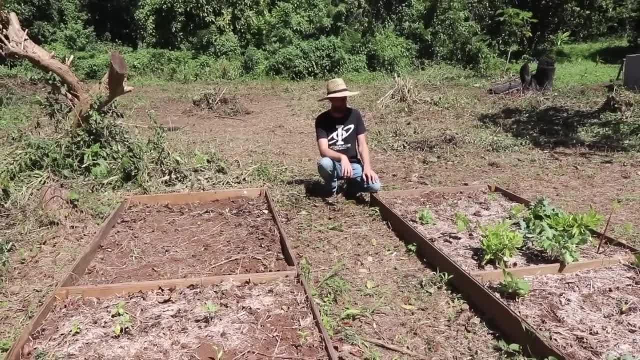 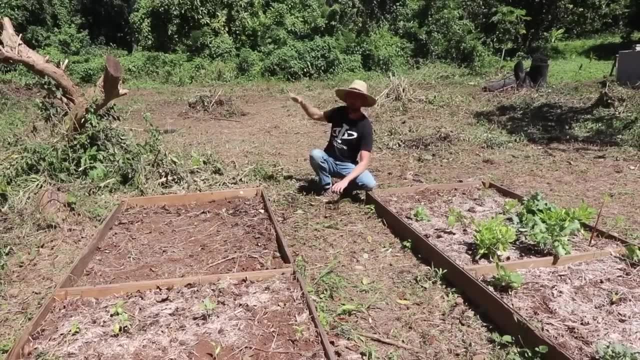 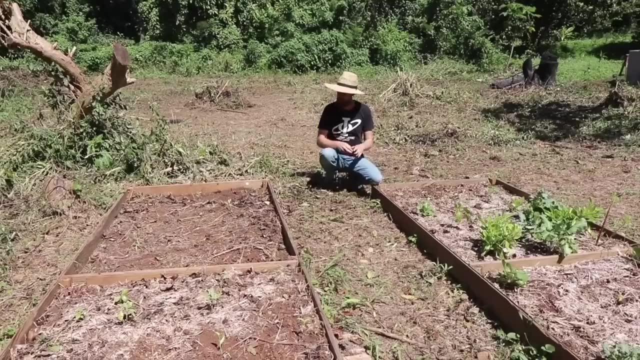 They're mostly tapped out And I just handed them over to a couple of my kids to replant. They were, as of a day ago. this was all like brush, like this tall, So these got cleared and weeded. The few things that were still edible in them got weeded around and the kids have replanted transplants. 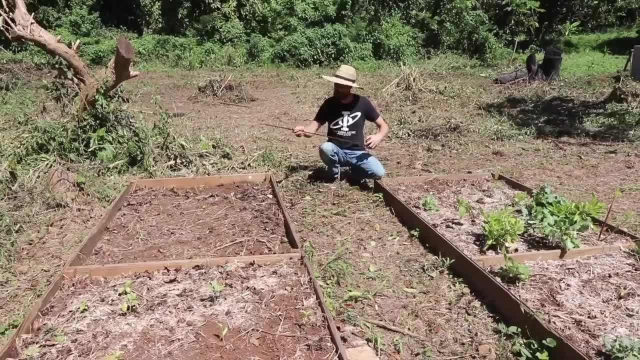 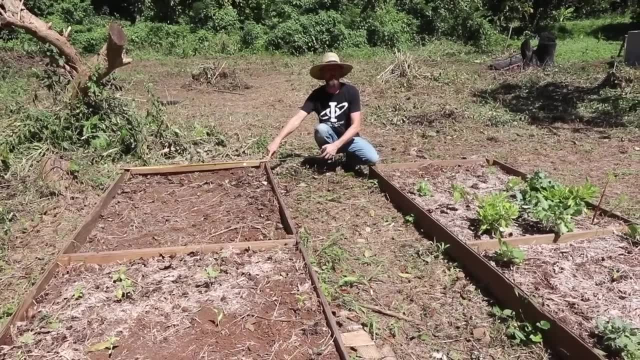 But I am going to continue this line that I started here, because I'm not a complete anarchist. These beds are four foot wide. Now, John Jeevans, the Grow BIOintensive guy, means that we have three beds here And we're going to put in two beds, one of which is a hundred square meters. 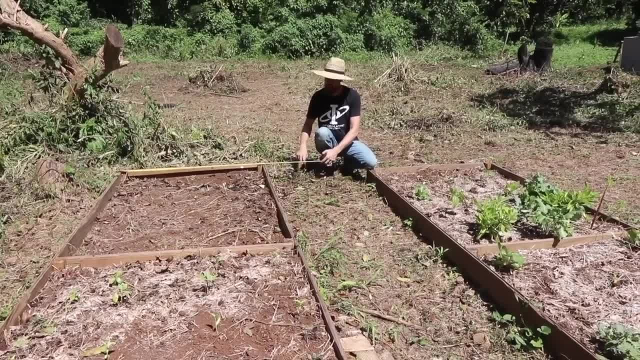 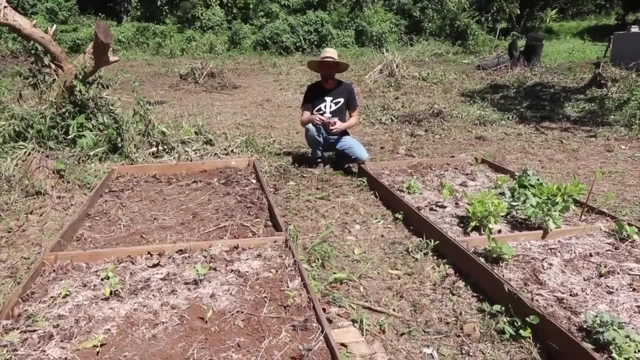 guy. He likes 5 foot beds. I don't like 5 foot beds. He likes 5 foot beds for the microclimate that it creates when all the leaves touch and all that kind of stuff. I'm not that fancy. I like a 4 foot bed because I can reach half way this way, reach half way the other way. 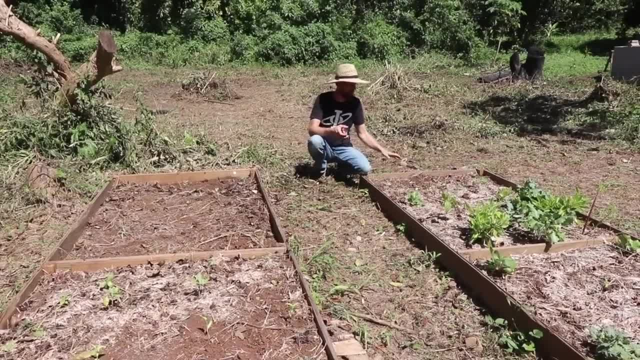 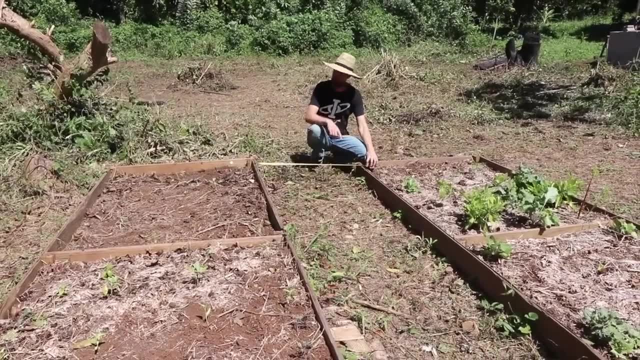 and even kids can get in there and weed it without having to like step down in the middle and that sort of thing. So I like a 4 foot wide bed- if I'm going to do beds, And then these have a 3 foot wide path. Now, 3 foot wide is nice, particularly when you have stuff. 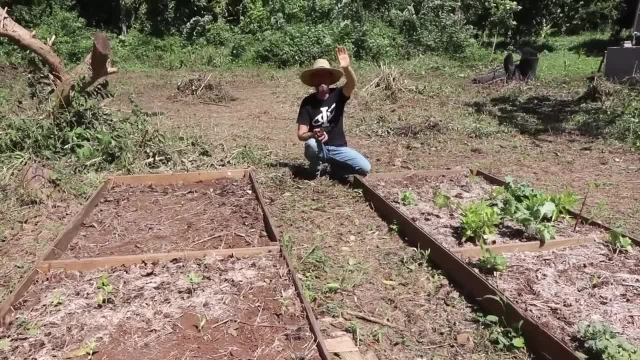 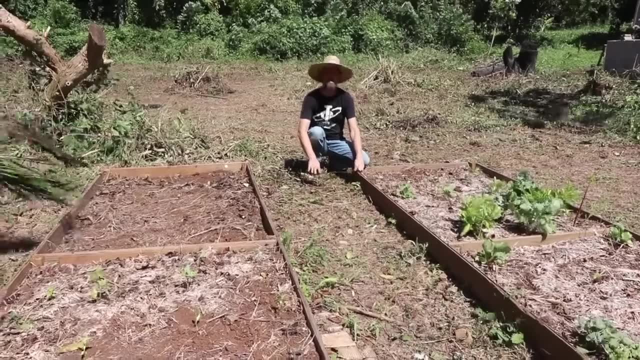 that runs over the edges, Like if you grow a tomato plant next to the edge, the tomato plant is going to come up like this and you go walking sideways. I've seen people do 1 foot paths in between their beds. You got a 1 foot path. you're going like this And when you have these edges it becomes almost a hazard. You're like going back and forth almost tripping over it. So I wouldn't go any more narrow than 2 feet. 3 feet is really nice because you can have a couple people. 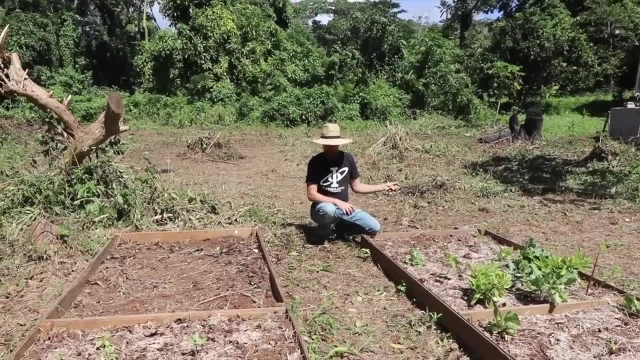 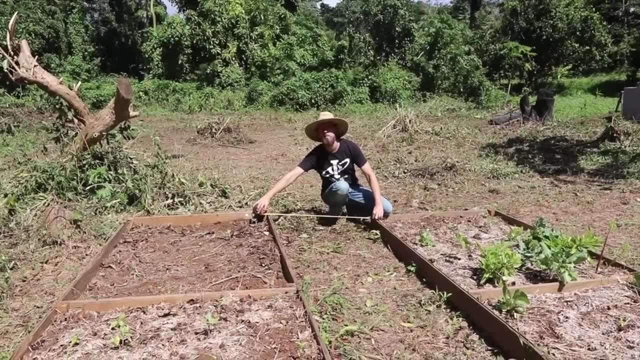 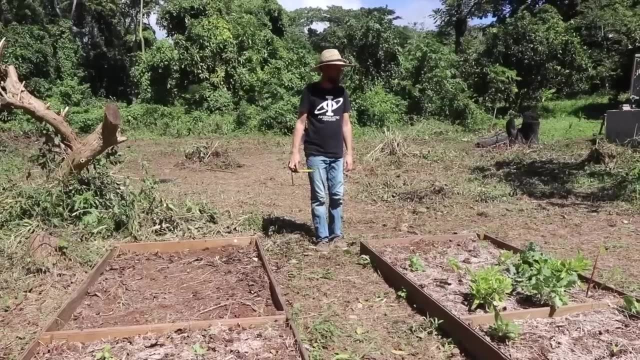 weeding at the same time in the bed and you're not running into each other. Or if you're like really fat, you know great, You can hit the golden corral and come home and weed. So 36 inches is what I got here. I might go down to 2 foot here, because I'm just going. 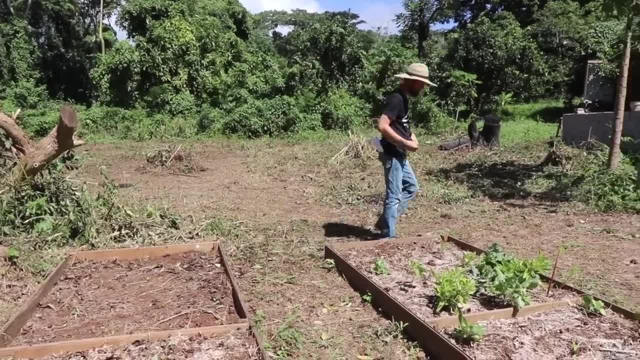 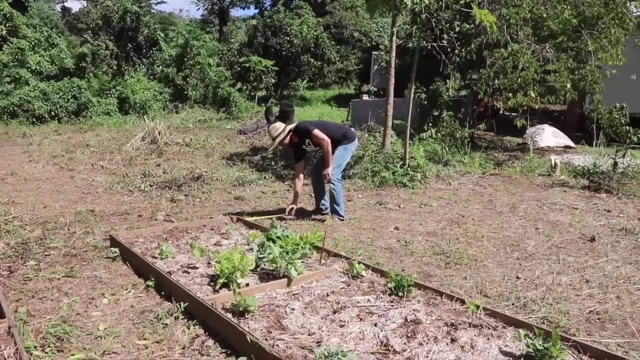 to be doing some dirt beds. Let me show you how I'm going to do that. I'm just going to go 2 foot. Okay, 2 foot takes me out like there. Now, that's still a decent path right there, So I can. put one bed here, go 4 foot. See, there's my 2 foot 4 foot right here. I can go another 2 foot and then I can fit one more 4 foot bed. If I go full 3 footer, I'm not going. 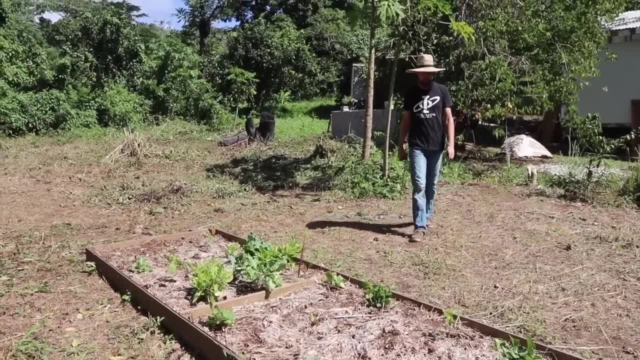 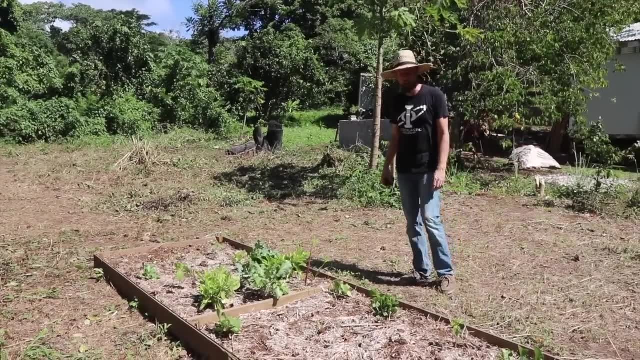 to make it. So I'm going to cheat a little bit and do 2 foot 2 foot wide on these guys. So first thing I'm going to do is build this bed right here. I'm going to mark the corners so I know my spacing before I start digging. 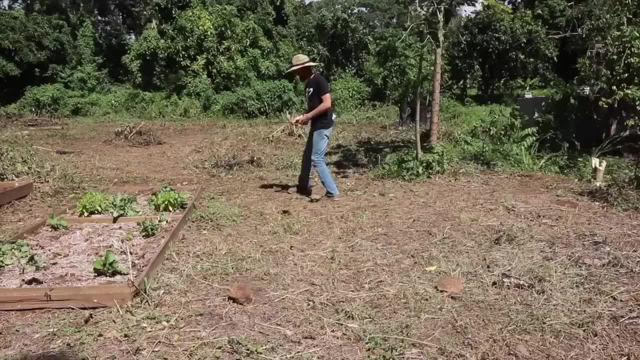 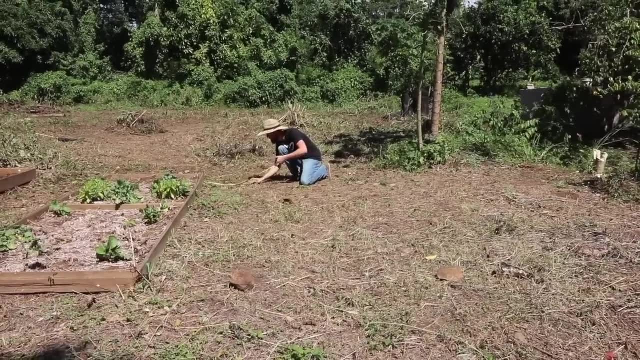 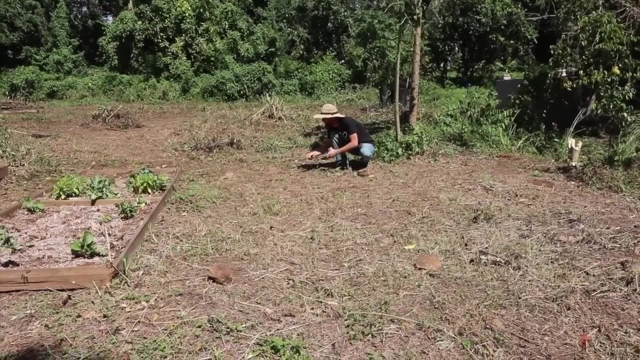 I'm going to mark the corners, I'll mark the corners and then I'll mark the edges. I'm going to mark the corners and then I'll mark the edges. So I'm going to mark the corners on this side and I'm going to mark the edges on this side. 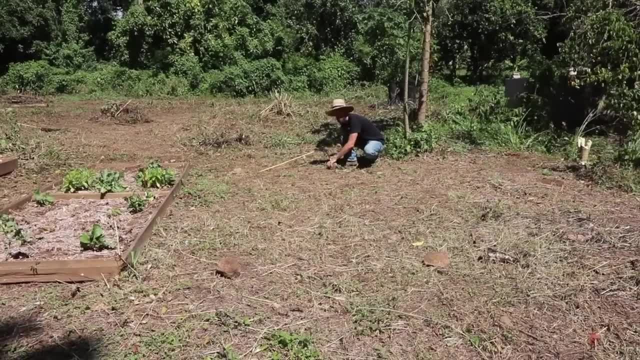 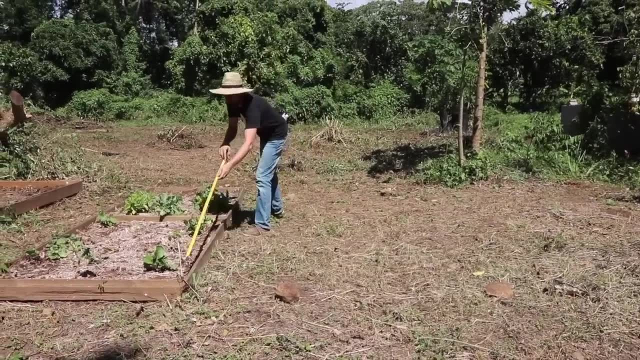 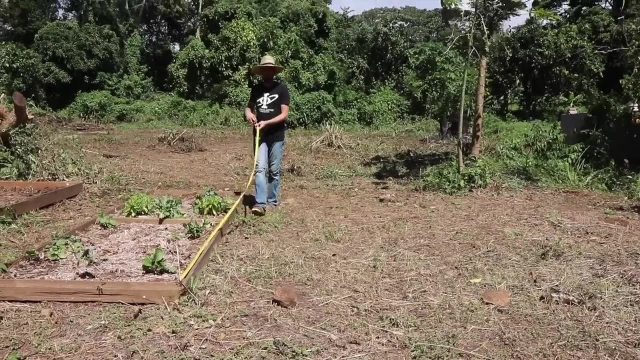 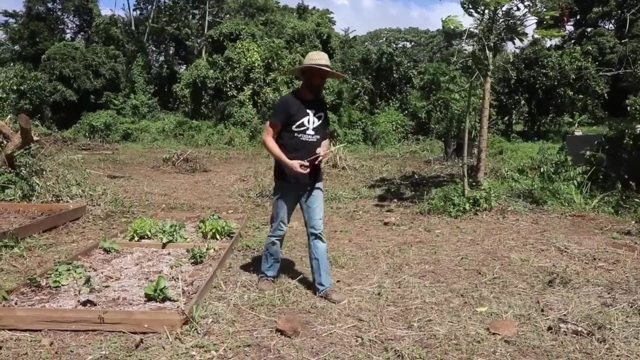 Okay, 3 foot, There we go. I can go a little bit further. See that. Yeah, Oh, it's a four by let's see, Four by 12, that'll grow you a lot of vegetables. Let's dig it. 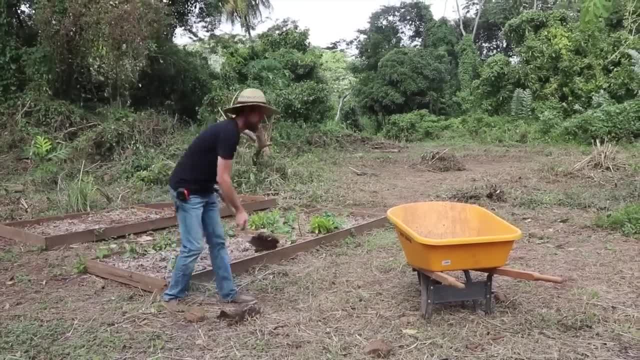 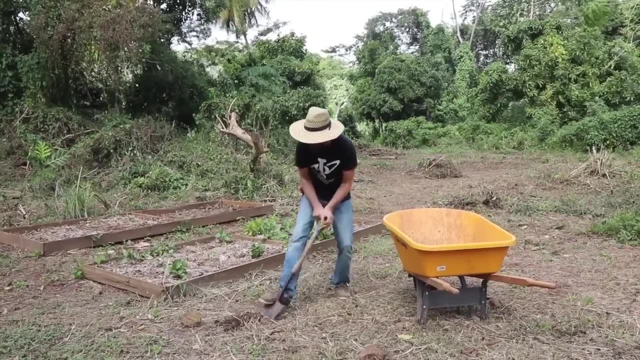 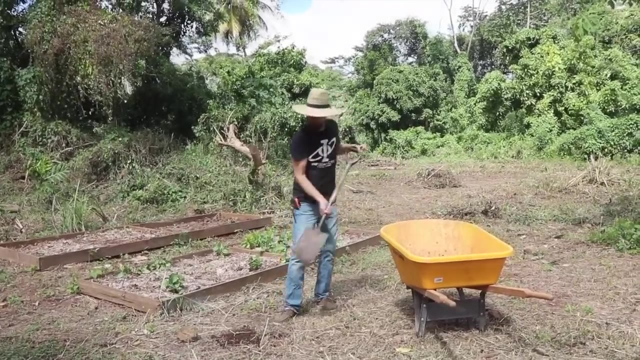 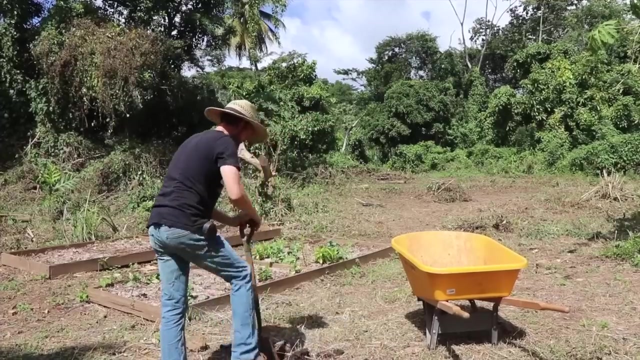 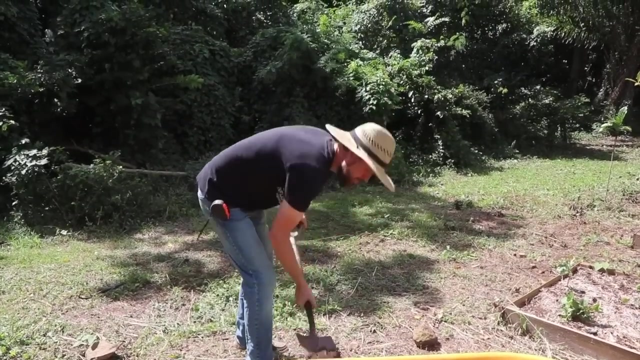 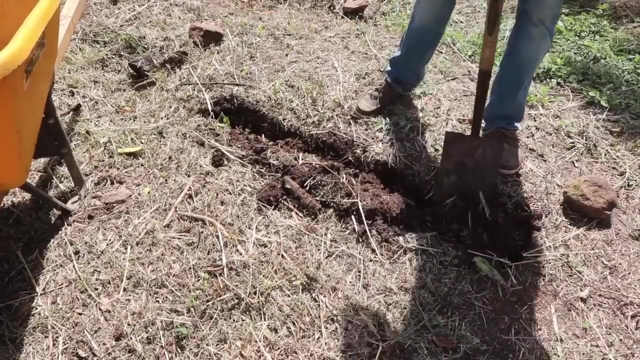 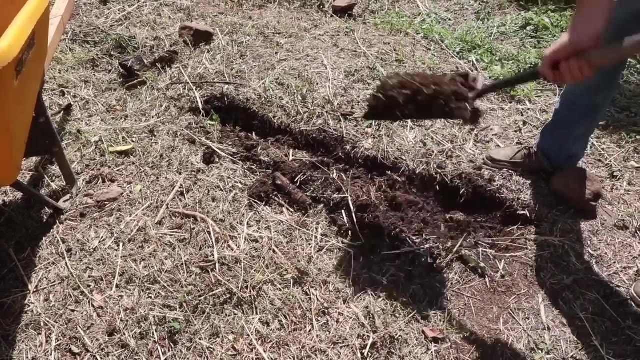 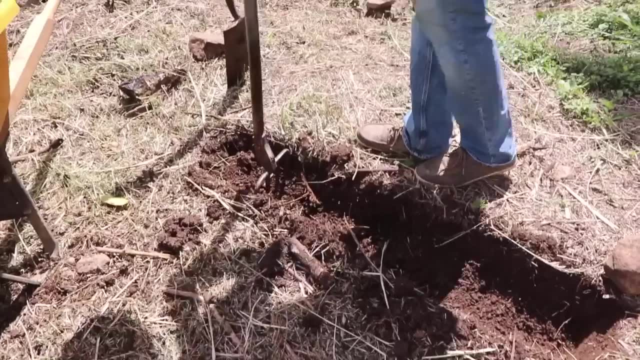 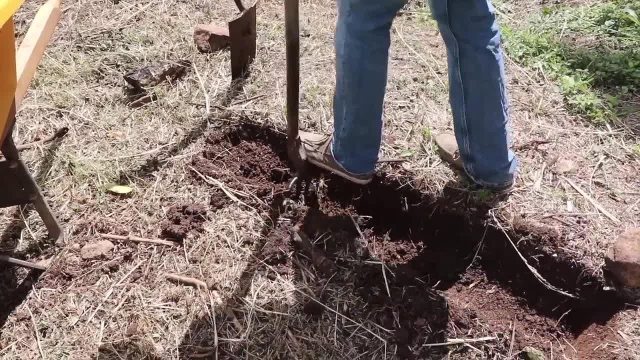 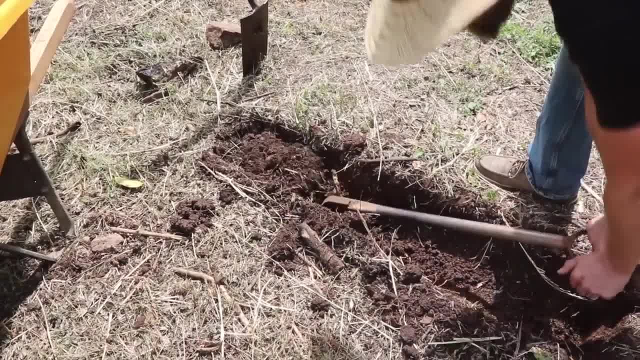 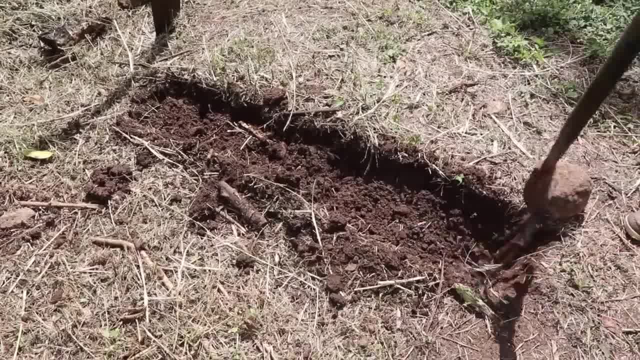 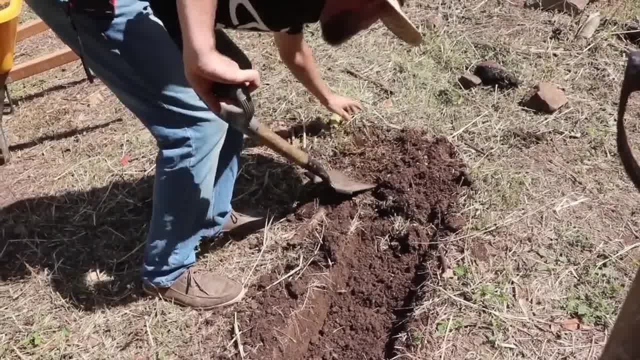 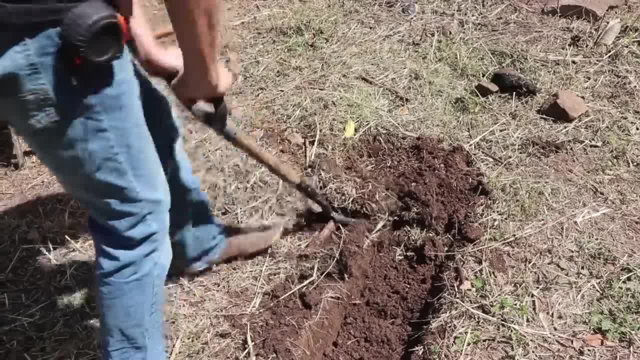 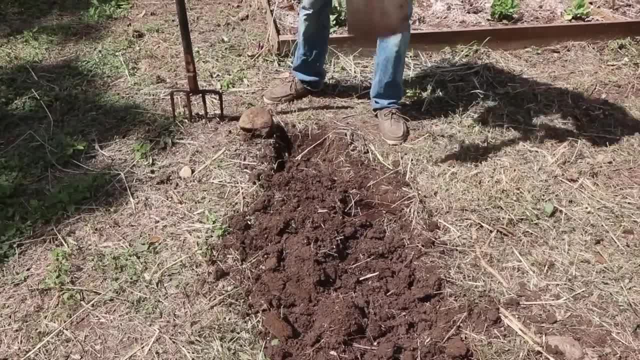 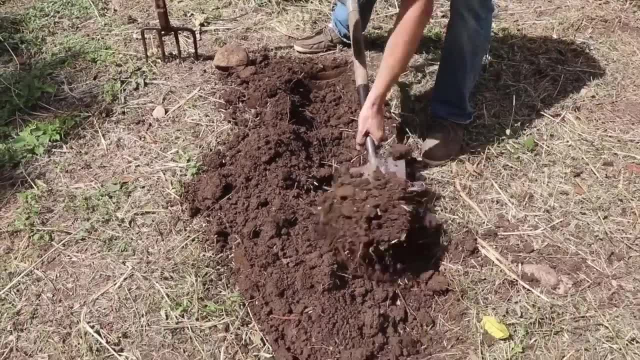 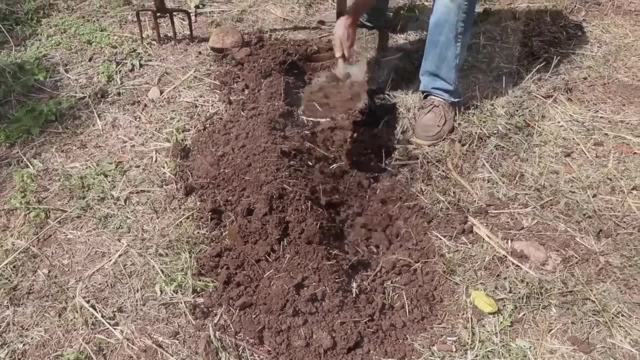 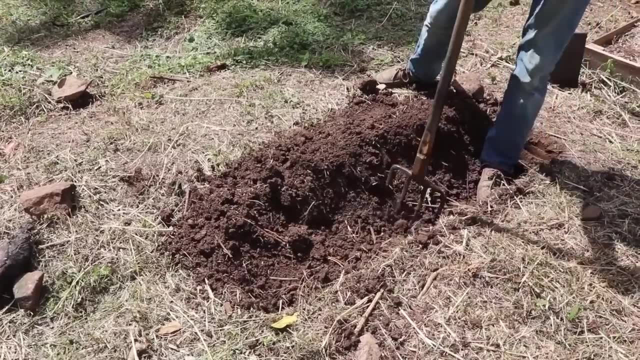 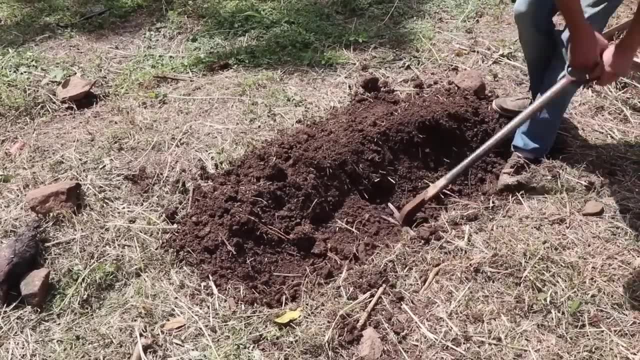 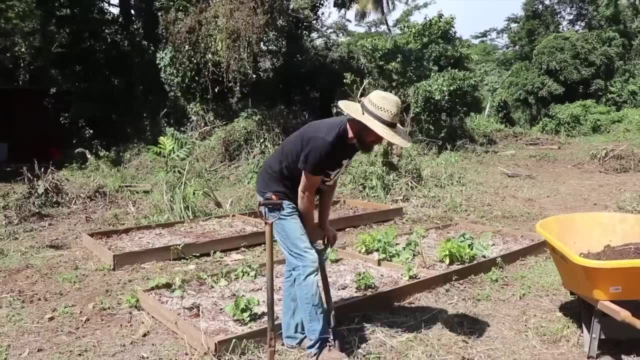 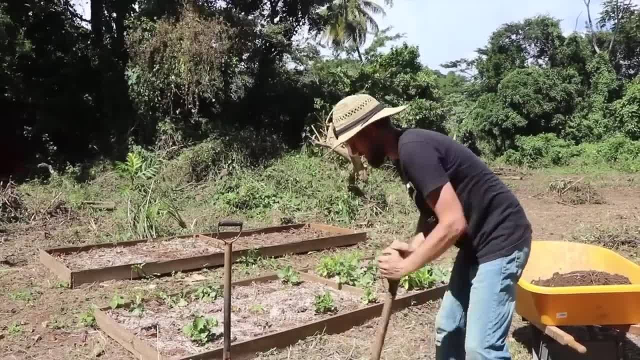 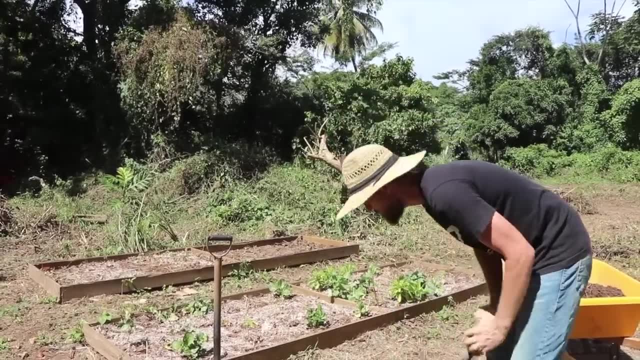 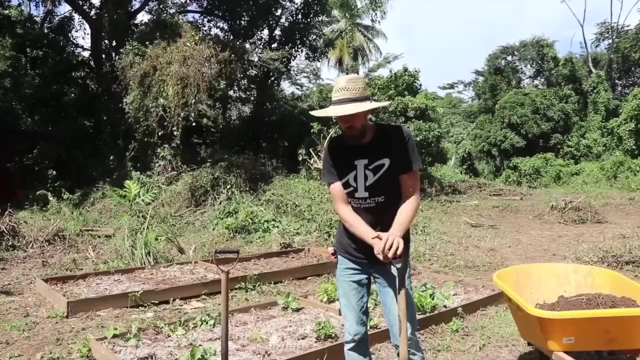 and then you turn the next one over into it and it's a lot of work, Really a lot of work. It loosens the soil quite deeply, Makes for the most amazing garden bed you've ever seen, but it's a ton of work. 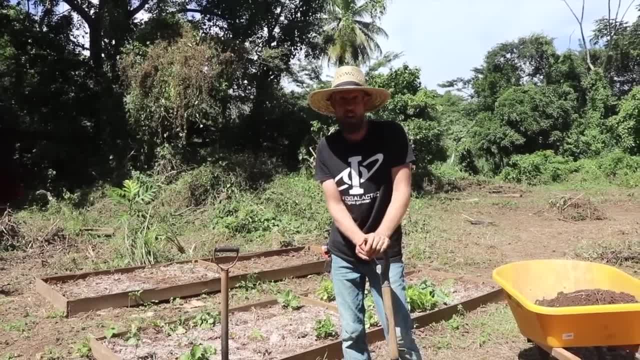 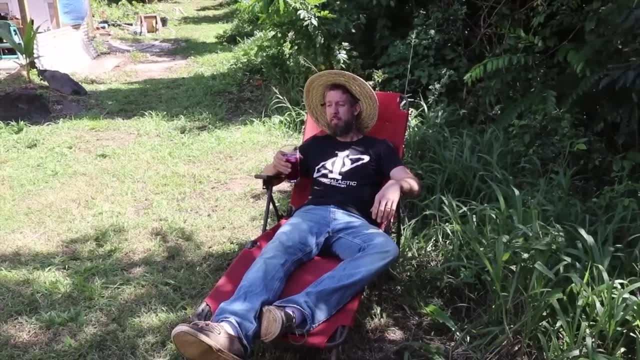 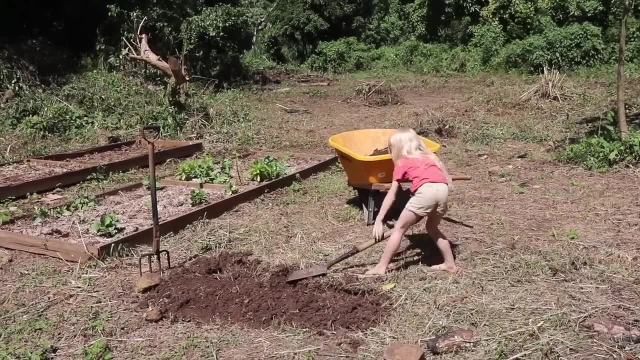 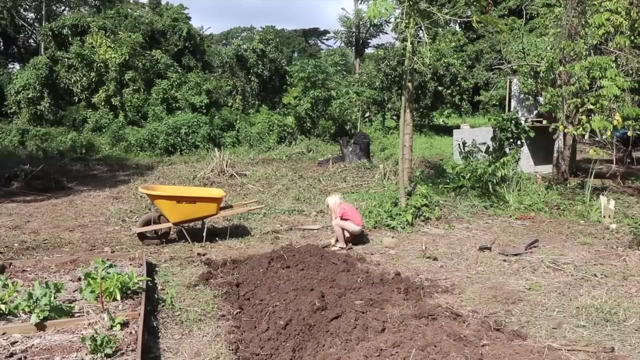 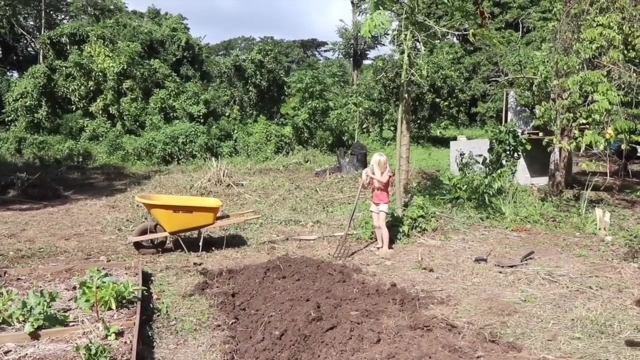 Fortunately there is a much easier way. Hey, you can do it, Come on, put your back in it, Come on. Yeah, you got it, You can do it, Come on, Come on. Oh, good job, Thank you. 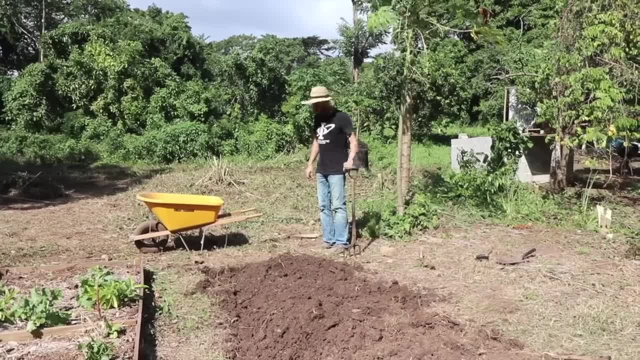 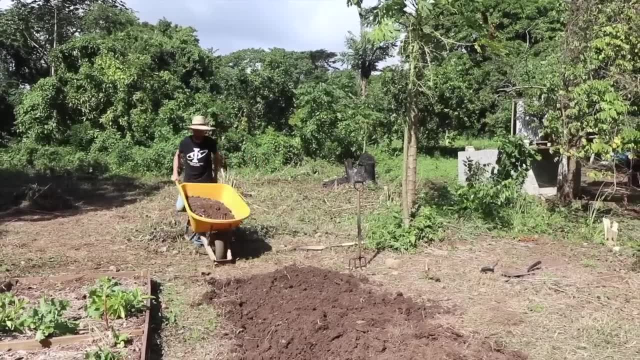 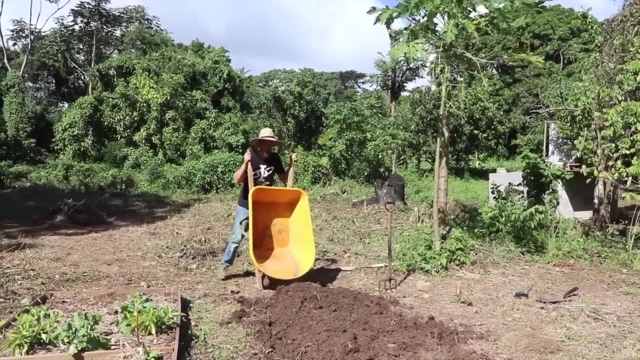 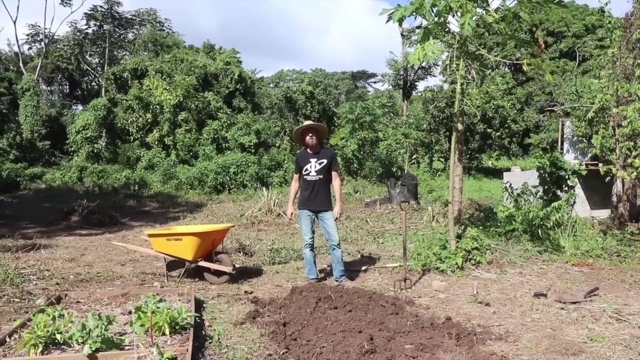 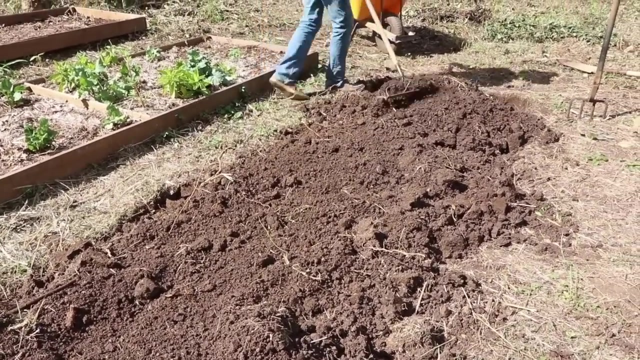 Go get some water. Now all we have to do dump this back into this trench- the dirt we took from the first bit, And we have Hey big mess of dirt. Let's make it look pretty. You're just gonna rake it nicely. You've got a good spot for your seeds and 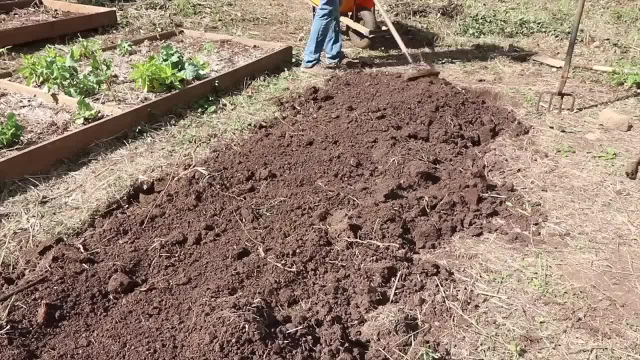 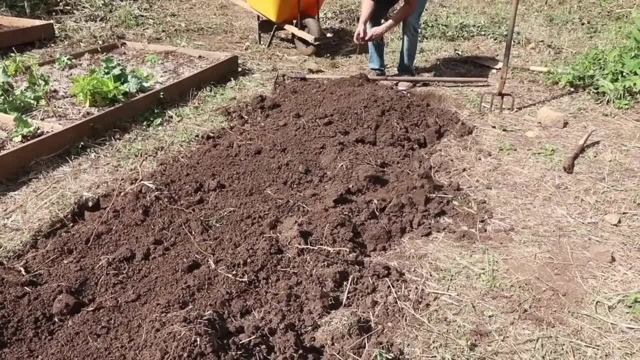 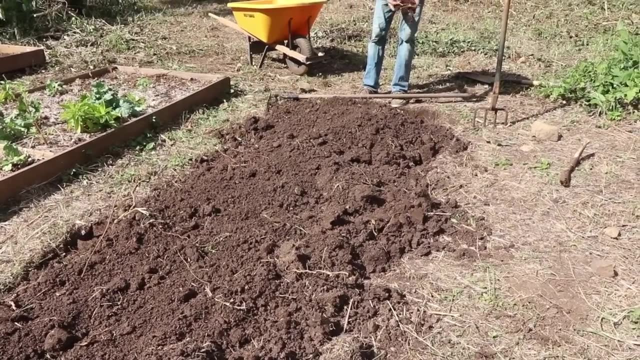 transplants and it doesn't just look like a big ugly mound of dirt. Now I know I said there was an easier way and then I put my daughter on it. I realized that a lot of you guys are probably watching from the United States or Canada or 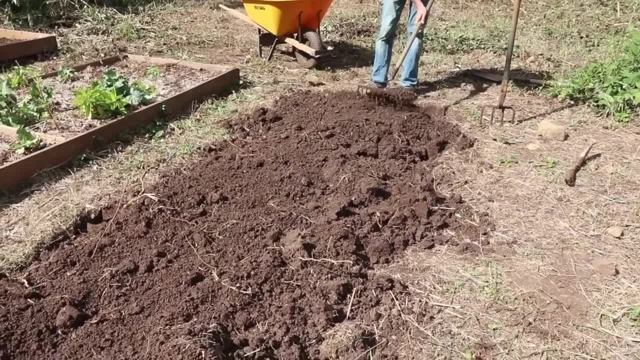 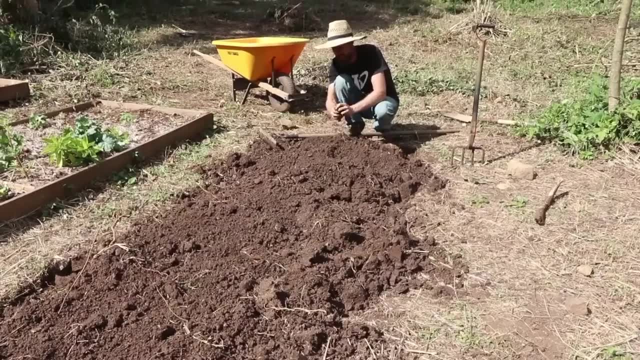 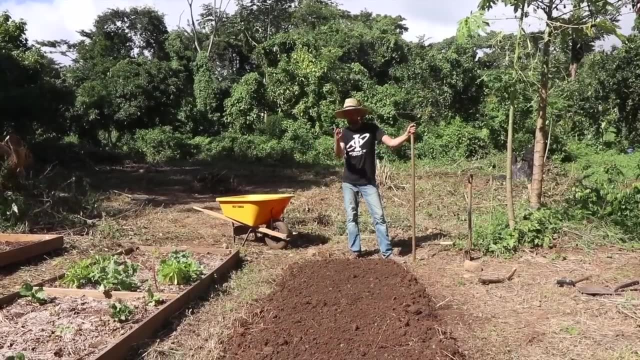 Australia or places with strict child labor laws. There actually is an easier way to build a bed than double digging. It doesn't necessarily give you the same incredible, deep, fluffy bed, And there we go. That is a nice, finished 4x12 double. 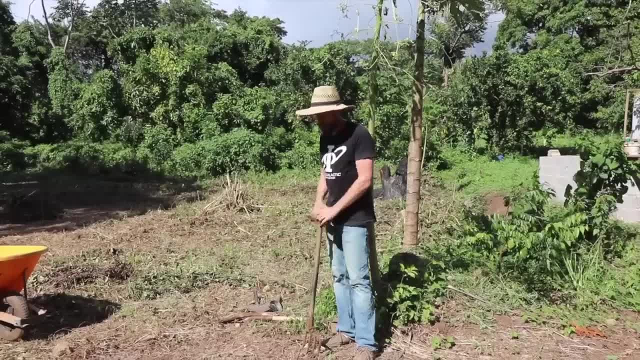 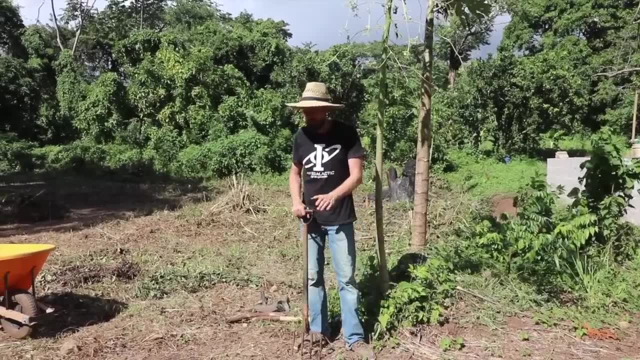 dug bed. Now I told you this was a good idea. There's an easier way. The easier way is to just take your spading fork. Okay, I want to start another bed right here. I'm gonna do another 4x12.. I am gonna do. 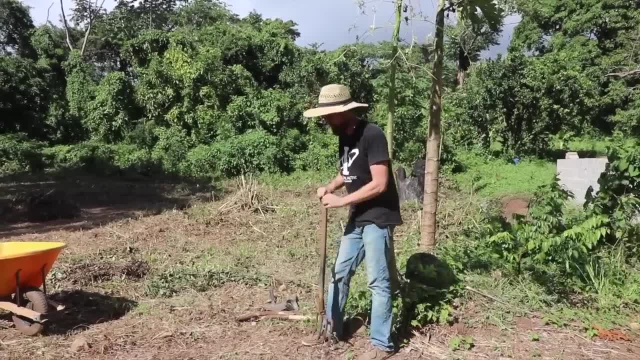 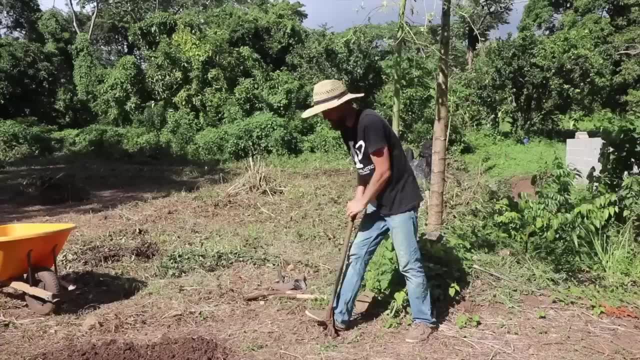 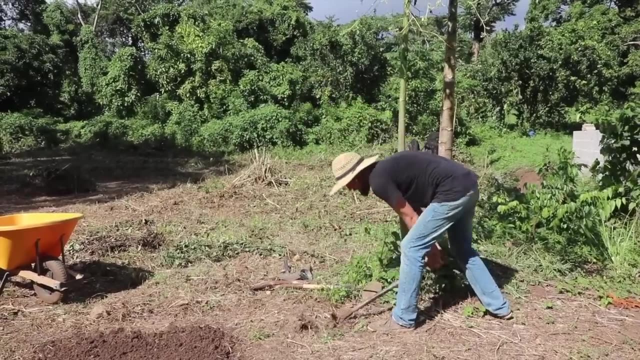 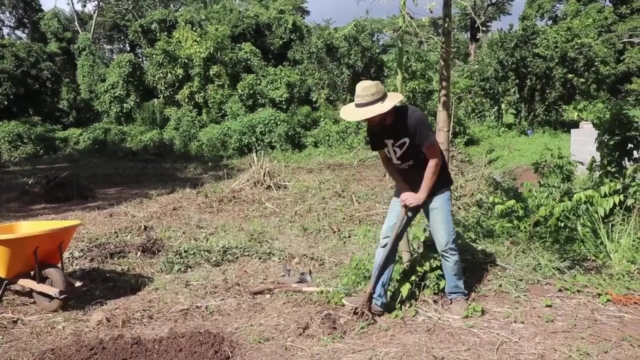 another 4x12, because all this ground behind me is gonna end up beds eventually. But I've got this fork and I'm just gonna go like this Loosen to the top of the fork. This fork is an old antique And I can just go like this And what I'm gonna do is just fork it up. Take out the. 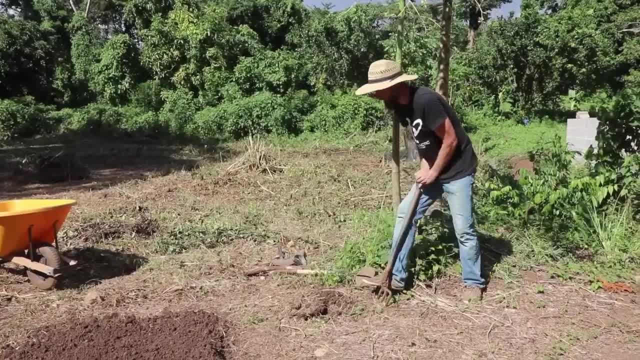 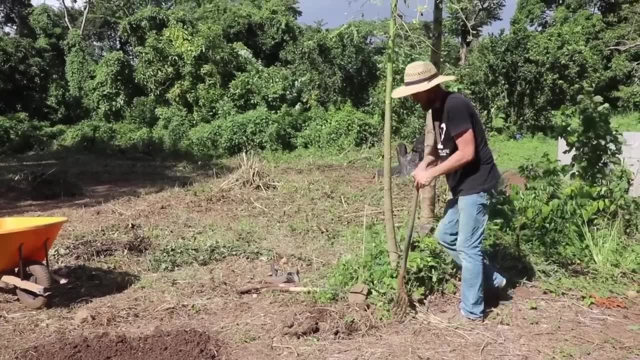 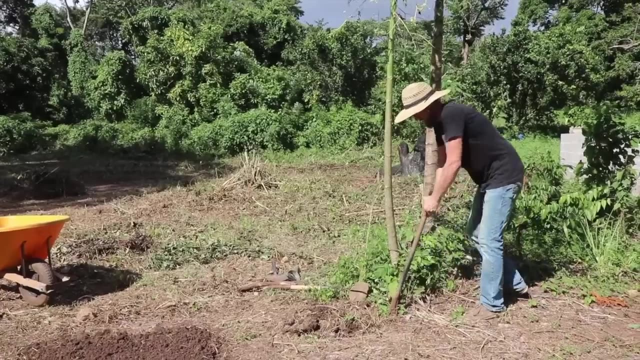 rock Your note. I'm not going nearly as deep because I was getting about 10 to 12 inches probably with the spade, Followed by maybe another 8 with this fork, Real deep. Now you may not have really compacted soil. You may have a back that does not agree with. 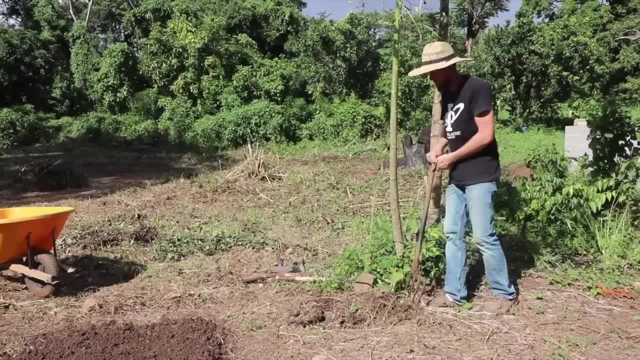 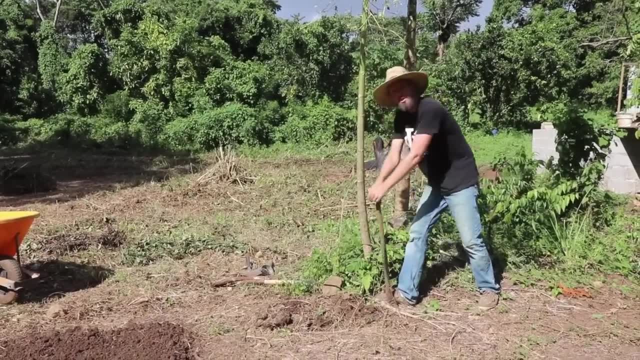 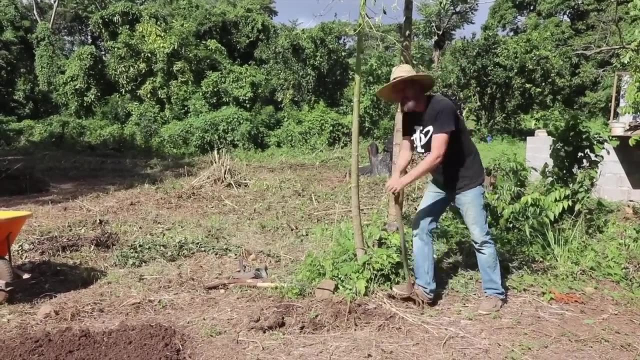 all that digging, You may say: well, you know what, I'll just take my fork and I'll do a bed like this. This gets you to about the depth of a regular tiller, Which is the other method that you can use if you want to go really fast and put in a garden. Borrow somebody's tiller. 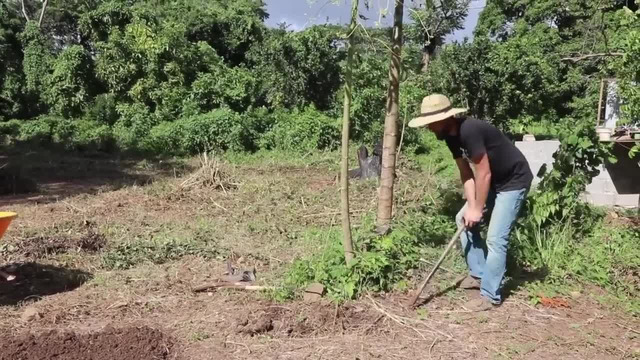 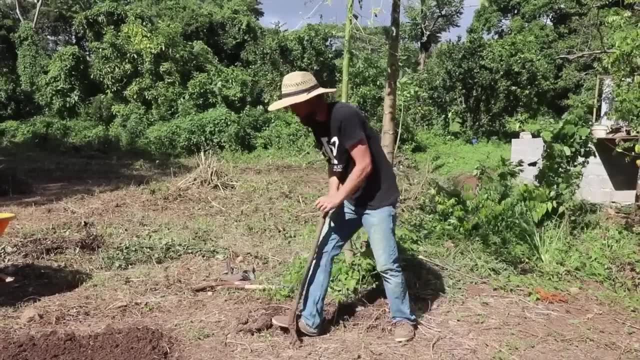 Go down to your local store. there You can often get it at a tool rental place- 40 bucks. you can go till up. you know an entire half acre of ground if you want to. The problem with the tiller Is that it doesn't go nearly as deep. 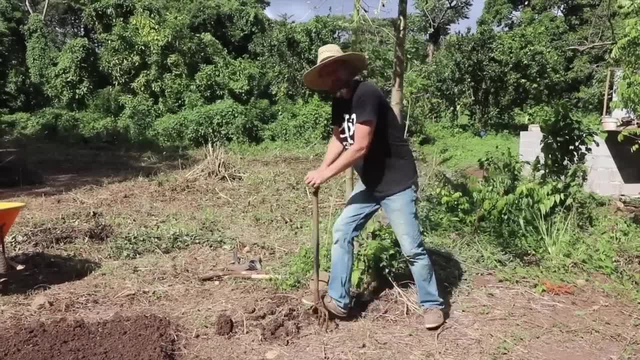 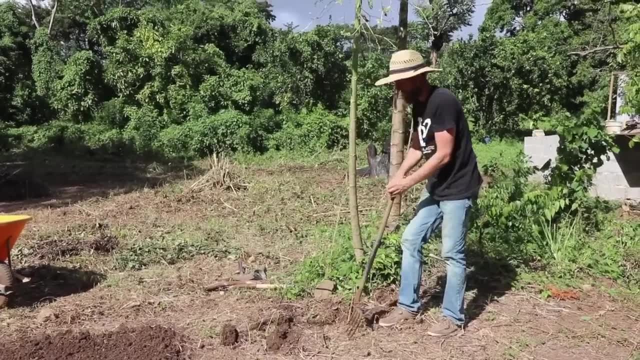 Shreds the ground And if you do it in the wrong time of year, Like if you've got real mucky soil or something, You do it- then you could really end up making a big mess of your yard. This is a little easier to control and, gentler. 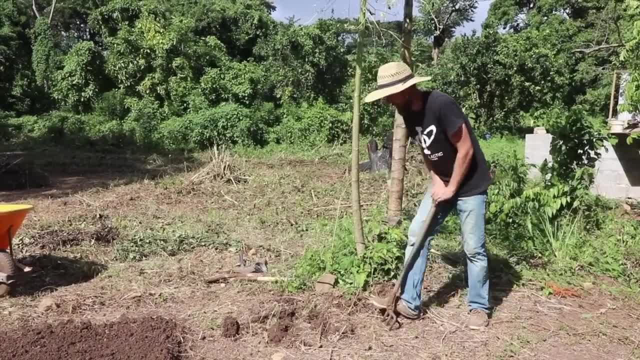 But it's really hard to beat what you get. How fast you get it with a tiller, Like it's just amazing. It feels like It's just so short, It's so heavy, It's all up to the tiller. It's just pretty heavy, It's just. 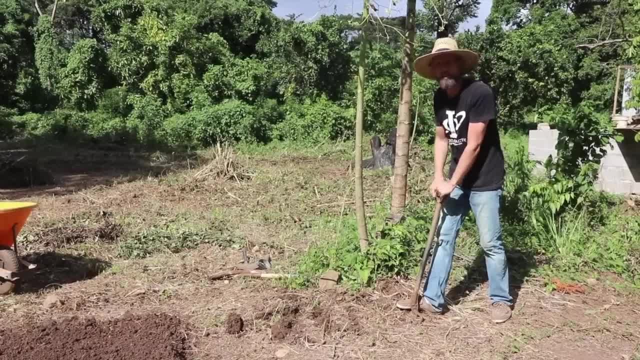 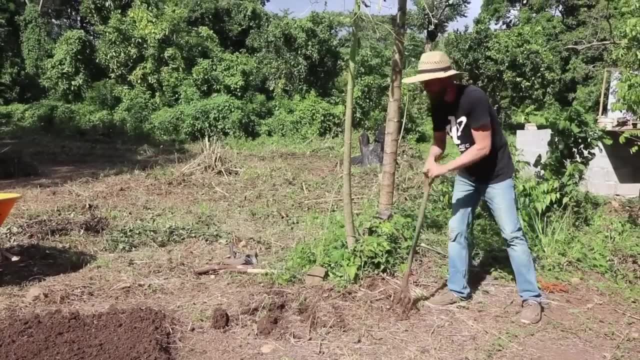 all up to the tiller. It feels like a rope. It feels like a rope, But it's hard to beat, holy moly. I mean, if I had a tiller right now, just tear this whole thing up, cut you know, run strings through the whole area and run beds- awesome, I do not fault. 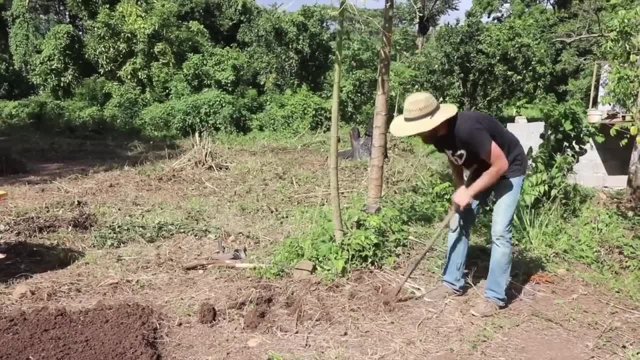 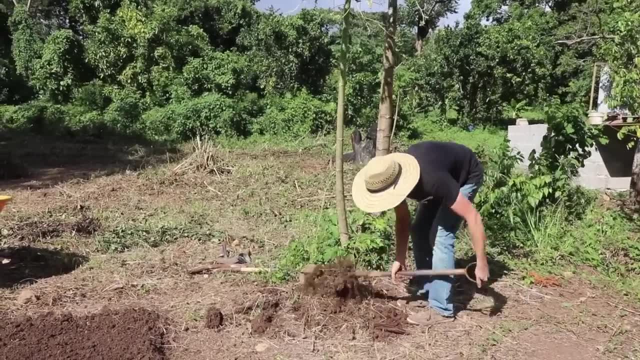 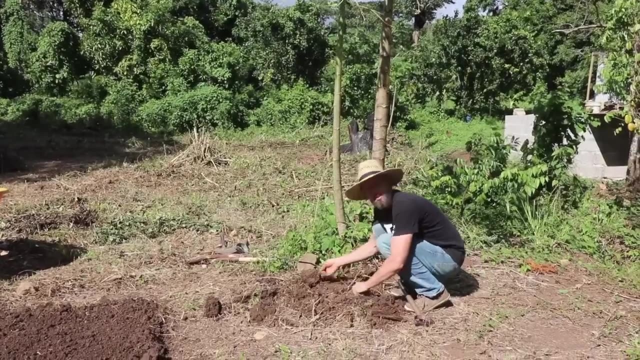 anybody for doing that, even though you may kill a few earthworms. so when I do this, I can just go back in like this and make a nice soft bed. I'm gonna do the same thing as much as possible: pick the rocks out, pick the perennial weeds out. yeah, we don't need all this, you know. 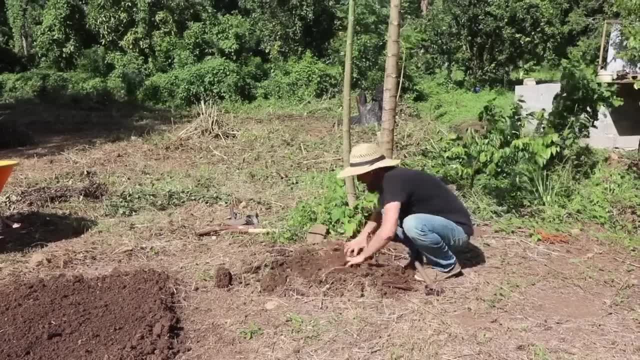 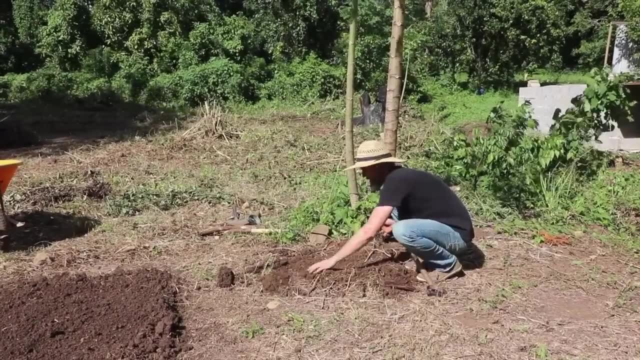 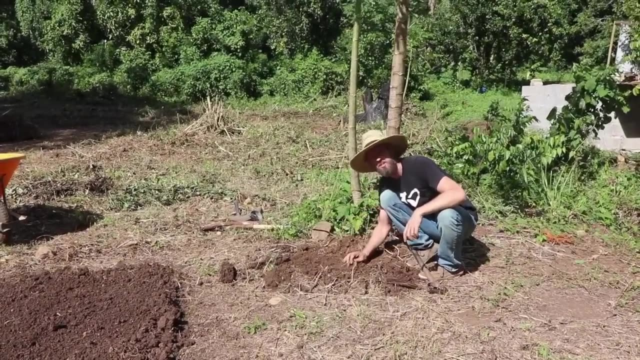 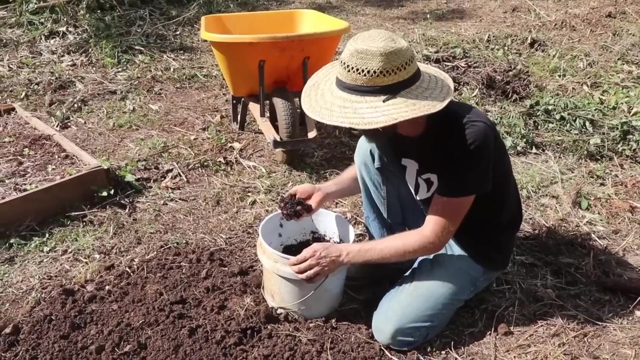 bust the clods. I could do the same thing that I did in the other one, just not quite so intense and not as deep. that's the easier way. those of you that don't really feel like doing all that digging or don't have a really strong daughter, I have here some beautiful 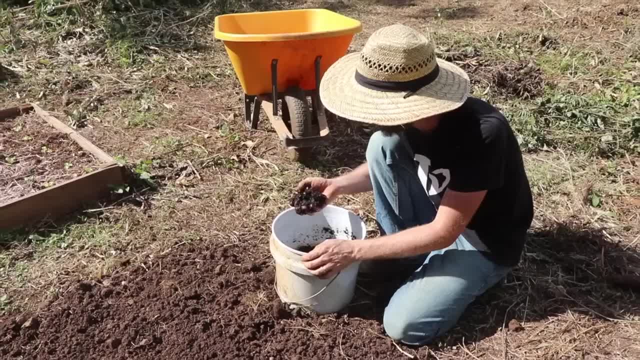 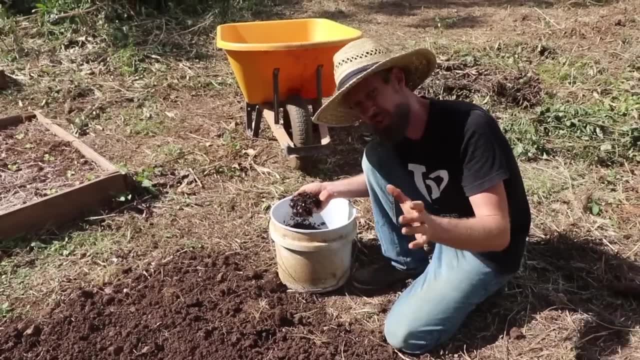 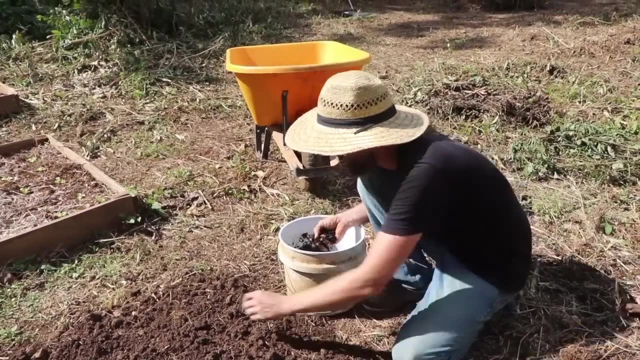 you compost still see a little bits of eggshells and stuff in it- perfect. and when I make a bed like this, we'll cover the rest of the fertilizing later, because you're gonna fertilize through the season too. but when I make a bed like this, I like to throw a little compost on it right at the beginning and 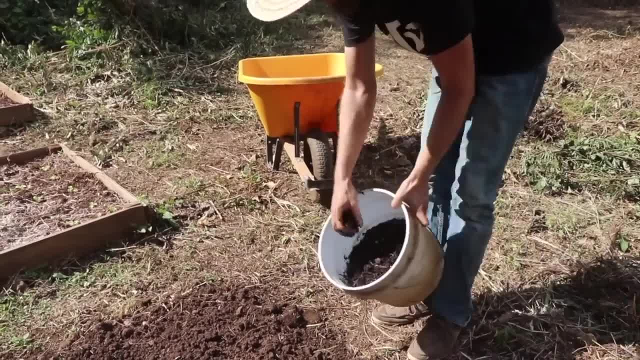 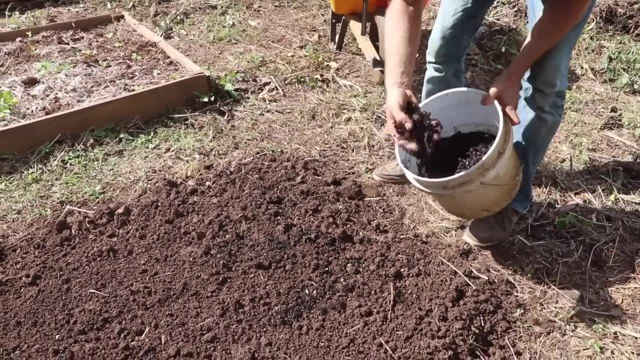 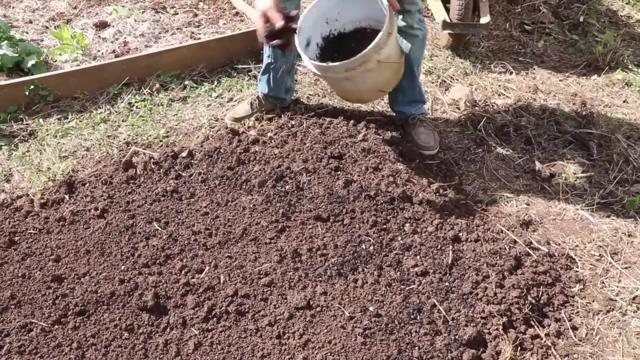 so this bit right here I'll just go across and go like: this doesn't need a ton. if you're not composting. I highly recommend you set up a little area, start composting all your kitchen scraps. when you mow the lawn, you go ahead and throw your grass. 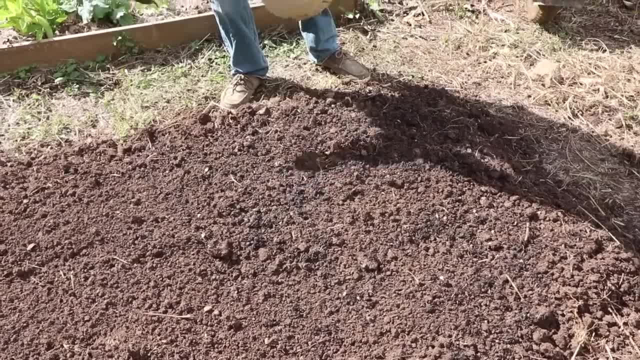 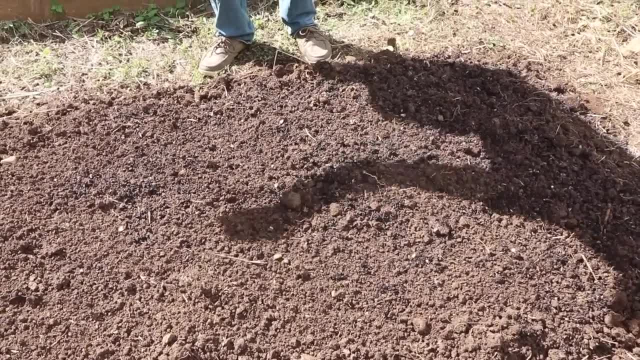 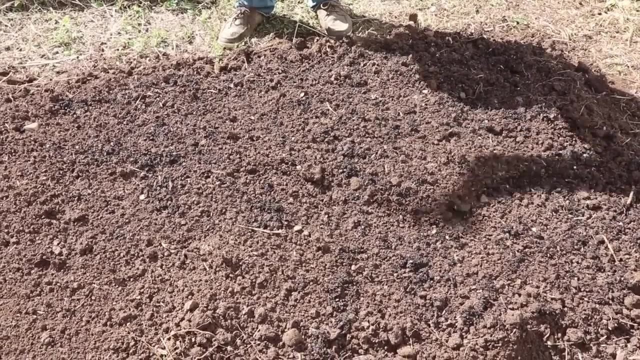 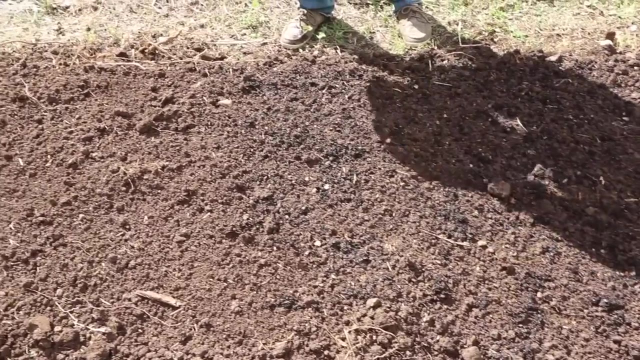 clippings in. you know you get serious. you take the shredded paper from the office. or you know, get all the paper plates from your next church picnic, throw chicken bones in there, it doesn't matter. I wrote the book: compost everything and I'm gonna show you how to compost- the good guide to extreme composting, and I 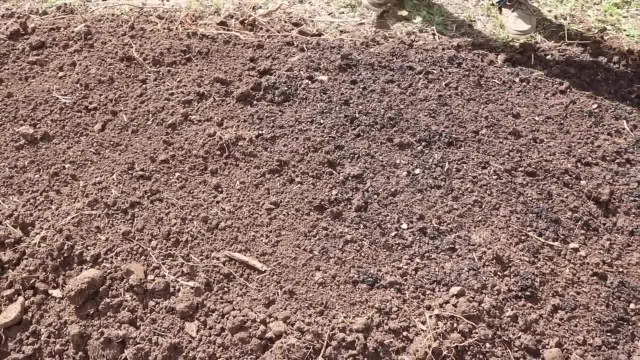 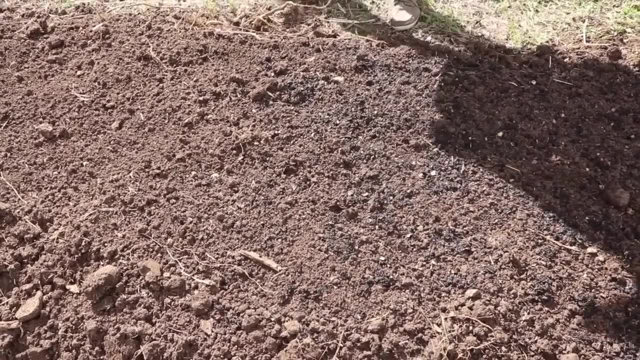 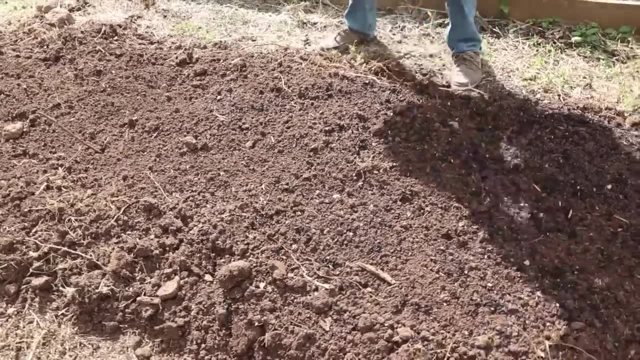 do compost just about everything. so long as you keep the rats out and keep the smell down, you could throw meat in there, you throw lasagna in there, throw a gallon of spoiled milk in there. all that stuff can be returned to the soil- much better than throwing in a landfill, don't you think? I think so. 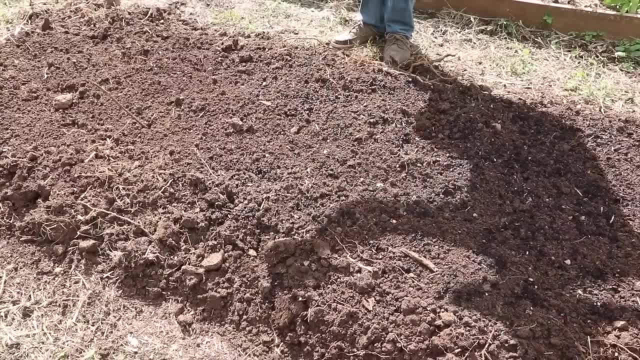 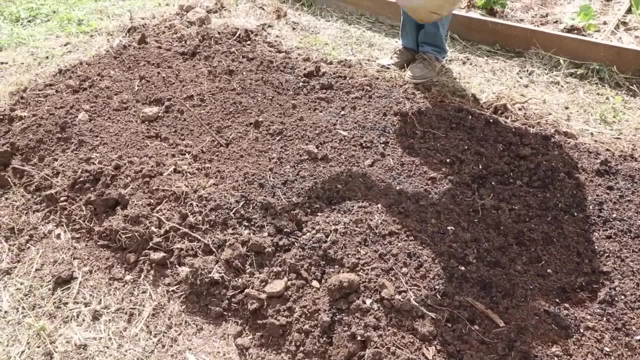 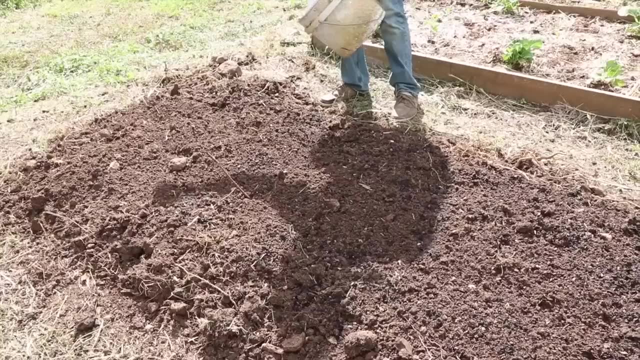 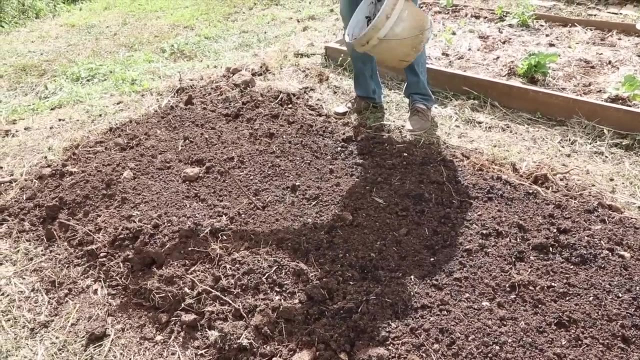 so you notice I'm not putting a ton of compost on here, I'm just gonna keep it on here. this is not an incredible amount of compost. you don't really need a whole ton, especially if it's new ground. you'll see some people using just massive amounts of compost. plants don't really need that much to be happy. I'm. 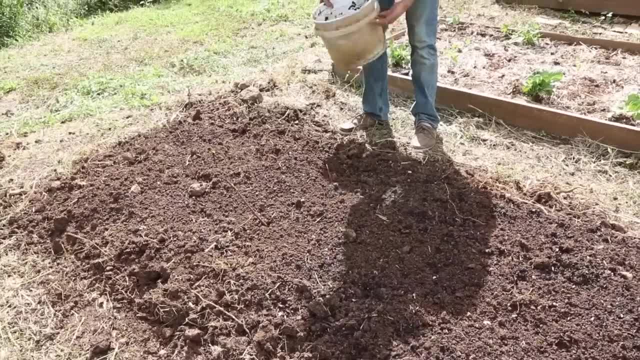 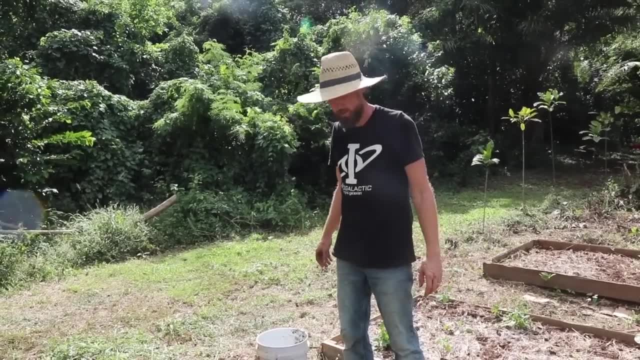 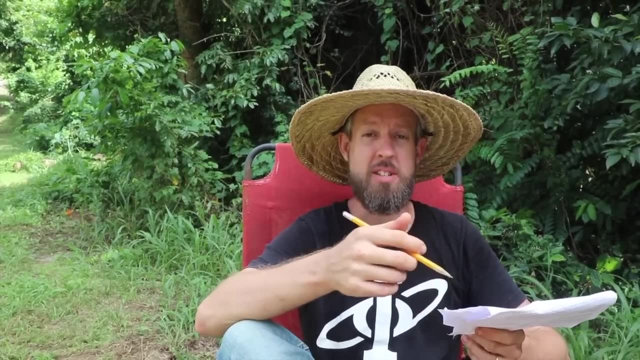 gonna run a little bit short here, but that's fine, that's good, we're ready to start transplanting. I'd say, before you actually go ahead and start transplanting or planting anything, or even buying seeds- I know it's really hard because you get to the middle of winter and you're like: I have a seed. 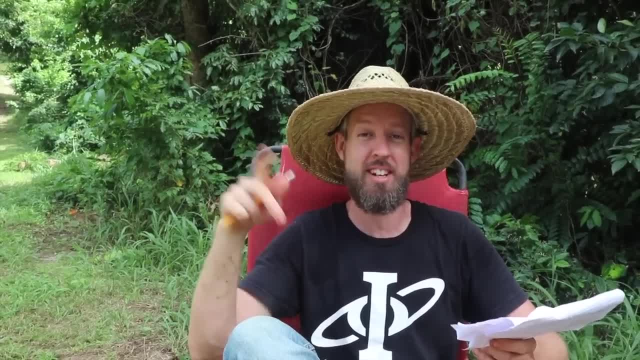 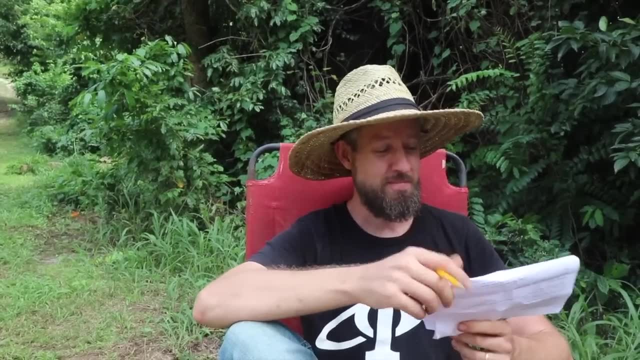 catalog. I want everything. I want the tomato. that's like a kaleidoscope. you know, you know before you get to that stage, if you can help yourself, you have to figure out why you're gardening. now I've went and I dug a bed. why am I even? 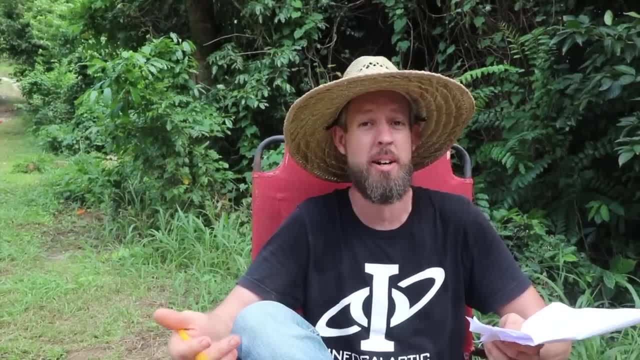 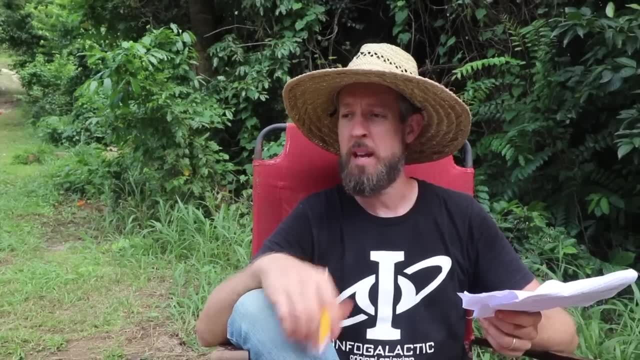 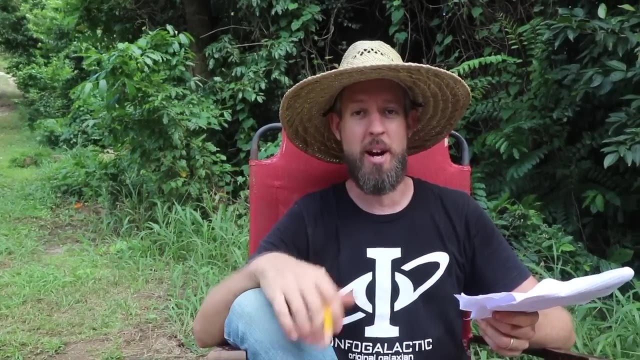 doing this? what was I thinking? why did I spend all that work? okay, do I think things are gonna get worse economically? am i a prepper? am i stacking ammo and gold and putting baked beans underneath my bed? well, in that case, I'm gardening for survival. right, I want food in hard times, so my focus should be for a garden like. 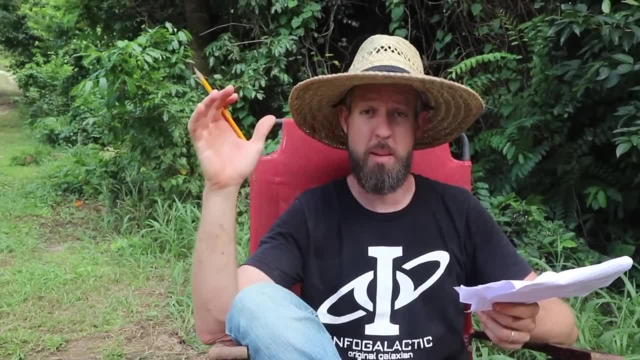 that on staple crops, right so? heavy-duty calories, we want to plant a lot of crops, right? so heavy-duty calories, we want to plant a lot of crops, right so we want to plant a lot of crops, right? so heavy-duty calories, we want to plant a lot of crops, right so heavy-duty calories, we want to plant a lot of. potatoes. if we're farther north, maybe you would plant some grain varieties of corn. you might plant Jerusalem artichokes, provided your intestinal tract can handle them. you might plant turnips. you know, you get a little further south, you get into the tropics, a little more tropical, you go for sweet. 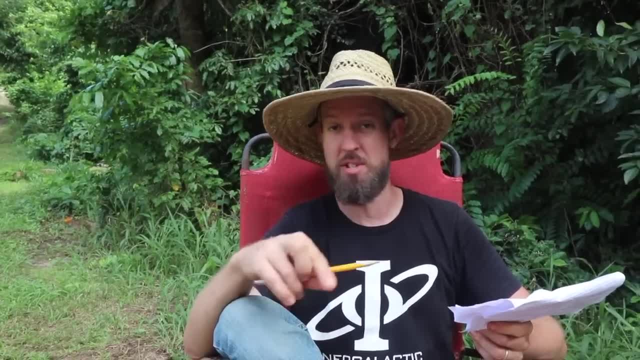 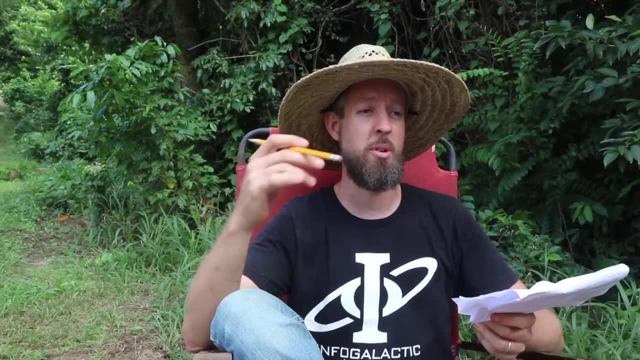 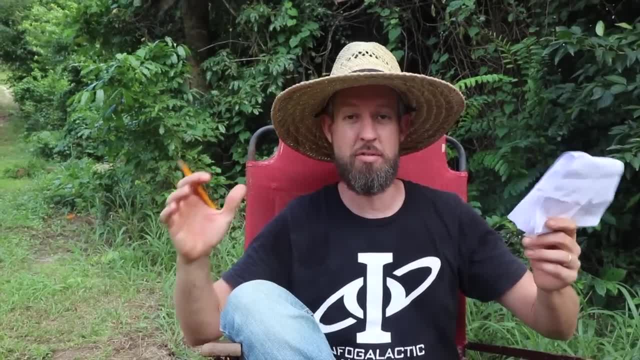 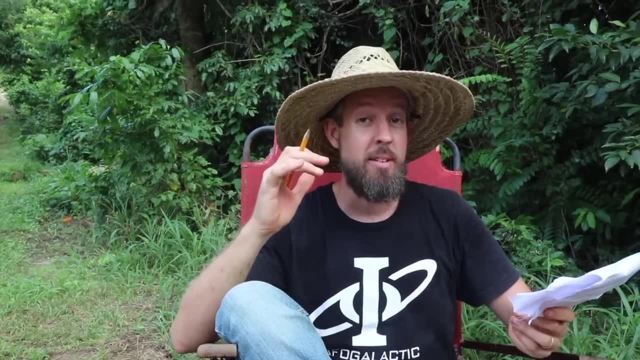 you could put in highly nutritious crops like cabbage and kale, so you're gonna have those around the edges. your main focus is on getting you through, feeding you, filling you up, and then, secondarily, you're going to go for medicinal. now maybe you're not in the survival gardening mode at all. maybe you want to live a. 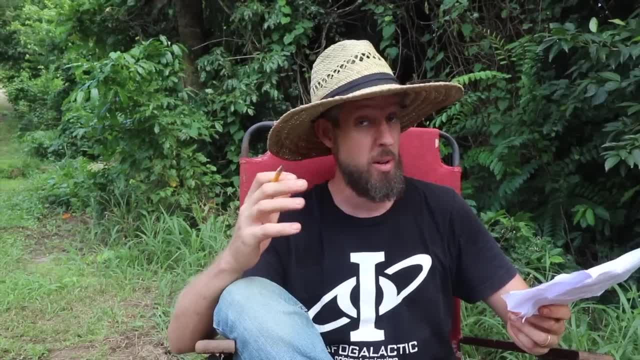 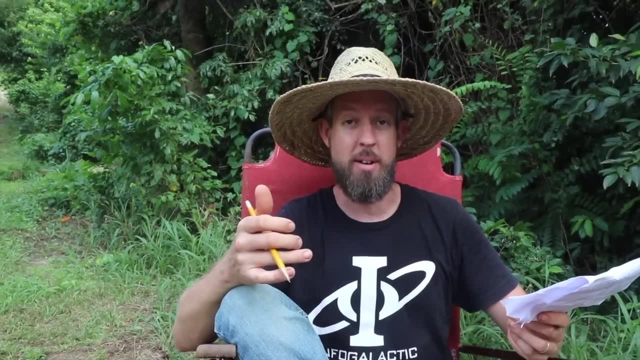 healthier lifestyle. maybe you love herbs. maybe you want to start distilling your own essential oils. well, in that case, let's take some of those things that rosemary and oregano. let's plant an herb garden so you go find the herbs that you like to grow and you plant a bunch of those. maybe you're. 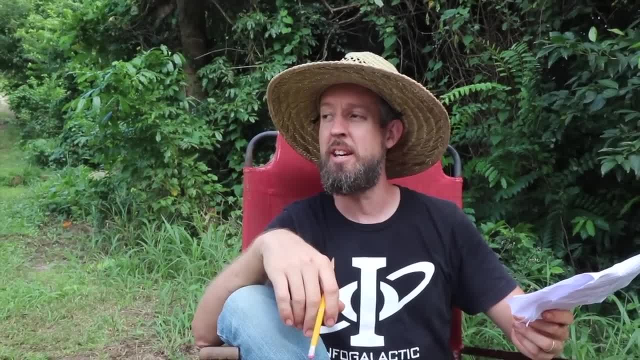 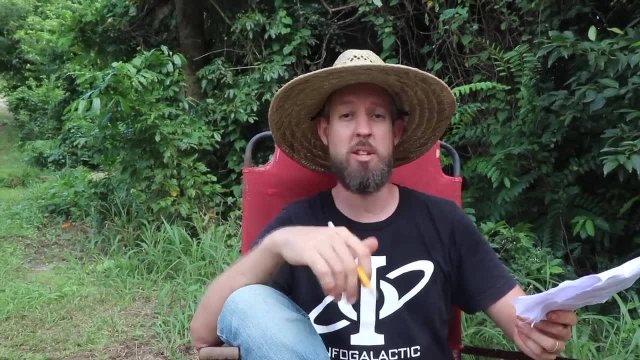 in a money saving mode. you're not a survivalist, necessarily. you're a mom. you've got kids that you want to feed and you have specific vegetables that you want to eat. the problem is, when you go to the store and you buy the vegetables, you don't know what they've been sprayed with. you don't know. 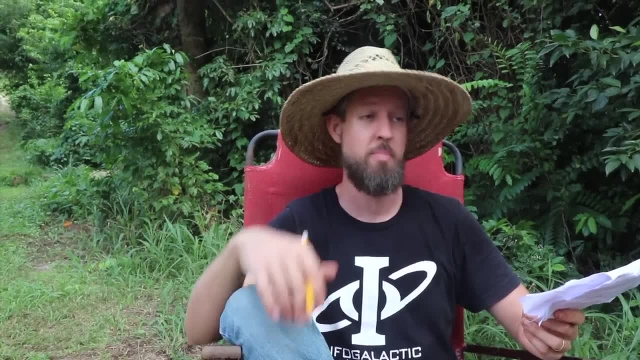 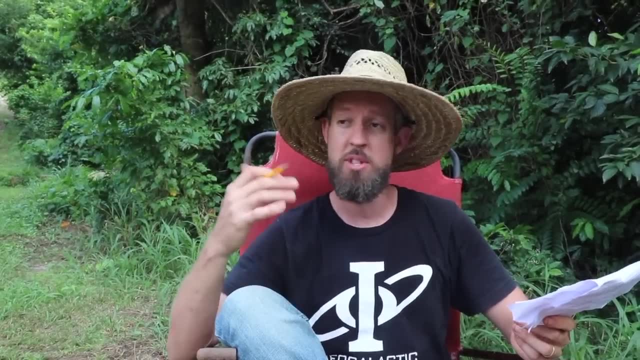 how they've been handled. you don't know if you're going to get e-coli or something horrible, you know. so you're like: i want to be healthy, i want my kids to eat good food, but if i go to the organic market totally breaks the bank, so i'm stuck buying bags of produce that i'm 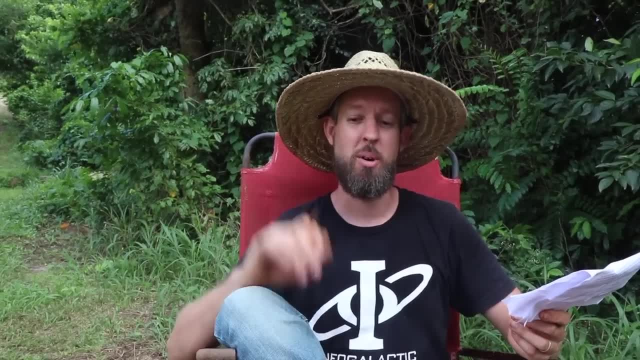 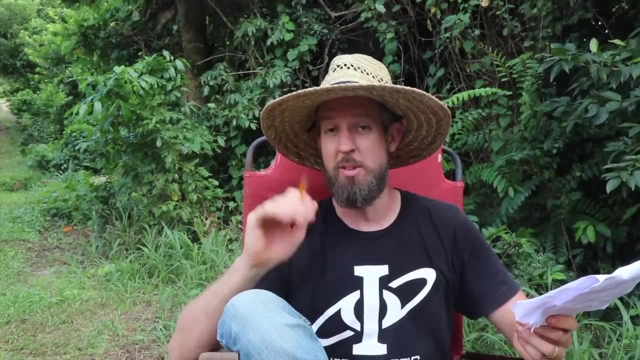 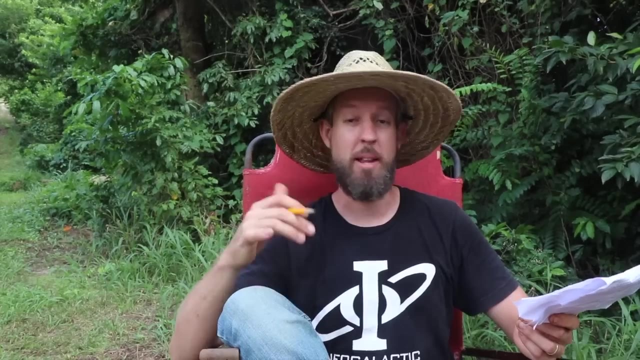 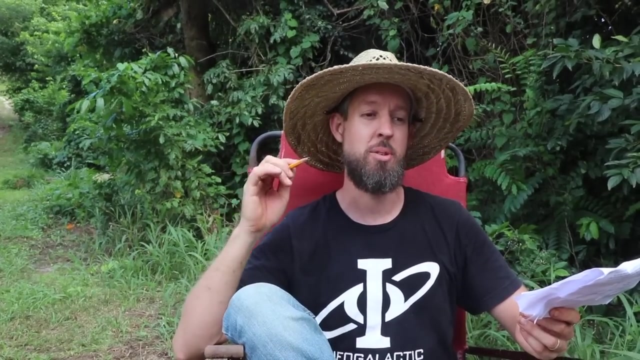 not you. So in that case, what are you going to do? you're going to look at your receipts. you probably already know in your head what, what you guys eat regularly. maybe you're going to plant some tomatoes, maybe you plant some fresh basil, maybe you plant carrots. you know what are you eating on a regular basis, that that you could get organically out of your garden in your backyard, knowing you're getting the highest quality and freshest produce. 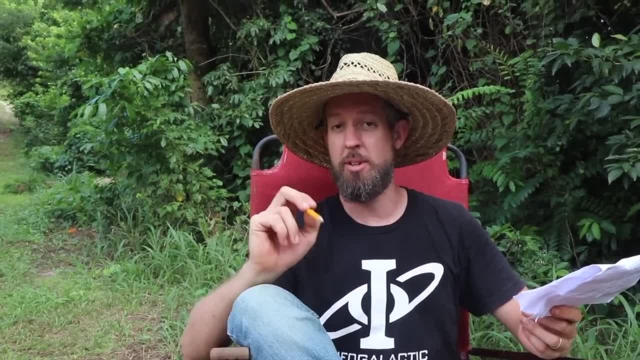 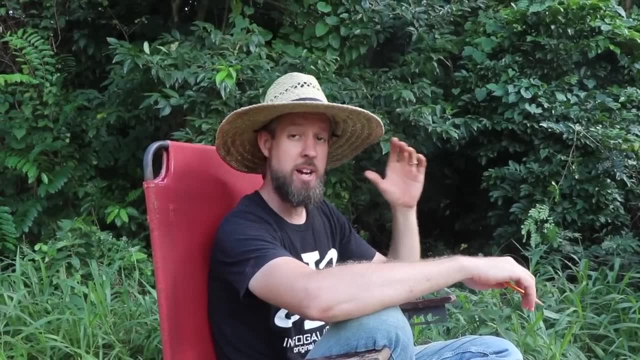 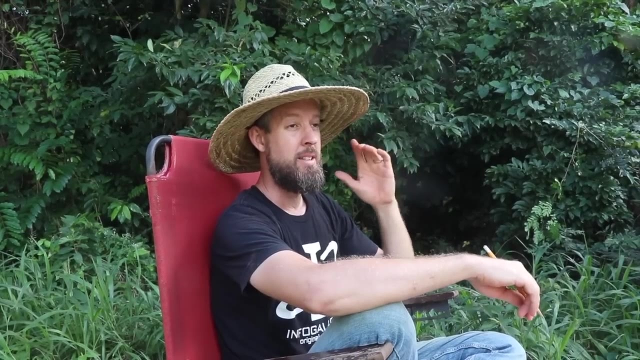 So you determine what you want to do in your garden first and then say, okay, this is my game plan, this is where I'm going to focus now. if you want success right off the bat, like this is your first garden, let's go for the simplest stuff. this is how I wrote the book: totally crazy easy. Florida gardeningens like. 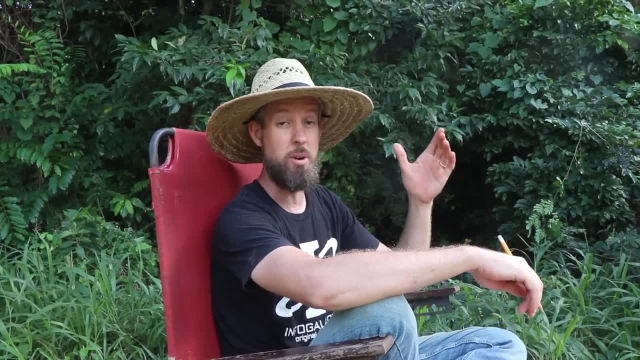 so far as i know. it seems like it's the best selling Florida gardening book on amazon, as best as i could tell on the rankings, and it's done very well, very popularly in the market and i've taken good atau back over to amazoncom. my 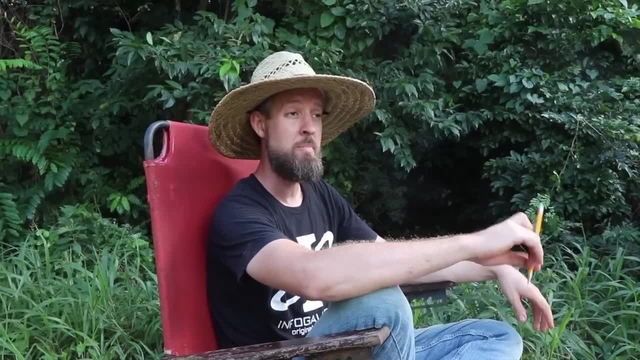 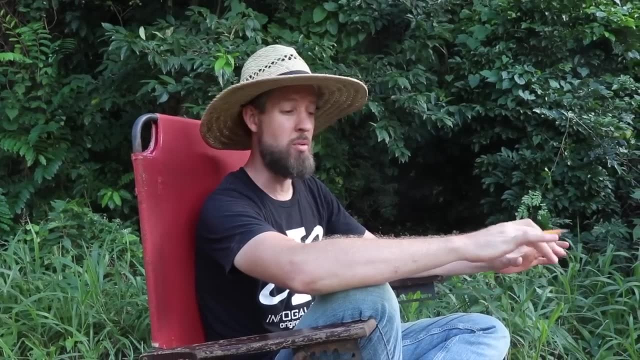 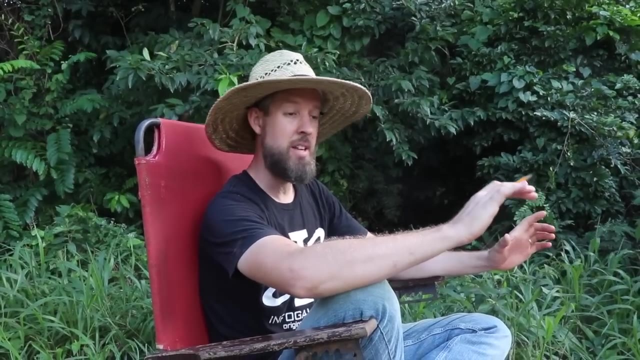 the rankings. You know it's done very well, very popular in the state of Florida, But in totally crazy easy Florida gardening, what I did was planted a wide variety of crops over multiple years And then the crops that were the easiest to grow, that did the best, that needed the least. 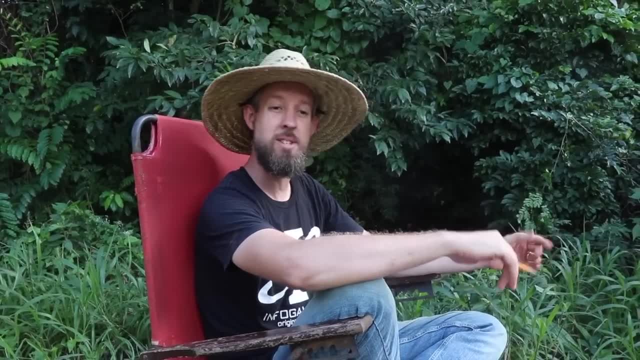 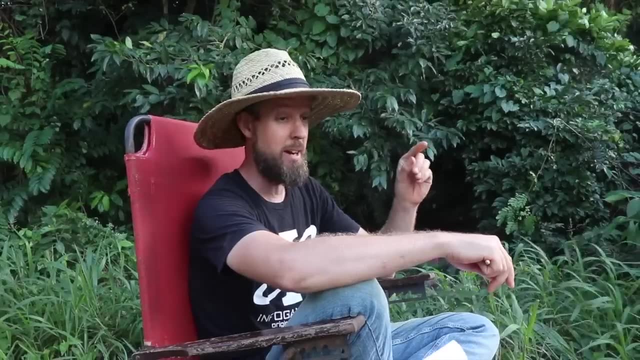 amount of work that stood, the heat and the weeds and the bugs and everything else. I planted them again and again, and again And I got an idea over time: okay, this thing will die, this one will live, this one dies, this one lives. And I planted, and I grew, and I planted and I grew, bed after bed. after bed until I had a really good idea how you could grow a very good garden in the state of Florida in my backyard, But your backyard is probably not in north central Florida, zone 8b slash 9a along a ridge. Okay, Everybody's backyard is going to be a little different, Even if you lived a city over. 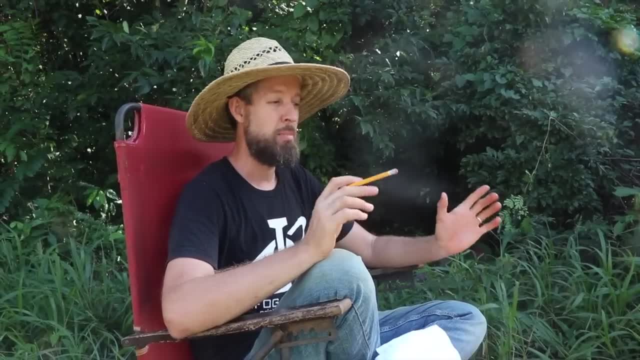 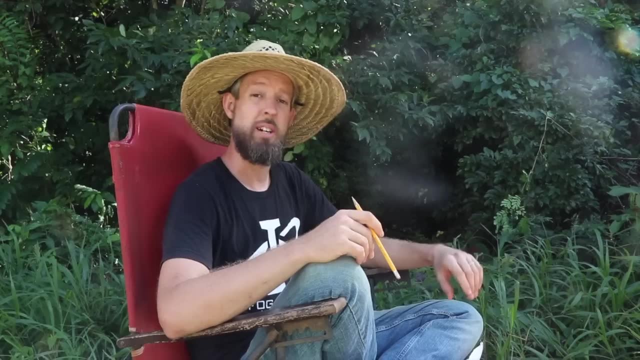 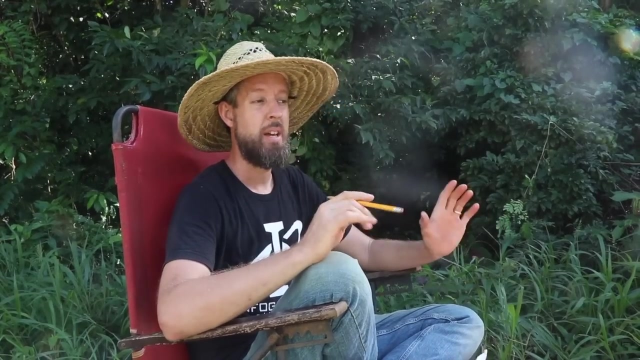 you might have a little bit different. a little bit different. My recommendations are going to work for the state of Florida, but they're probably not going to work the same for Georgia or California or New Zealand. There's a big change in climate And when we buy seeds- 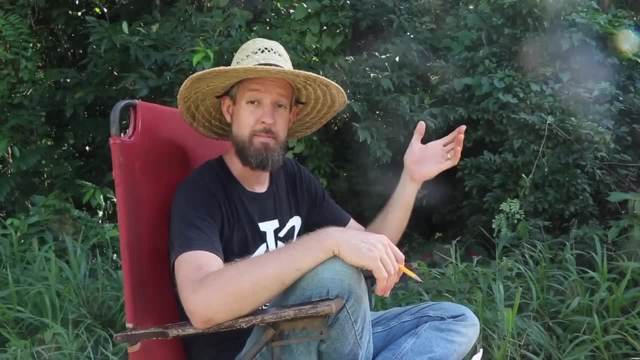 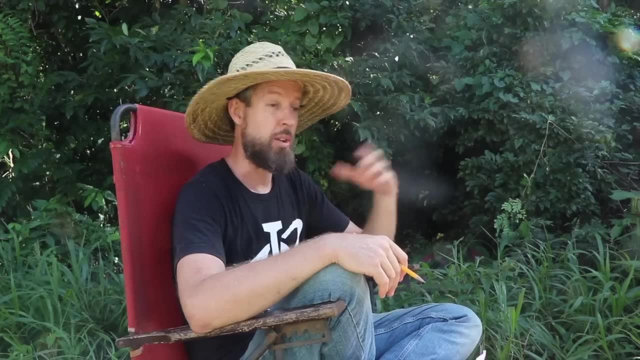 you might be buying seeds that are coming from New England or Brisbane. You know if they're grown in that climate, they're going to be growing in that climate And you take them and you grow them in Arizona or Costa Rica, you're going to get different results. than how they originally grew in New England or Brisbane right. So when you put them in your garden, you are putting them in a completely different environment than the one they were necessarily adapted to, unless you find a really local seed company and plant from them. There's. 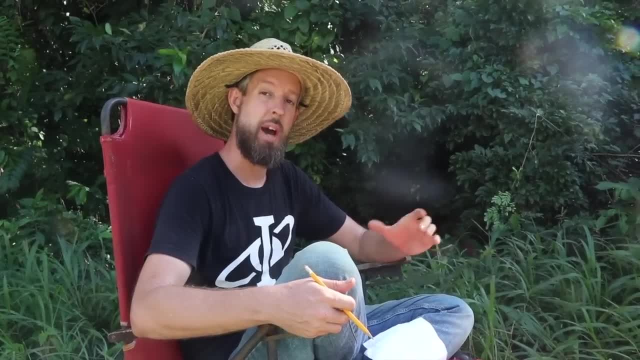 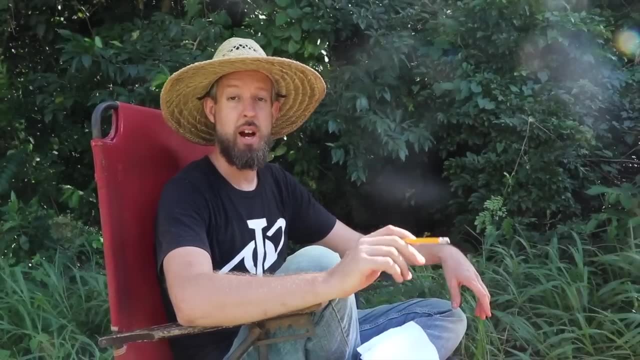 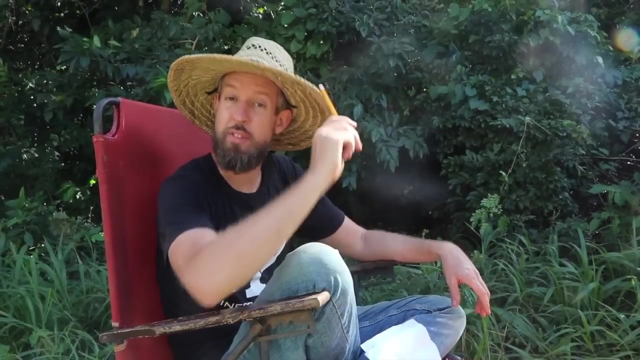 different environments and different plants do better under different things. We know that plants adapt to where they are, So you have some options to figure out what the easiest crops are for your garden. Option number one is to take the scientific method. The scientific method is to just go. 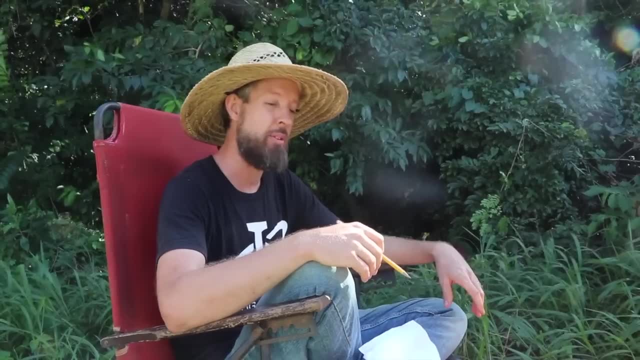 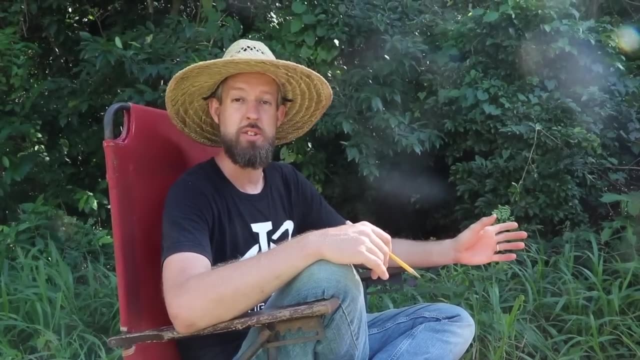 and get all different varieties of seeds and plants from wherever, anything that strikes your fancy, anything you're interested in. You plant your garden beds The first year you're going to have failures- all kinds of failures. We always have failures, but you might have a bunch of 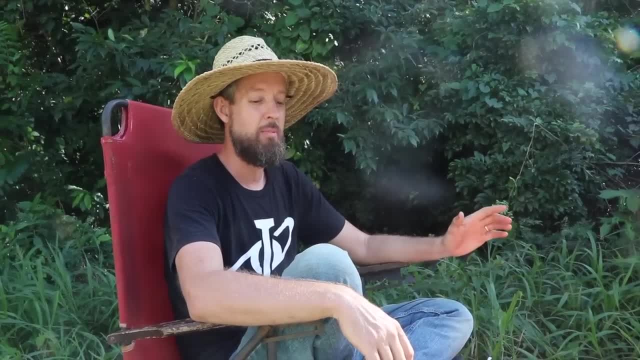 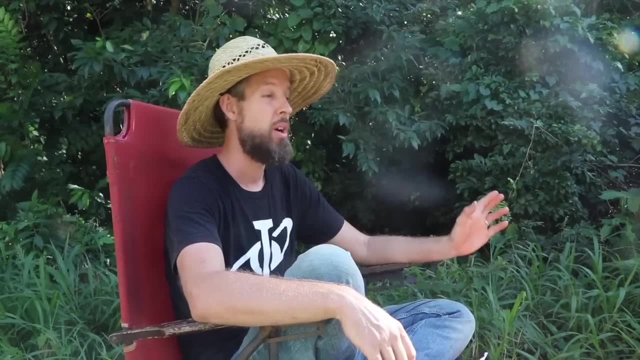 failures because you're just trying everything, The ones that fail, you say, okay, well, that one didn't do very well, Well, it might be a bad year, I really want to try it again. So you try it again the next year, if you want to, or you just discard it. 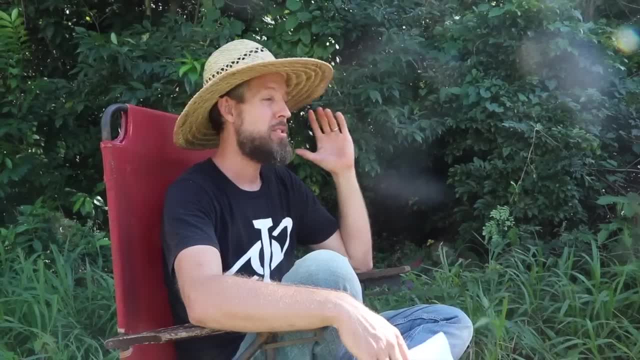 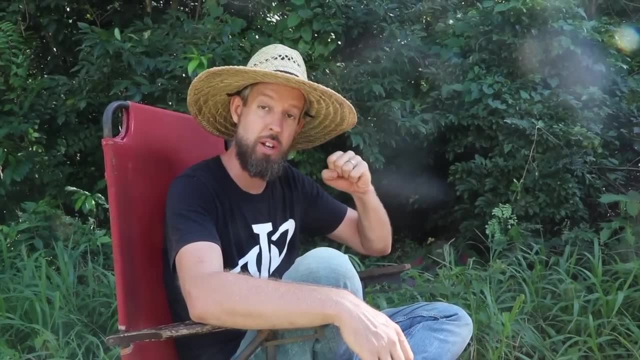 right off the bat: Quick death, sudden death, right. So such and such type of bean did not grow well for me, I'm done with it. And you plant another type of bean That one does well the next year, Okay, hold on to it. So what you do is you hold on to the ones that grow well And if you can save, seeds. that's even better because they'll start to adapt to your environment. the best and healthiest plants You save seeds from, those They'll adapt to your climate. After a few generations you'll have a variety that does much better than they would right from the seed packet. 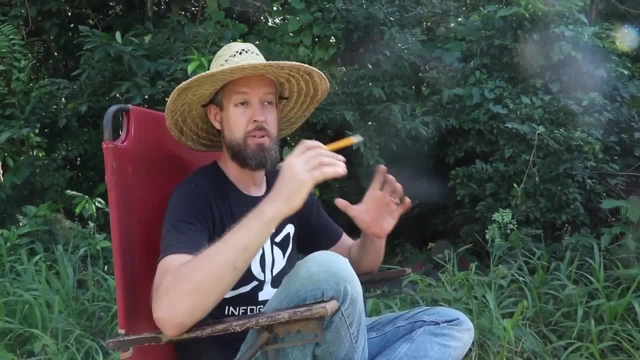 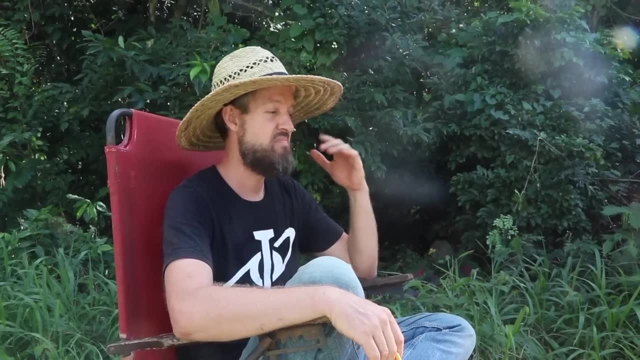 So what you're going to do is just plant a bunch of stuff that you're interested in, select out the ones that do really well, plant them again the next year. So you're doing the scientific method. You're not necessarily making control groups and all that kind of stuff. 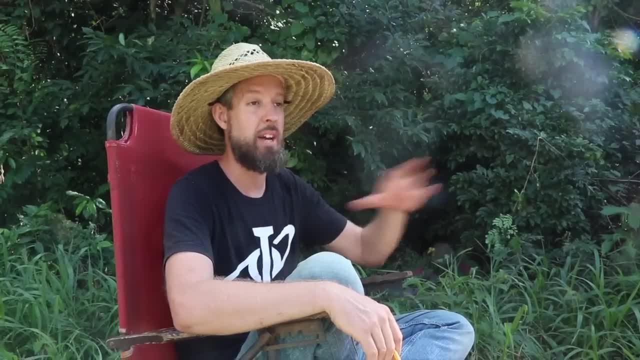 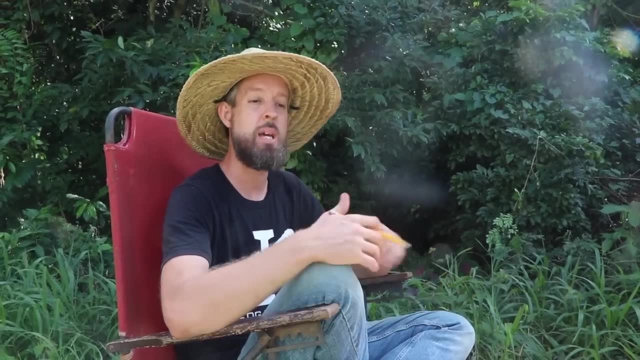 though you can. if you have that kind of mind, You can just plant a whole ton of stuff and just see what survives. Whatever survives, plant it again, Because it's better adapted to your climate. Keep trying new things. Don't just buy one variety of. 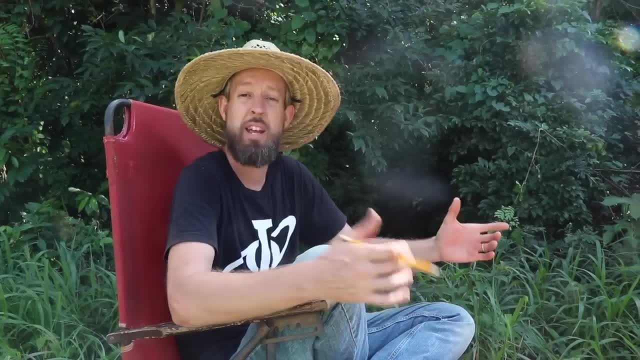 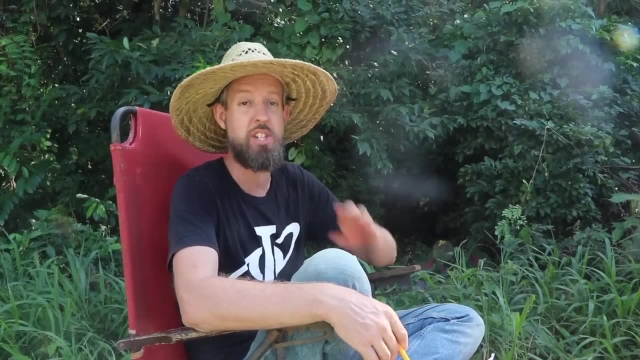 tomatoes and then say, oh, tomatoes don't grow here when they do poorly. No, buy like five different types. One of those varieties might do really well. You could chuck the other four and then get four more different varieties the next year and add them to that one And you can kind of figure out. 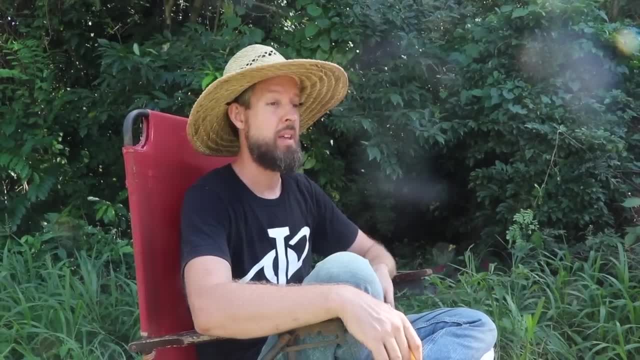 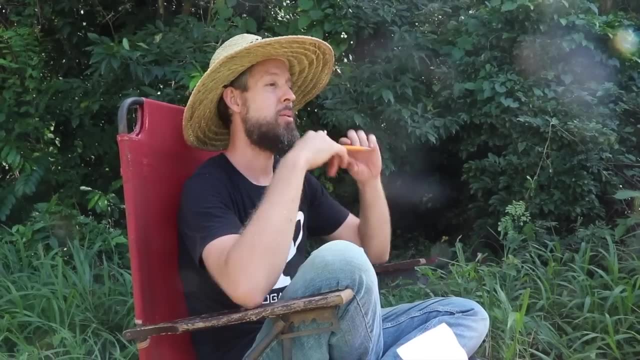 which tomatoes do well. Now, that's the scientific way to do it. That takes longer. The way you can really make it easy is to do the phone a friend method. Join a gardening group, Or you're walking around your neighborhood and you see an old lady out there. 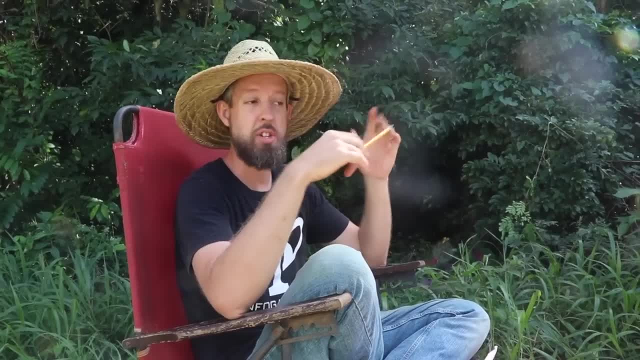 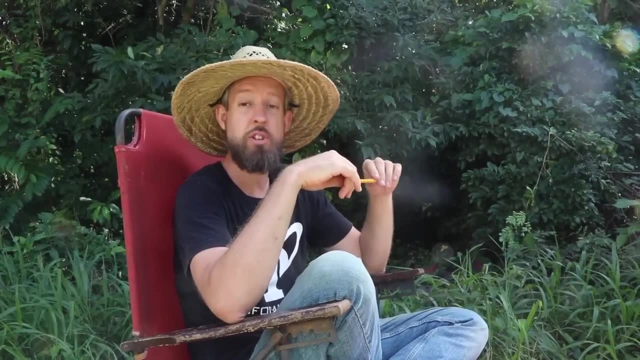 gardening And you say, hey, what are you growing? And she tells you what you're growing. How long have you been growing that? Well, I've been growing it for 20 years, So it obviously does. well, May I have some seeds? Or where did you get the seeds Right? So you find out what somebody has? 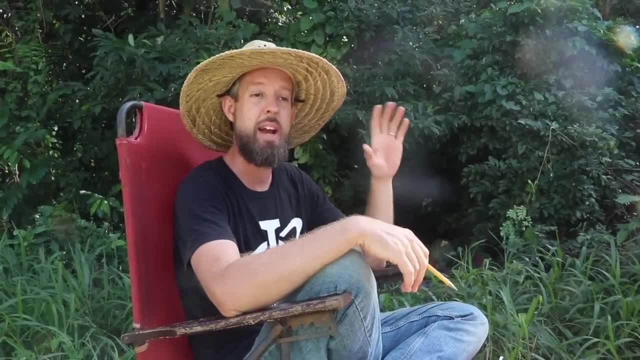 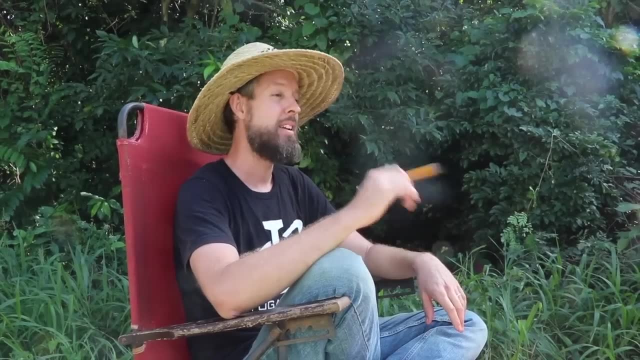 already done the scientific method on. They've been growing such and such tomato. Amish paste tomato has been doing really well, four blocks from you. Okay, plant that. Another thing you can do: okay, you make friends with gardeners. You could join a local gardening meet-up group. 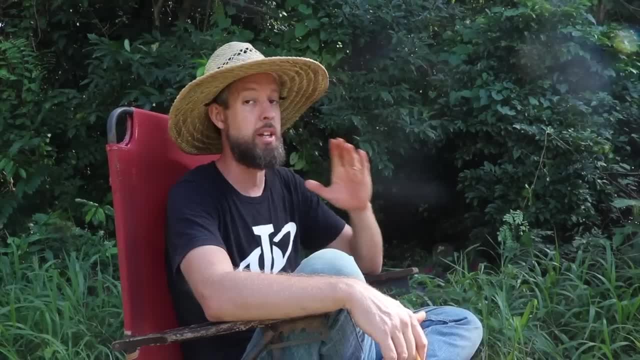 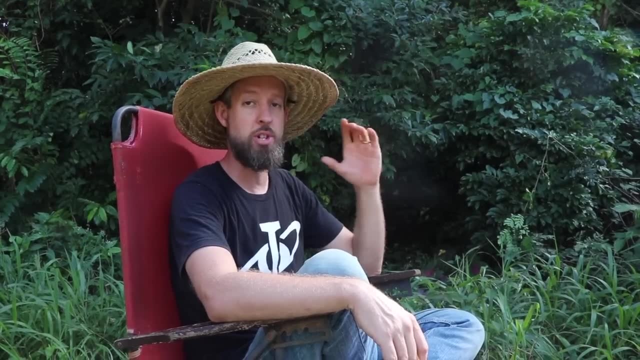 You know, pick their brains. What grows really easy for you, What grows really quickly, You'll figure it out. Another thing you can do is rely on the power of capitalism. right, If it's being grown commercially in your area, chances are it grows really well in your area because businessmen, farmers over time. 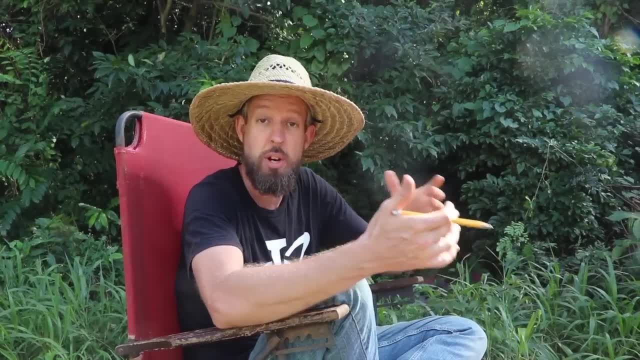 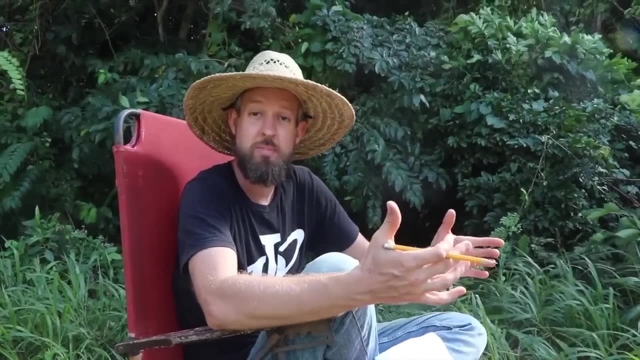 have determined. okay, this is a really good area. What do we think of when we think of Georgia? right, Jimmy Carter? We think of, uh, Peanuts, You think of pecans, You think of peaches. Those all grow really well there, So probably plant some of those. Now, if you go into your local farmer's market, you see all this produce. and where do you grow? Well, I grow right up the road there in Fort McCoy. Wow, Fort McCoy, okay, that's like 25 miles from me. 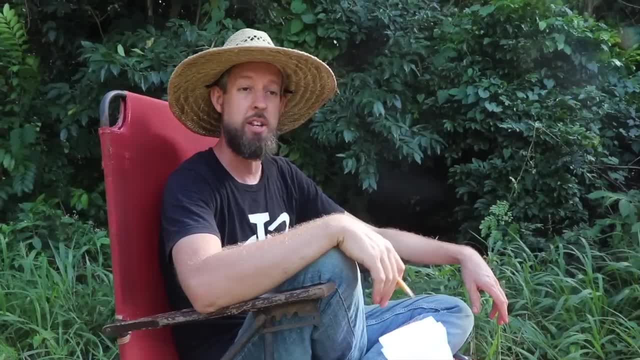 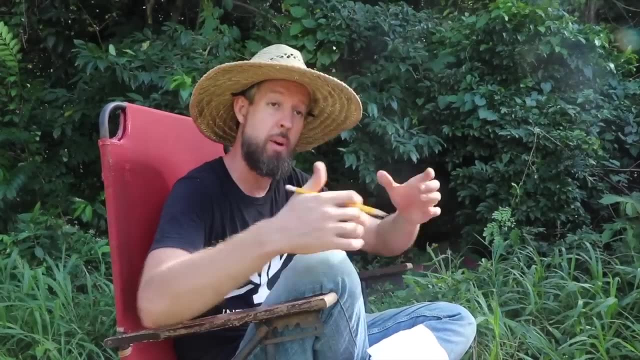 Uh, what are you growing? Oh, I grew this and this and this. How do they do for you? Are they easy? Oh yeah, super easy, No problem. Okay, grow that. Growing for the market and selling it. It may not be as wild and crazy as you want to try. 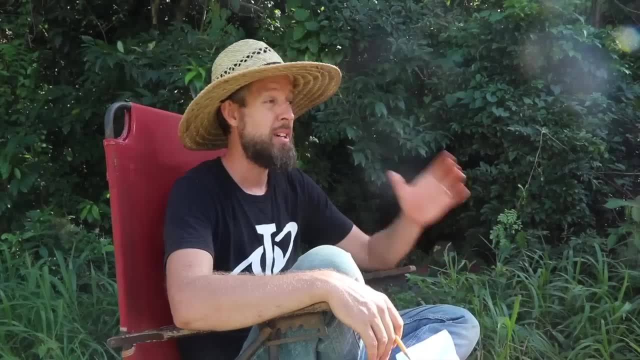 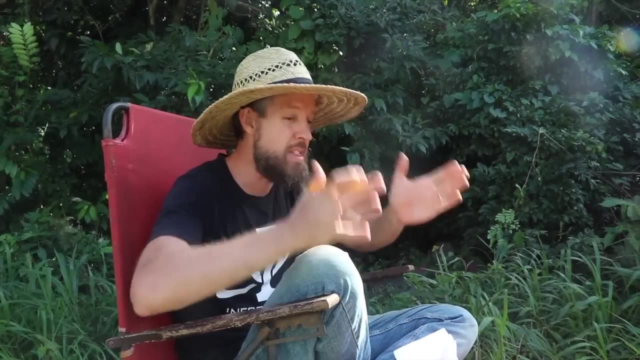 It may not be those kaleidoscope tomatoes, but you know, it might be something that just really is going to do well. It's almost certainly going to do well, And so you've got these, these things that are really suited to your area. 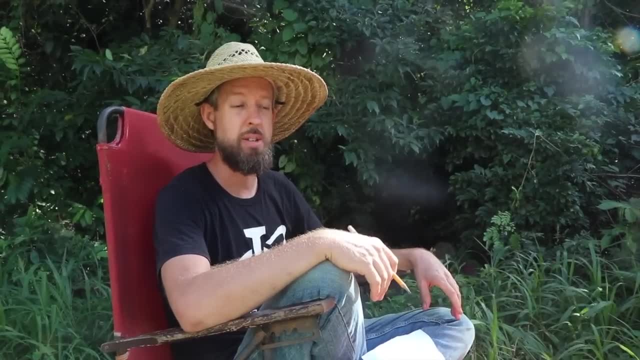 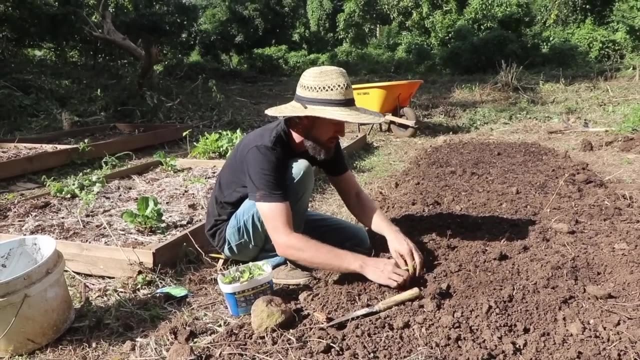 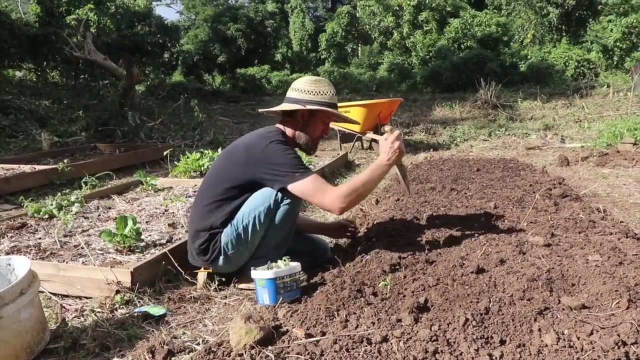 and you're just going to roll with them because that's the way to do it, the easy way, and we're all about doing it the easy way. I know what I want to grow. I want to grow everything in the entire world, so it's very easy for me to plant a garden bed. 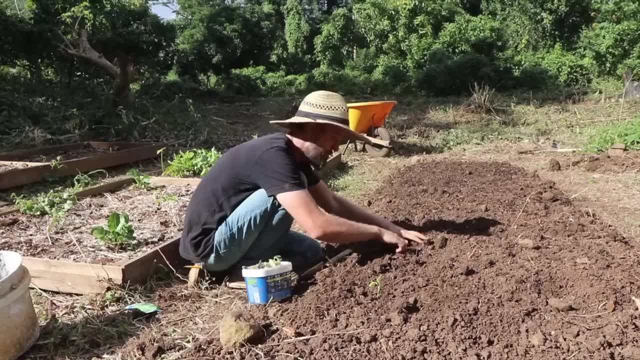 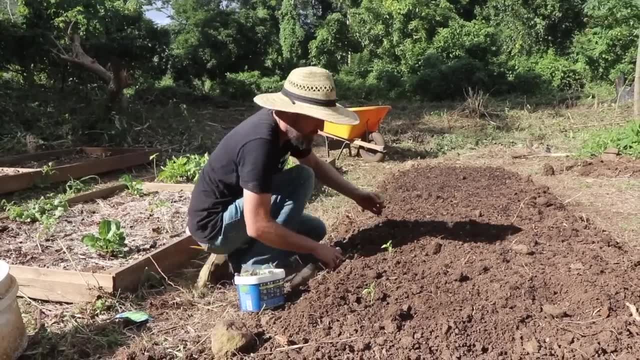 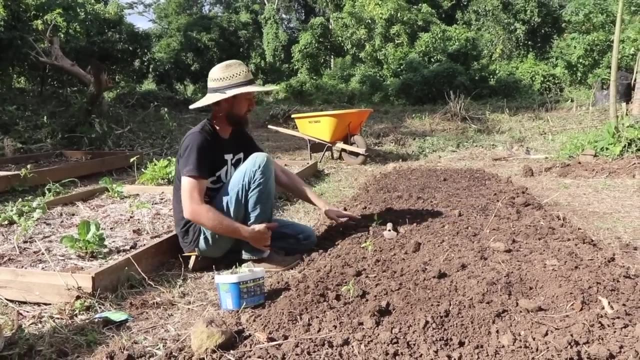 My big problem is planting all of the transplants and seeds I seem to accumulate. It's actually kind of ridiculous. What I'm putting in right now are some bell pepper transplants. I don't believe in putting them super tight. This is plenty tight. 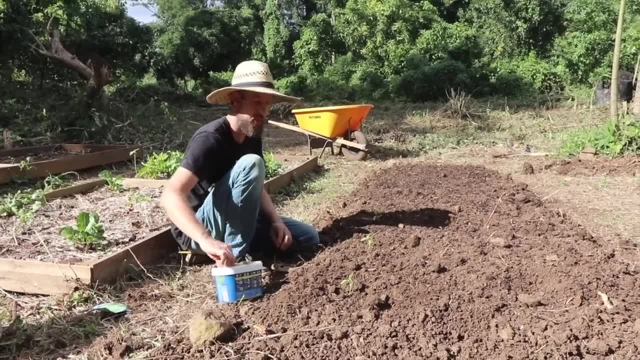 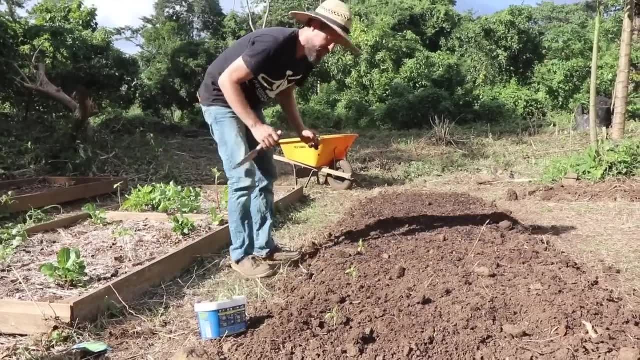 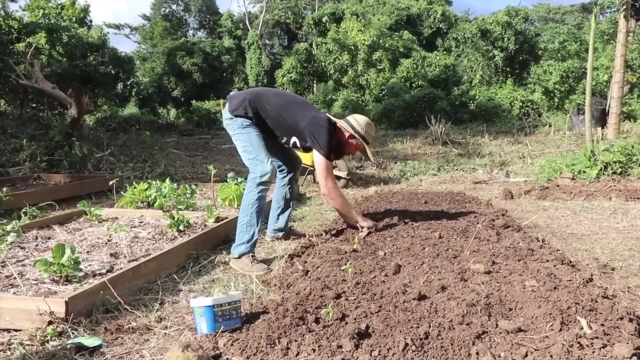 I don't like to put my transplants or my seeds too close together, because when you do that they fight, and I don't want them to fight. I don't want them to be struggling for light and resources, so I give them a decent amount of space. 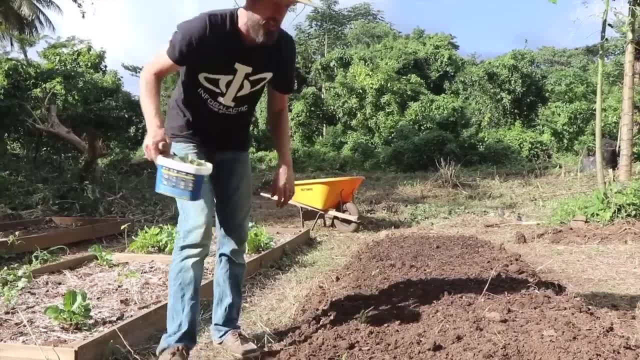 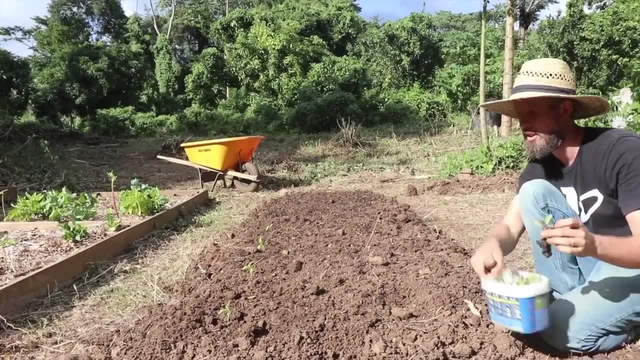 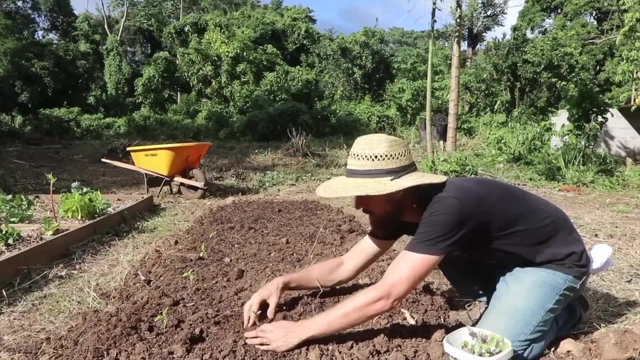 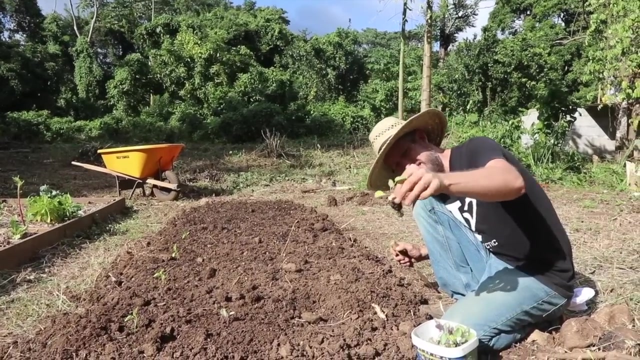 So I have here some lettuces, I have some cauliflower- I love cauliflower- And you see, I plant them to the same height that they were basically in the tray. so you look at the bottom of them and say, okay, there's my soil height. 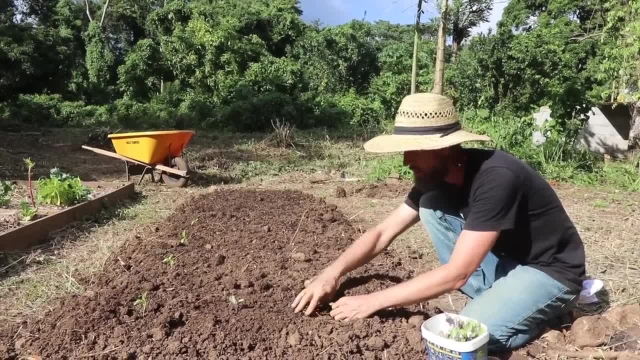 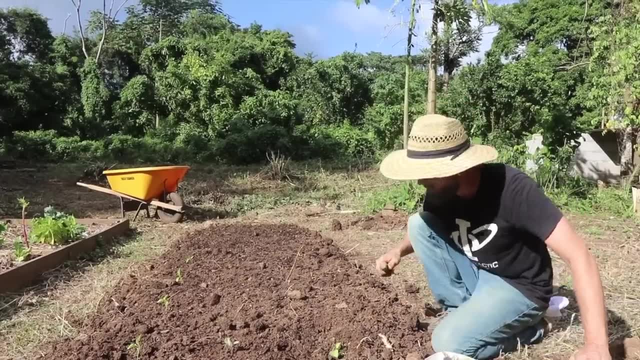 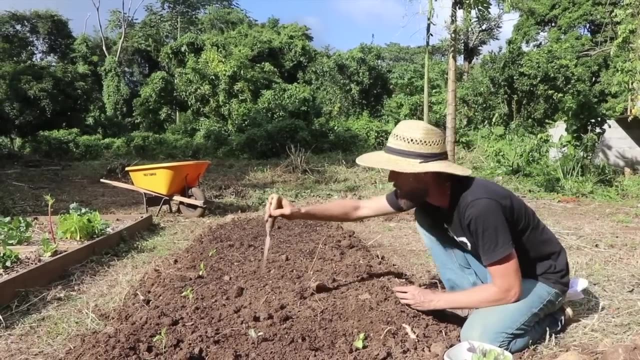 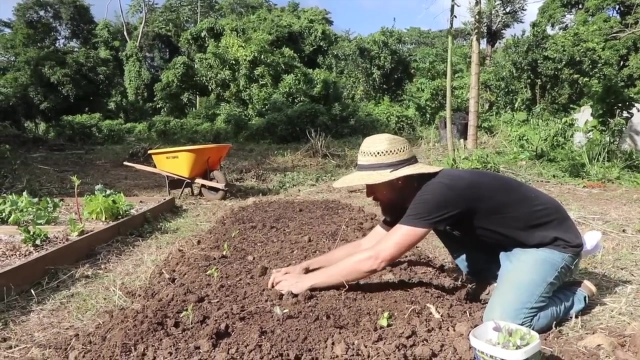 That's good Right there. Now it's important to, when you're doing your spacing, you know you don't go too tight. It's actually better to go too far apart than it is to go too tight. If you go too far apart, you just have to weed a little more in between. 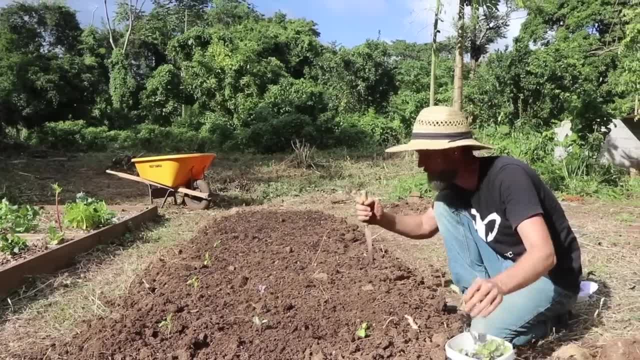 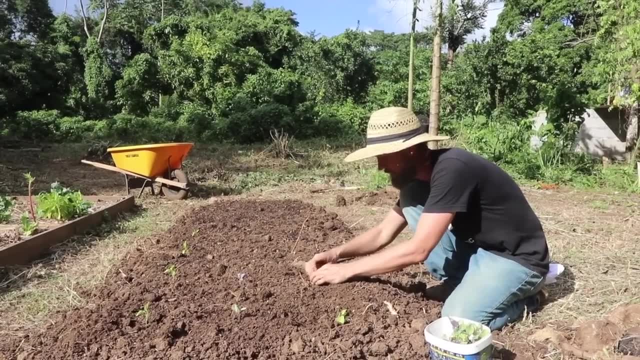 But if you go too tight, sometimes everything just strangles all up on each other and they don't produce very much. You'll actually get more production by planting farther apart sometimes than you will by planting really tightly. It's kind of a paradox, but it's like. 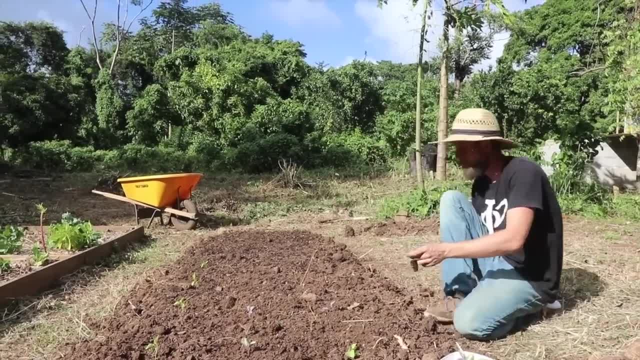 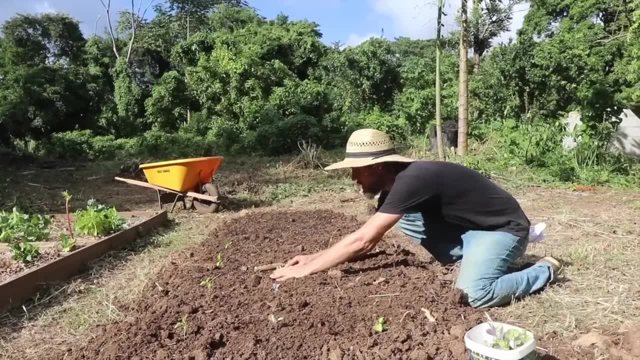 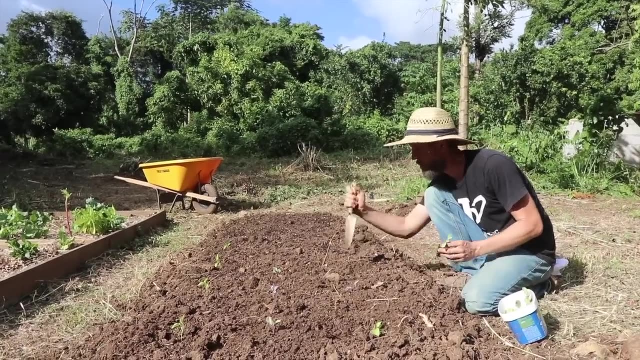 you know you think you're going to get more by cramming them in, but you don't really So if you are going from seeds, look and see what's the spacing that they recommend- Just go with that, Go a little wider. Either way: go with it or go a little wider. 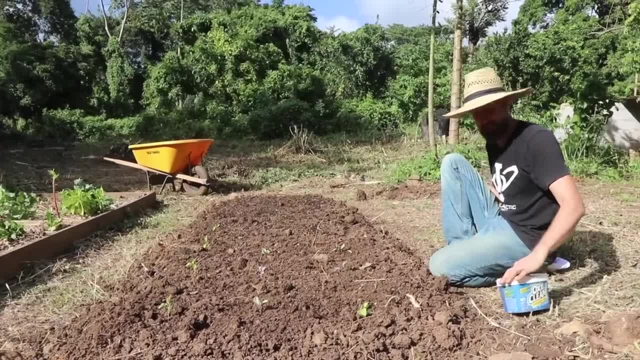 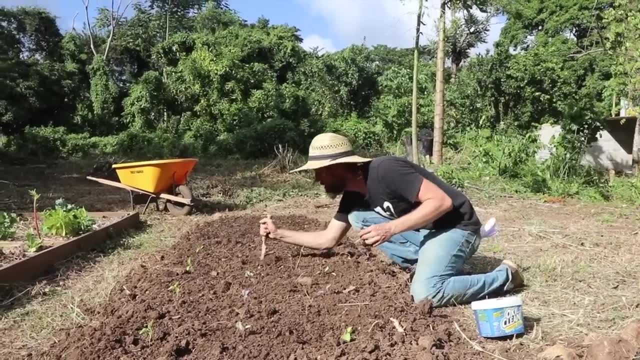 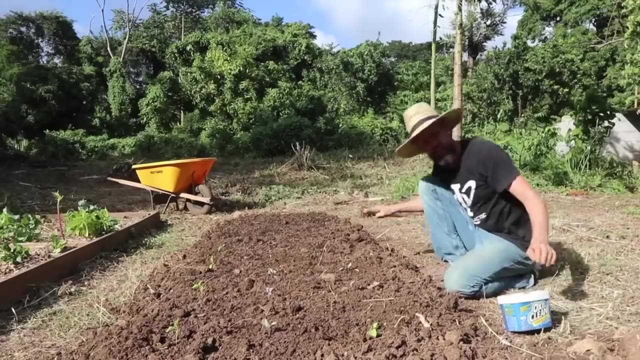 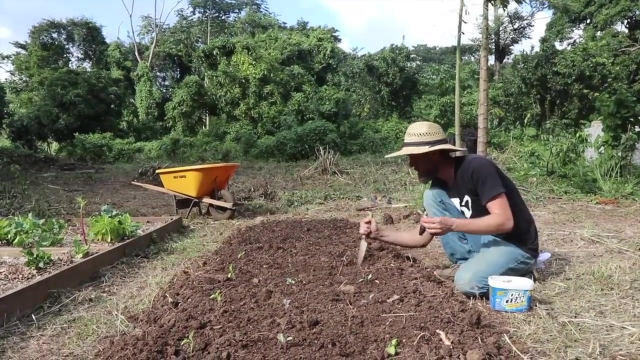 See, I'm gonna. I'm gonna plant this bed with just this little thing of transplants here. very easily I can plant the whole thing. I'm giving plenty of space. Now there's some dispute over seeds versus transplants. I got these transplants the other day. 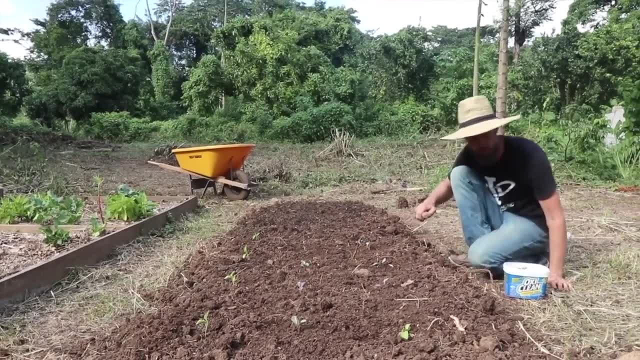 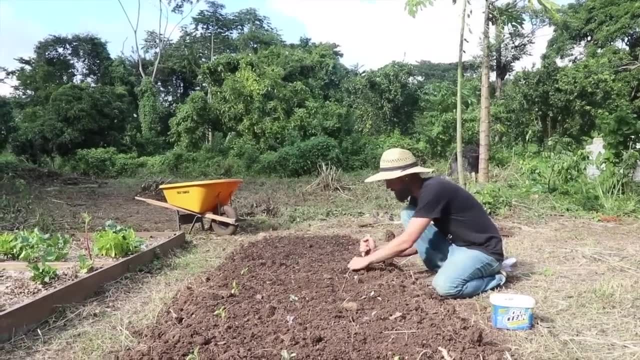 About 25 cents each from a local place. They just pull them out of the trays and you go up to the front and they count them and there you go, You've got a whole bunch of them. So it hardly costs anything and it's really easy, because I 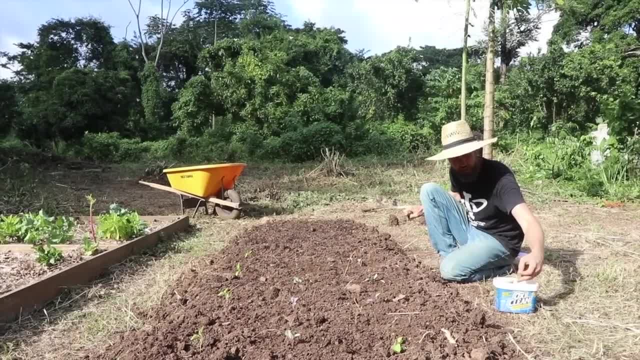 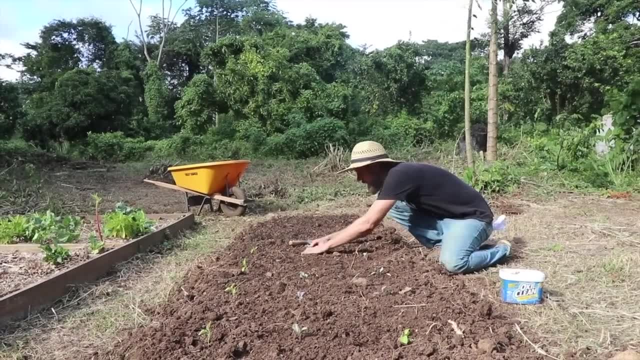 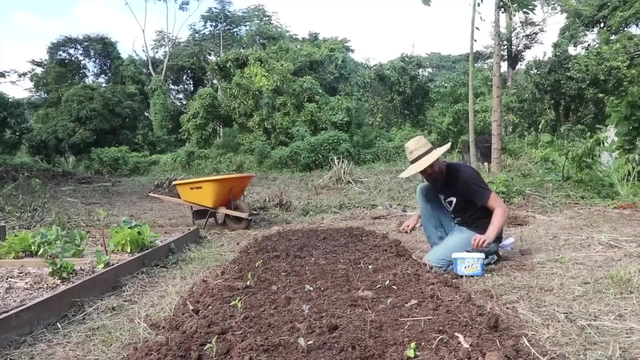 could see them already and I don't have to wait for them to germinate. but there is a big benefit to planting instead seeds, and the benefit of that is there's no transplant shock, first of all. So when you plant them, they're not just, you know, going struggling from being in a really 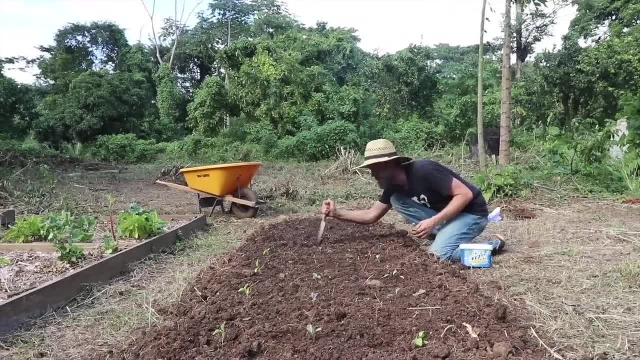 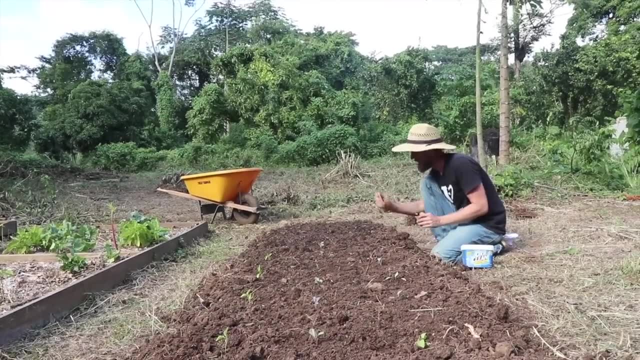 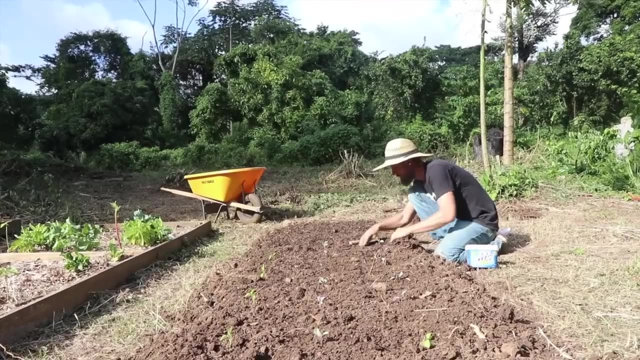 nice, perfect environment, getting watered all the time, to suddenly being out in this middle of this really sunny, hot area And suffering, and suffering, and suffering, and it's so terrible, My little baby's suffering. It's so sad. You plant them right in the ground from seed and they grow right where they are. 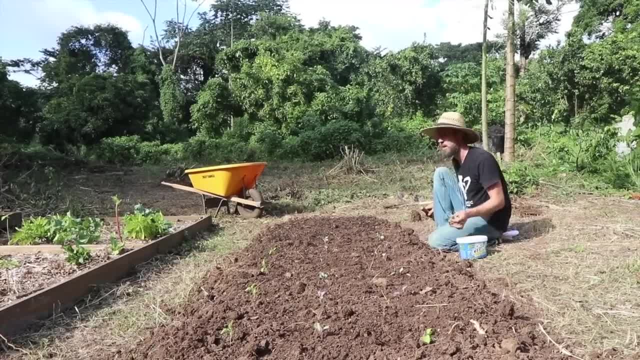 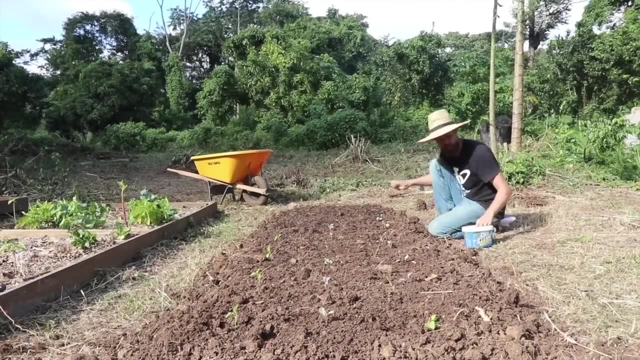 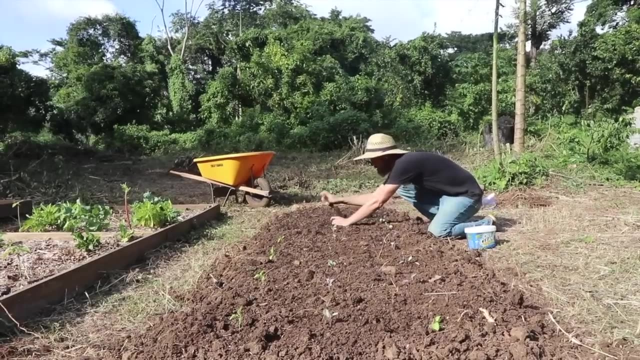 and they get strong and they like it and they're well adapted to the spot. Now, if you have a cold, colder climate with a shorter growing season, it makes sense to start transplants early. That's really the best time for doing transplants. The best situation for transplants is when you're you're in a place. 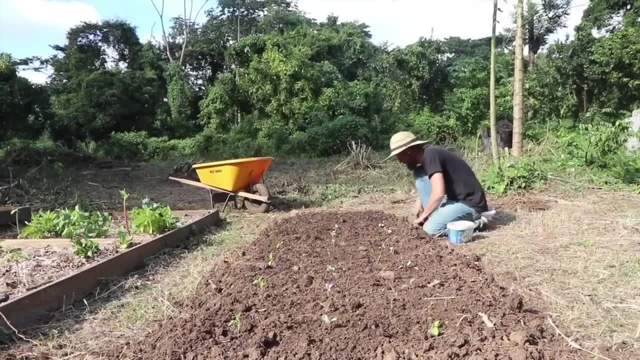 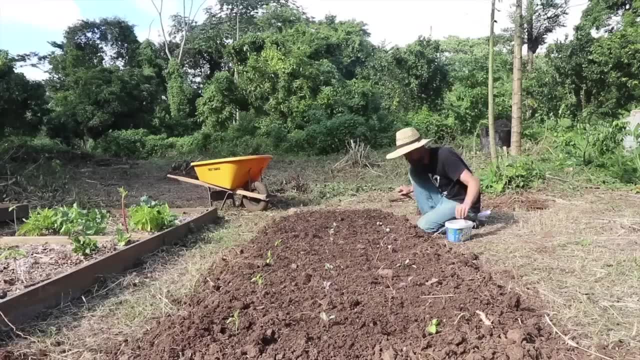 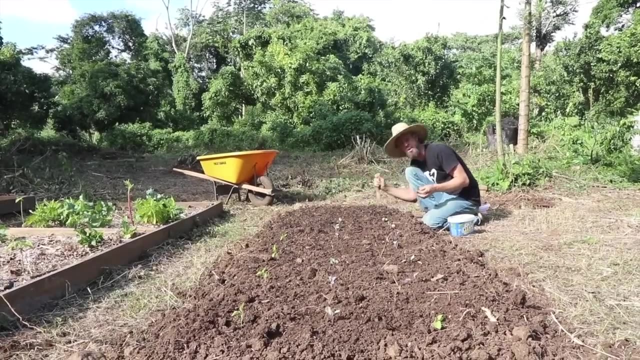 where you've got to get a jump on the growing season. You want to get something in and there you go. but you'll save a lot more money by going from seeds. There's a big benefit to that price-wise because you could pay, you know, two bucks for a packet of seeds. That might get you. 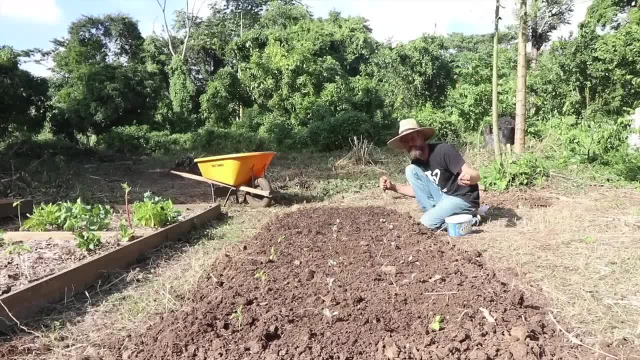 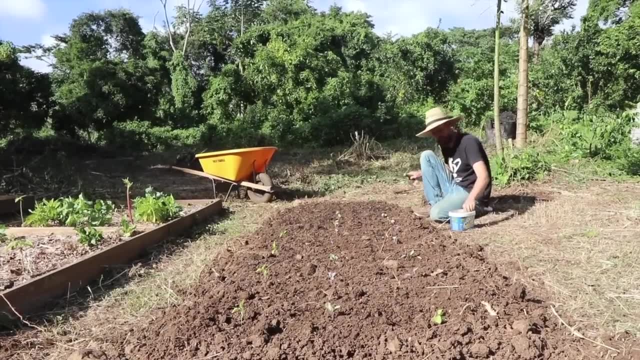 four transplants, but that packet of seeds can have 50 in it. So if you start your own transplants, you save a lot of money. Or if you direct seed, you save a lot of money. Another benefit of direct seeding is when you 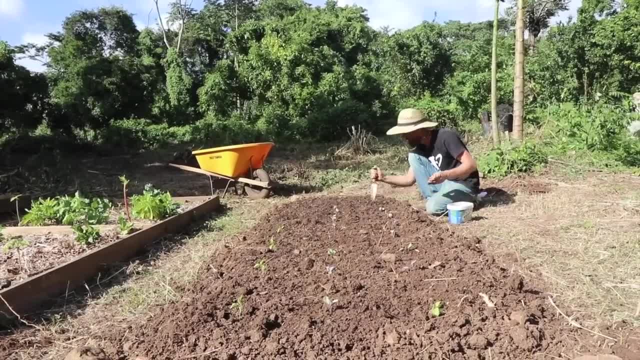 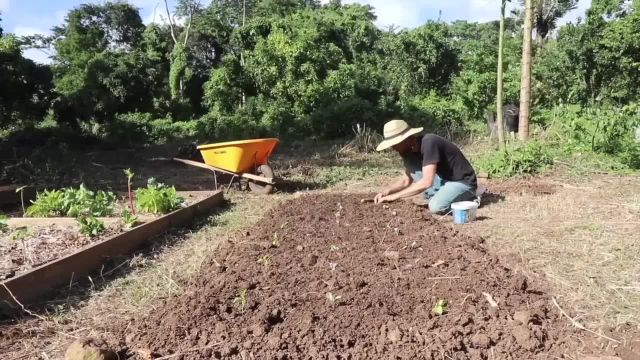 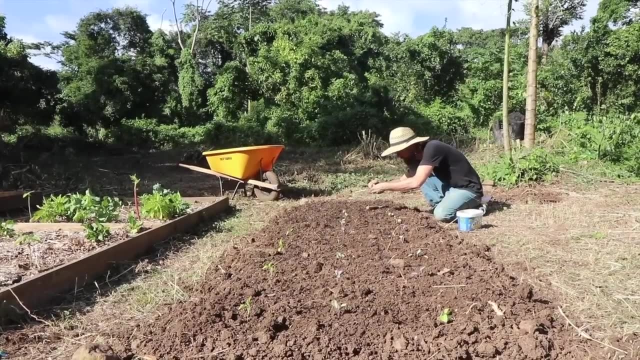 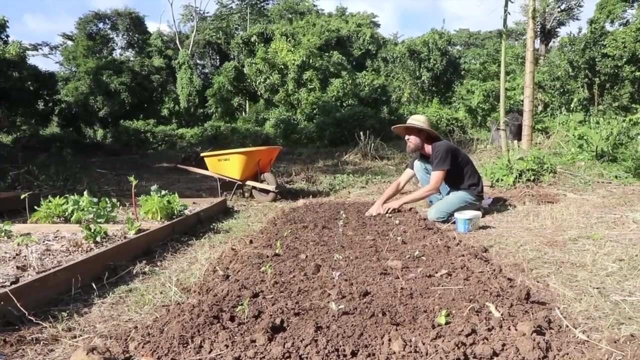 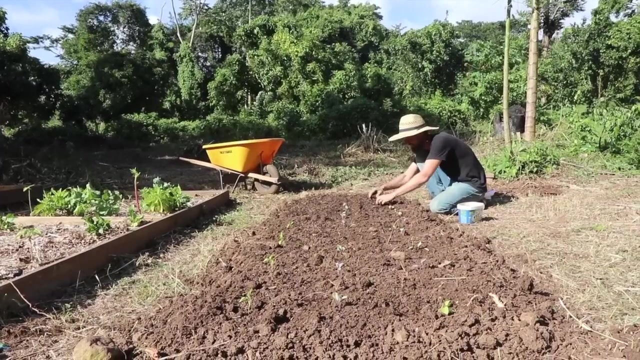 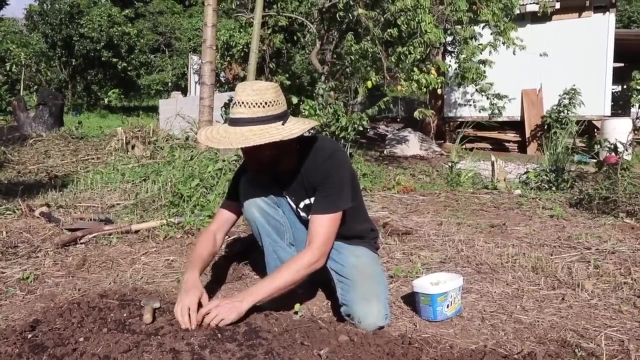 stick them right in their roots, go straight down, They get. they can go for resources quickly And an additional benefit. I forgot what I was going to say, Totally lost it. There was one more benefit with seeds. Oh, I remember. An additional benefit of going with seeds over transplants is that seeds are so cheap. 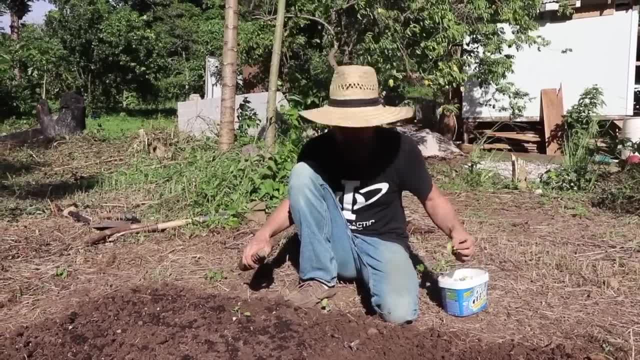 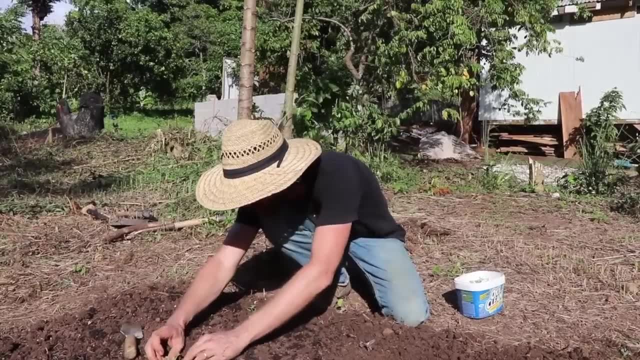 you can just throw a bunch of seeds in and whatever comes up and looks really good. then you can thin it out later. You don't really want to do that when you spend 50 cents a transplant, but if I was going to do this in seeds, I would be able to get the seeds right away. That would be great. 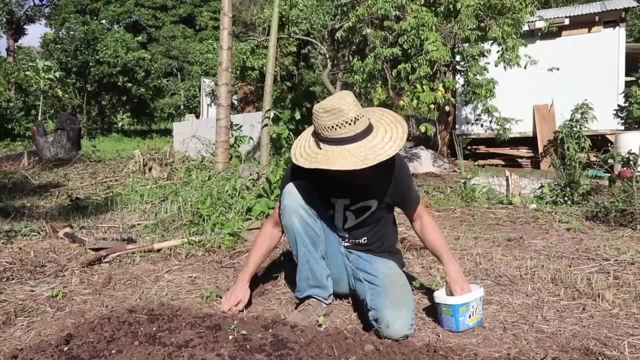 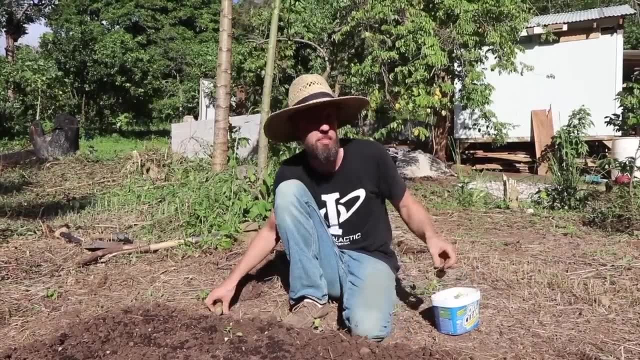 this in seeds. I would just make a furrow right down here, plant them closer together, cut out the weak ones when they come up and let the strong survive. and I might thin a couple of times until they get out to about here, and it still cost me less than a transplant. 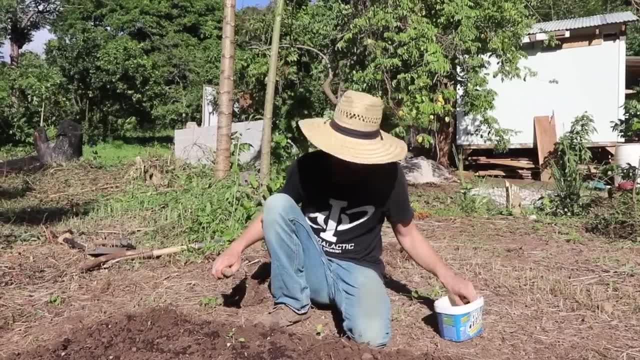 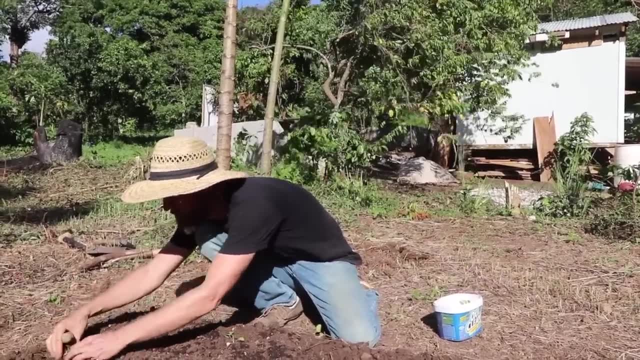 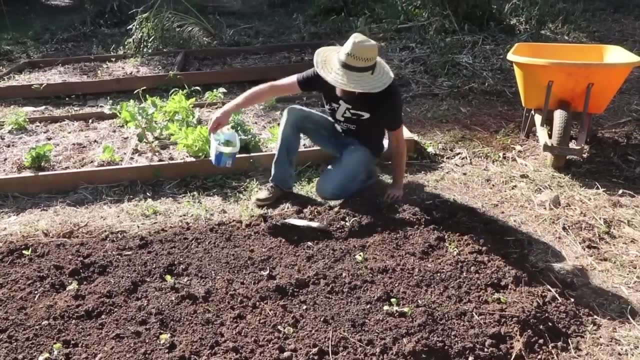 now we're planting pak choi. we have some cauliflower and then some kale got mixed in. they look pretty similar. these varieties look similar. they both have a little purple in their leaves. look at that. while I was prattling on about seeds versus transplants, we pretty much got the whole bed planted. takes way. 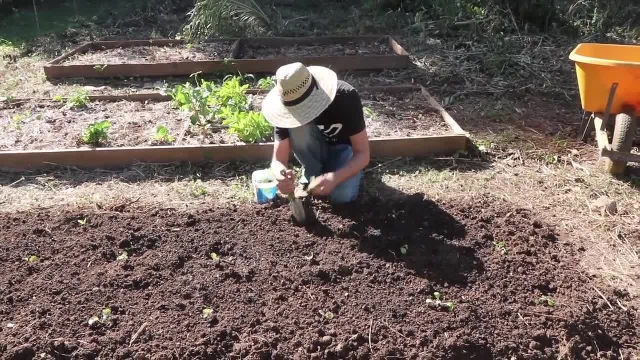 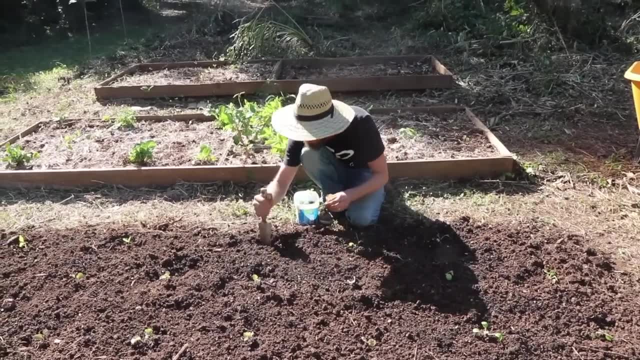 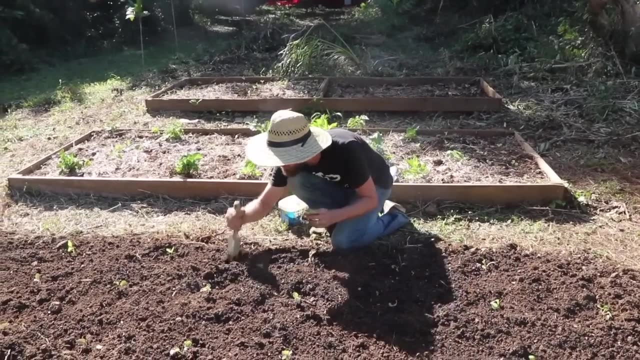 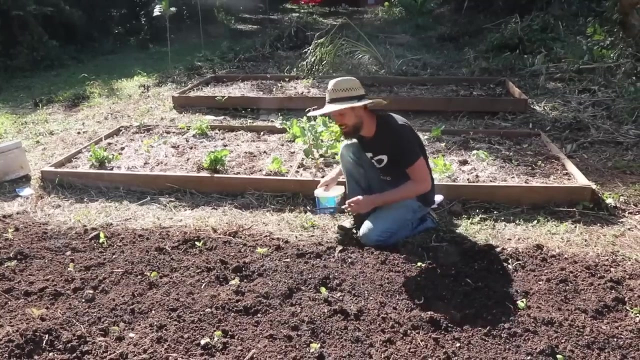 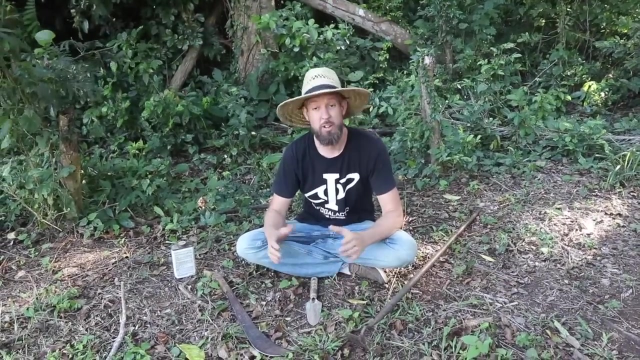 longer to dig it than it does to plant it. all right, space for you. I've still got transplants left over. I have to have my daughter dig it for me. another bed: there's my last bell right there. look at you. there we go. that is satisfying folks. let's talk a little bit about tools. you don't need fancy. 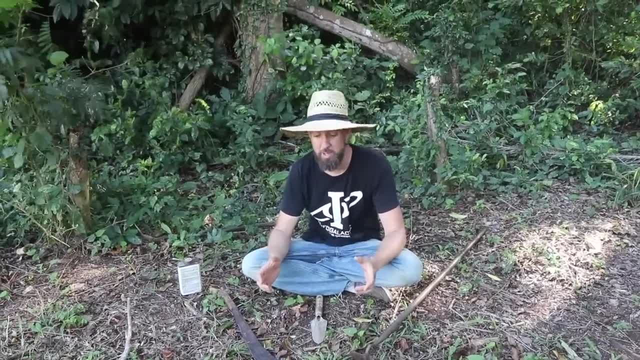 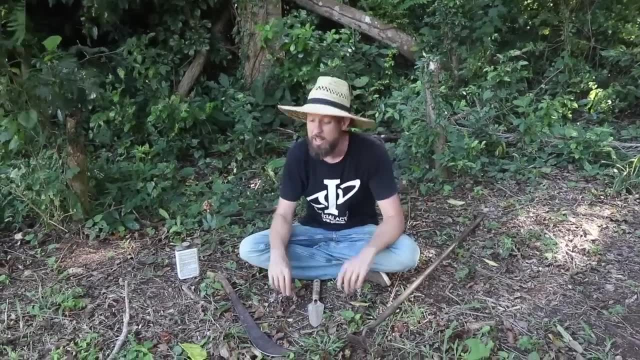 gadgets. I mean, you don't need a big composting tumbler to make compost. all you can do is just take a few pallets and lash them together and throw compost on the inside of it. just throw everything in there to rot. you know, you don't? there's usually an easy way to do that, but I don't know if you've ever done that. 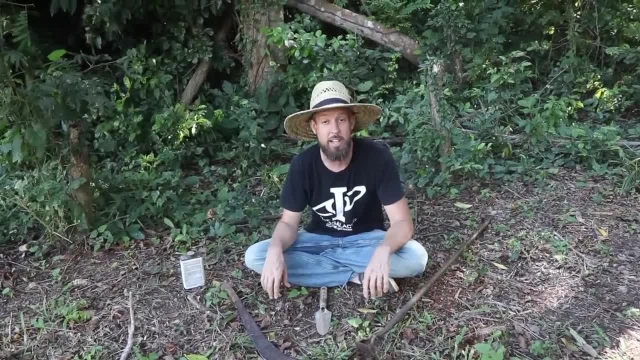 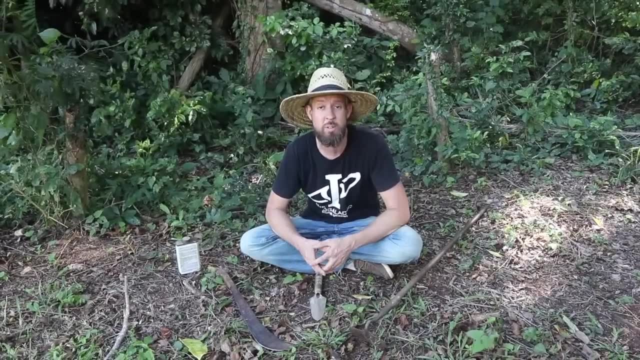 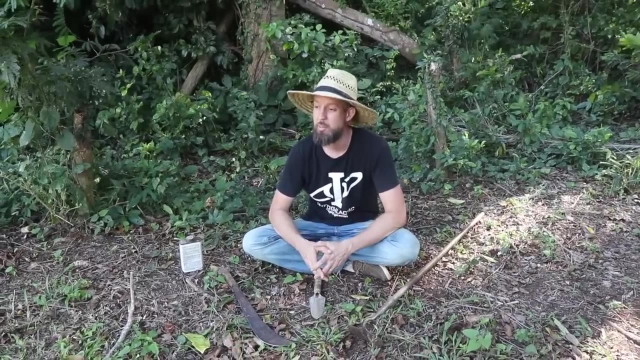 you don't need to go buy something in the back of the gardening catalog that's really complicated to turn the ground or whatever else. I find myself using the same simple hand tools over and, over and over again. I don't have a whole ton of gardening tools. I have more than average, but I don't have a lot of gadgets I have. 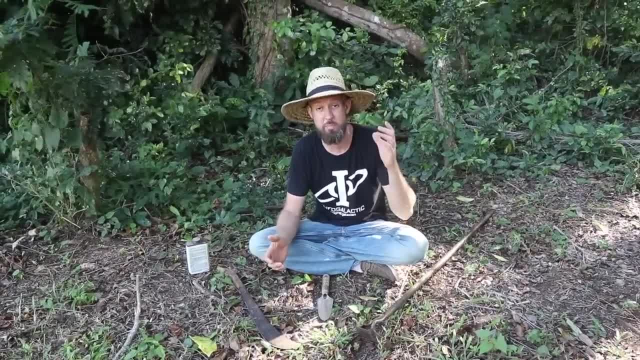 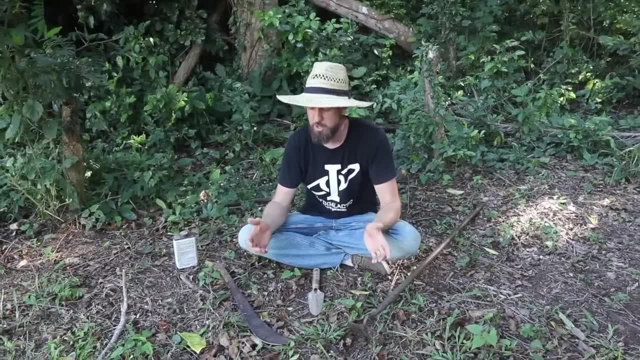 good, simple tools. so you've already seen my spade and my fork and I use for double-digging or for loosening the ground. that days they get used for planting trees and the fork gets used for loosening, and you know there's a lot. 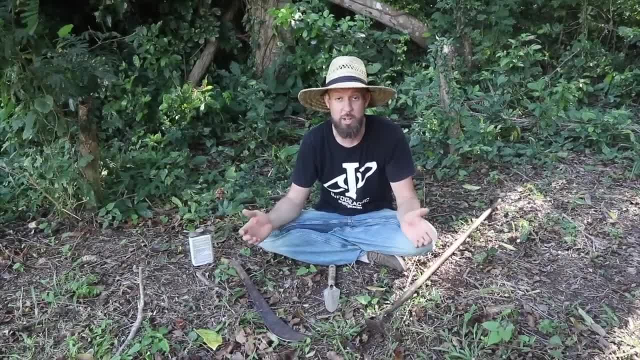 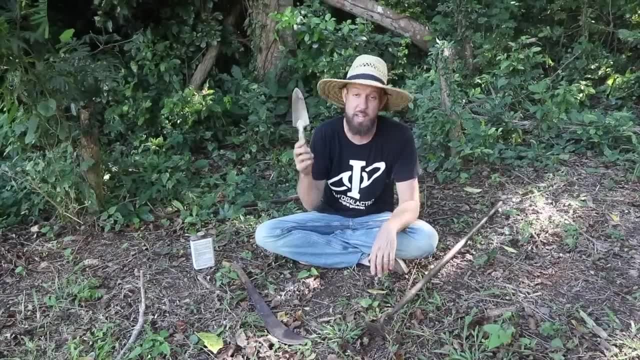 of use that just any good spade or shovel will give you. so that's, that's so simple. we're not even gonna talk about it. and you've seen my little trowel. one of the kids gave me this one as a gift and you know you don't actually need a. 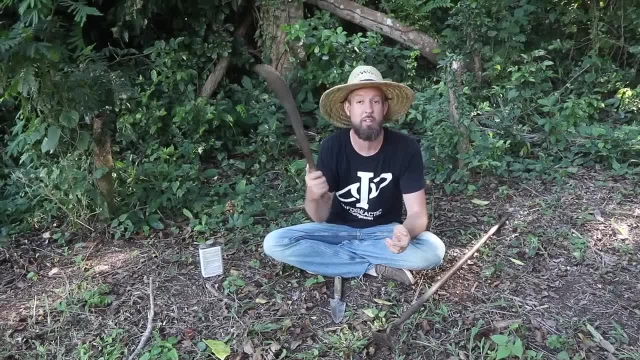 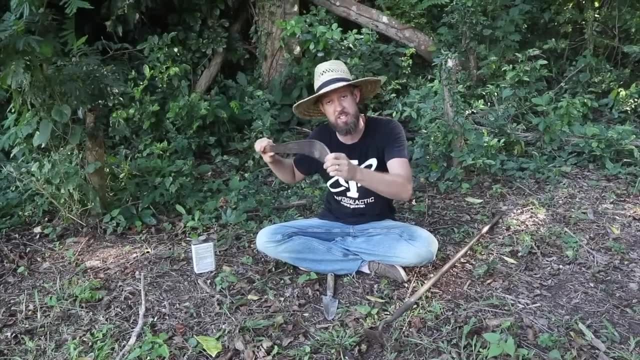 trowel if you have a machete. machete is one of my favorite gardening tools. this is a nice kind of short, simple type. when it's got a little bit more space in the ground, it's got this: get this nice thick steel to it. this is a Martindale. I. 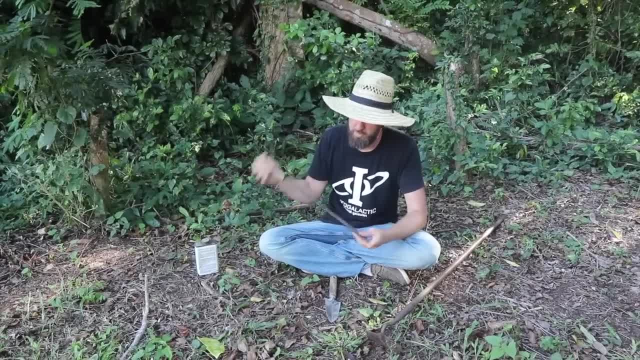 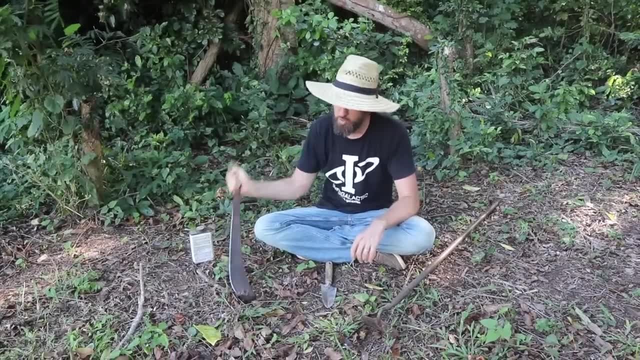 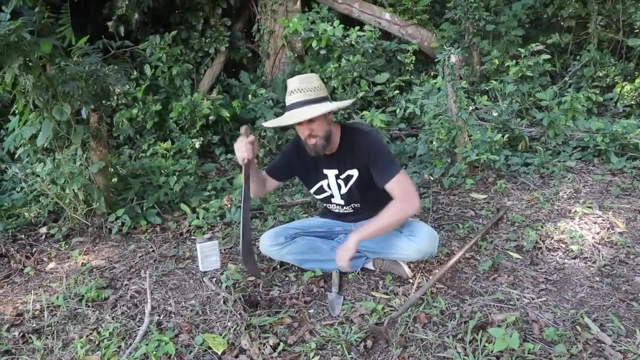 think it's called a mongoose. so this style here is actually quite versatile. you can use this instead of a trowel. I could just dig in the ground with this actually very easily, and you can just kind of crouch, whack it in the ground, stick a transplant boom, whack it in the ground, stick a transplant in. you know. 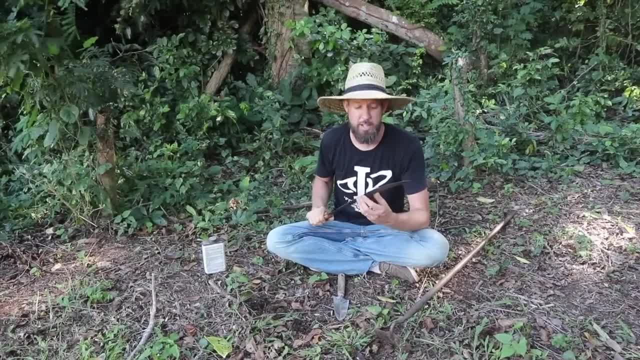 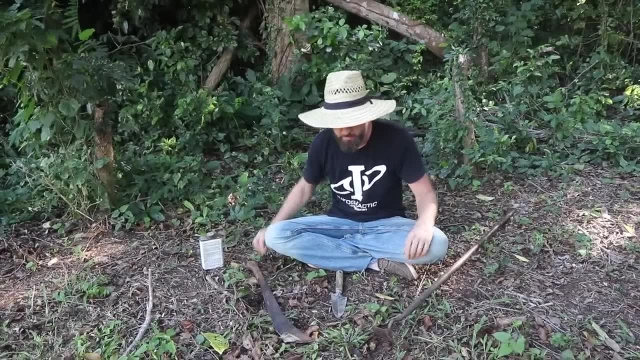 and you can chop through roots, you can take down brush, you can chop up stuff before you throw it into the compost pile and you can compost your enemies- the other tool that I find using a lot during the season after I've planted, when the weeds start coming out. 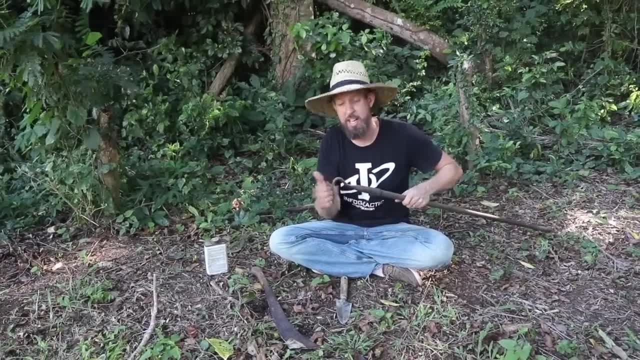 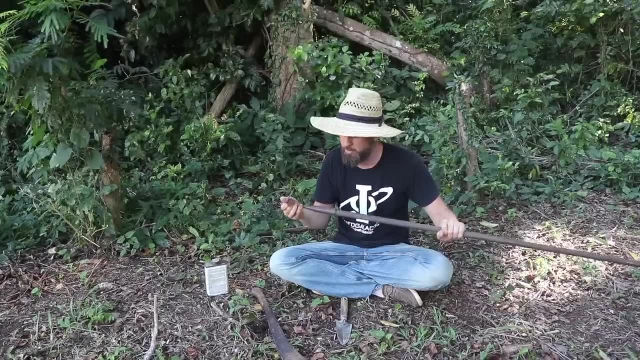 and being a problem. it's just a regular old garden hoe. this is an antique that I got on a date with my wife. when we were in the town of Micanopy in Central Florida. I saw this in an antique shop. I bought it for 15 bucks the one solid. 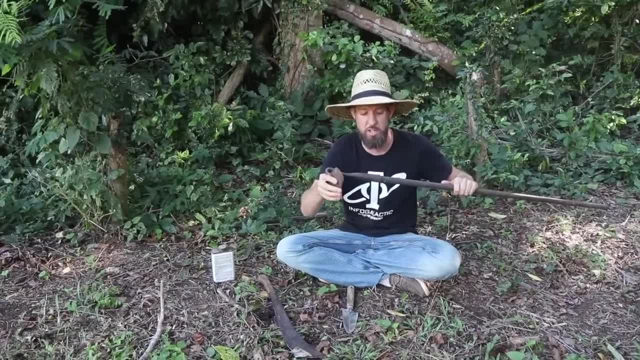 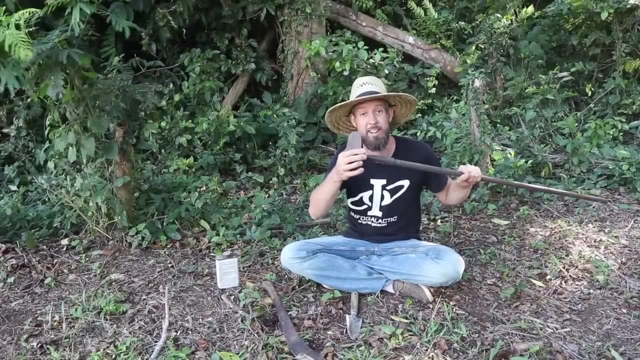 piece all the way around. this is an old-style one. the new style ones are made of crummy or metal. they don't hold the blade. you might not have thought about it, but this is a blade right here. so when you see, you know you're hacking at the ground with a hoe. it's not the right way to do it. 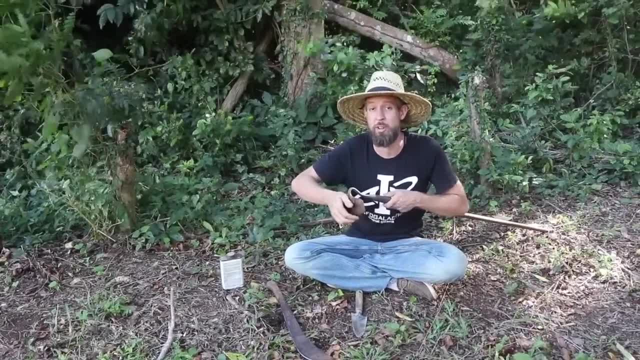 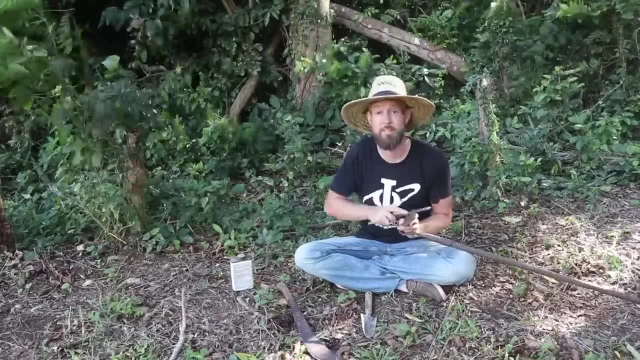 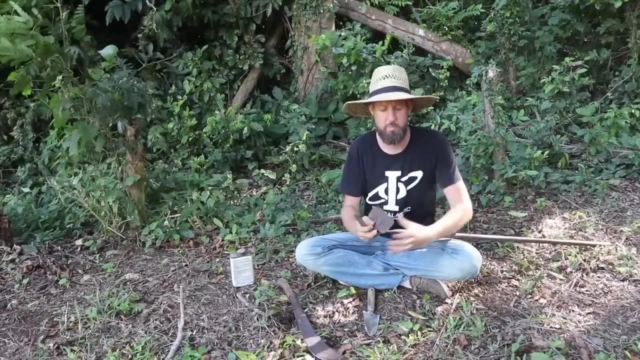 you should be able to, with a small amount of effort, do the hoeing that you need to do in order to do that small amount of effort. sharpen the blade so you get your. take that old hoe out of the workshop or wherever you have it, back in that dusty corner with all the torture. 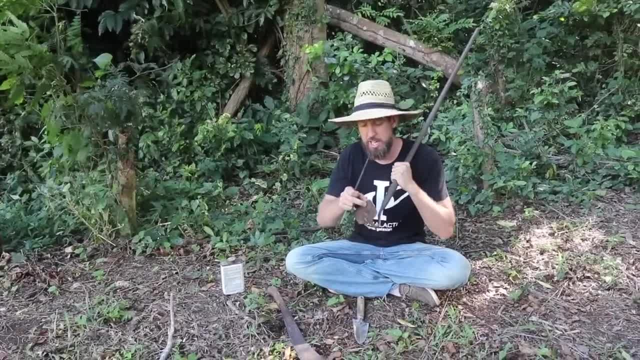 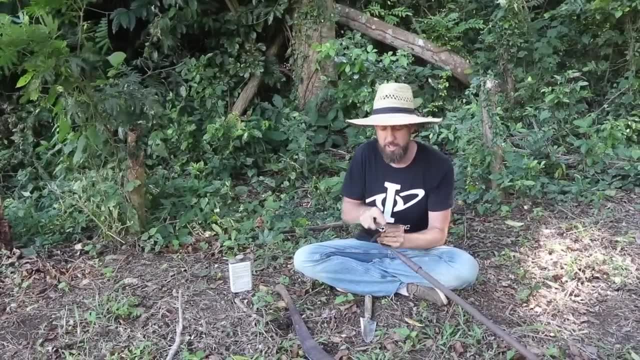 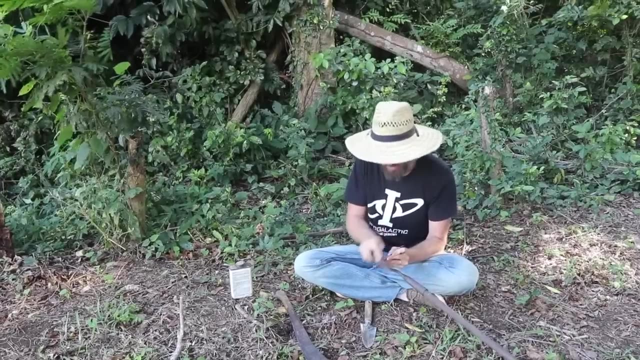 implements and put a nice edge on it. this one's got a ding in it right here that I have to hammer out, but otherwise I'll just put a nice blade on it. you also want to make sure that you bend this head right here, so this has a good 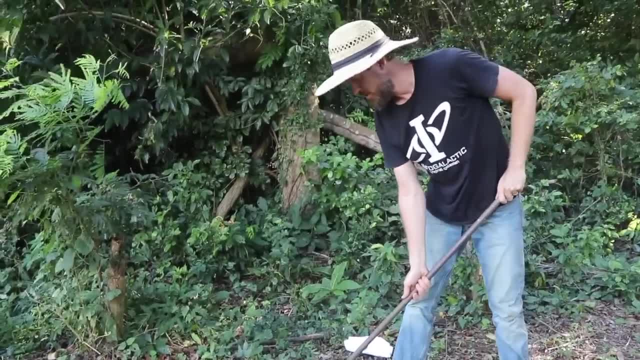 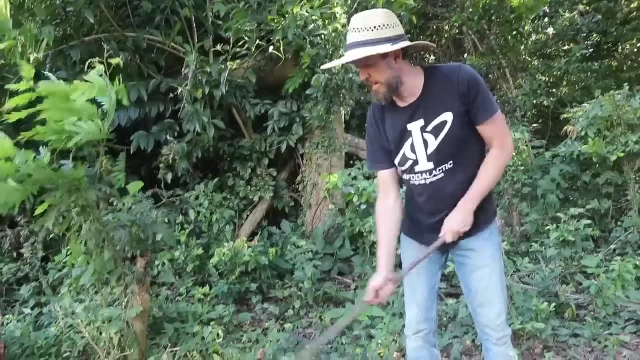 angle. so if I'm standing up, This shouldn't be, I shouldn't have to do like this or do like this. it should be at a good cutting edge to the ground, so when I'm at a comfortable angle I can just go along and weed like this. 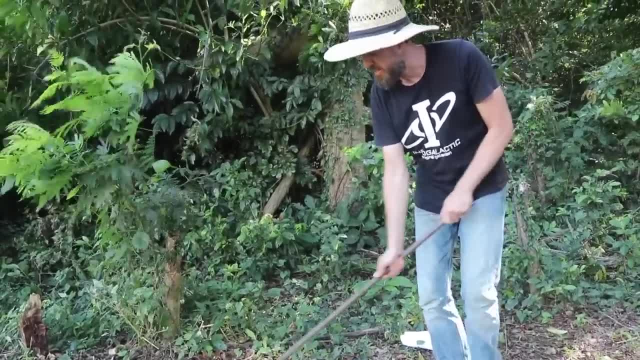 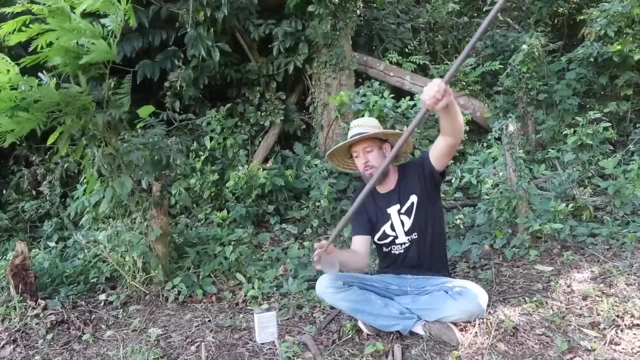 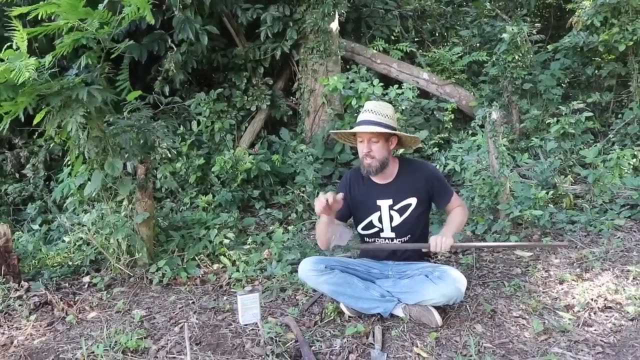 The idea is to decapitate the weeds. the idea is to decapitate the weeds, not to chop big divots in the ground. You want it to kind of go along the ground. that's why it has that angle, And if you have nice loose soil, like in your well dug beds, it's very easy to use a hoe. 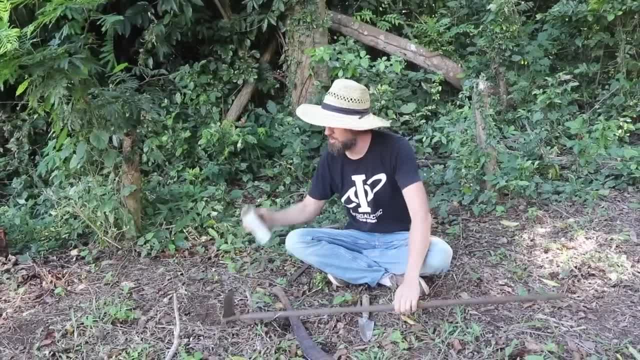 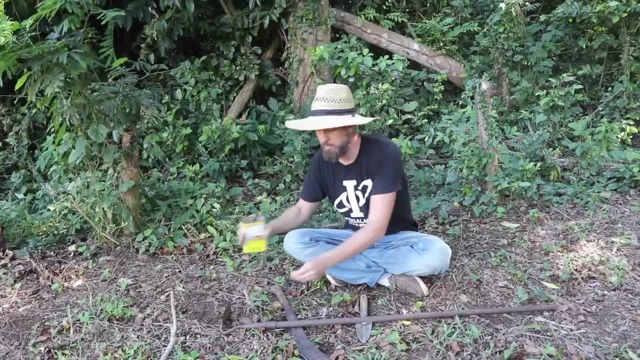 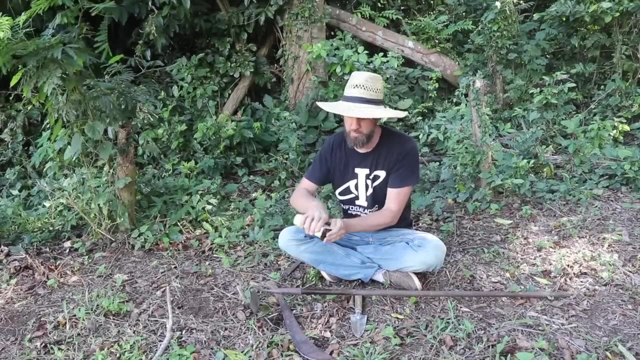 So once you put an edge on there, make sure you take care of the wood handle too. This is linseed oil. the boiled linseed oil dries faster, but my friend Steven Edholm of Skill Cult thinks that they probably put some sort of weird petroleum stuff in it, or 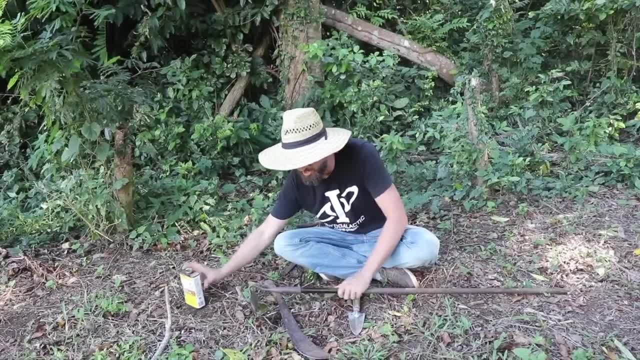 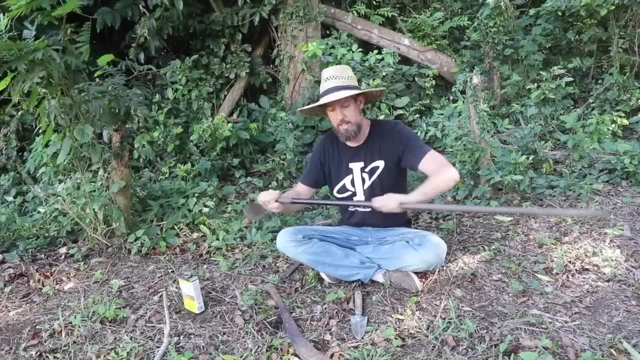 something. so he doesn't like it as much, I will use either. I'm not actually all that picky, But what you do is you just oil it. Oil up all the wood surfaces and this oil will soak in and dry and it will make it last. 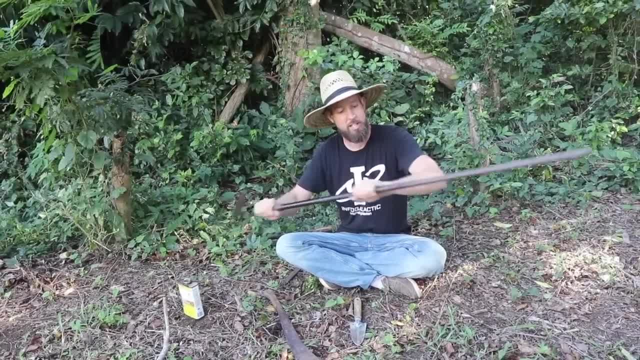 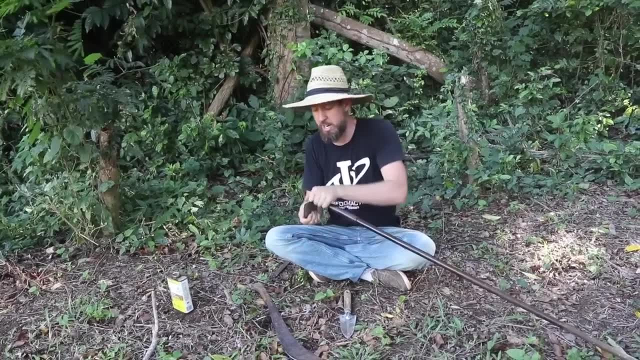 longer help. keep it from dry rotting, give it a little solar protection, keep it from wet rotting too, And now you've got a nice, happy handle. I'll actually oil the entire head when I do it too, just to keep it from rusting. 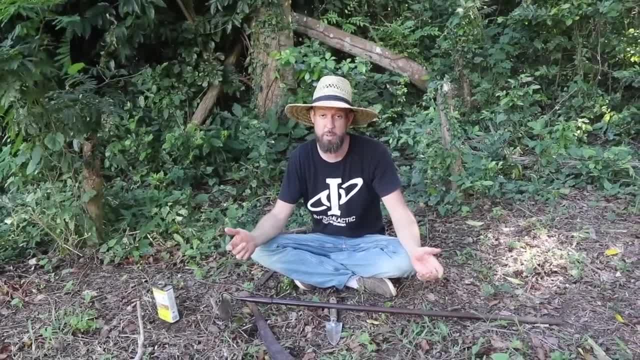 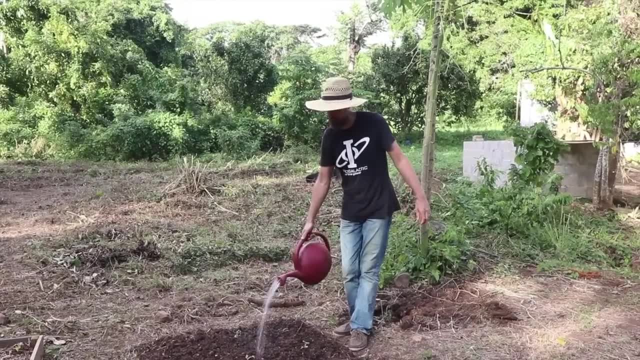 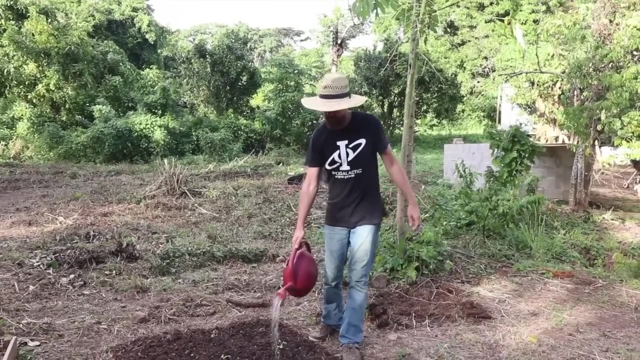 And that's it. These tools are pretty much all you need for a good, simple, frugal garden bed. I know this is about starting your first garden, But I would be remiss if I did not give you any idea about ongoing care. 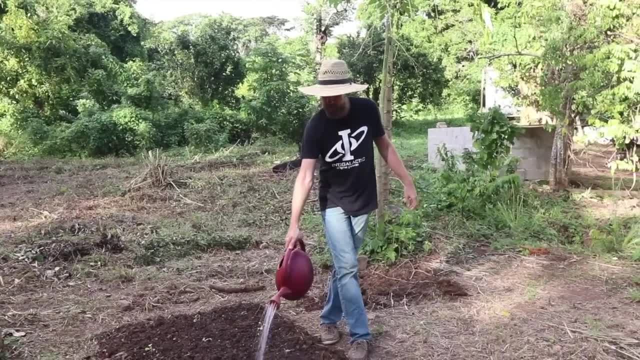 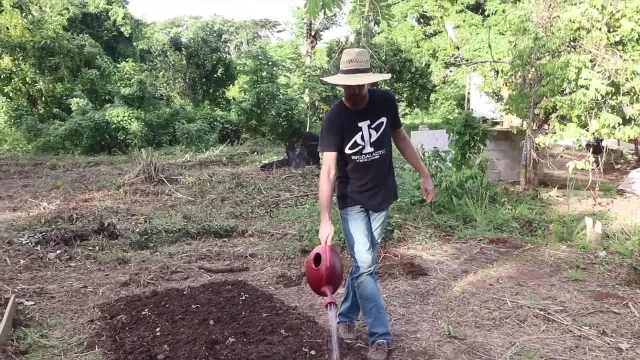 Obviously, when you put in transplants or you plant your seeds, you want to water them. You want to keep them watered. Watering is one of those things that gardeners like to dispute about. Personally, I'm a big fan of garden hoses. 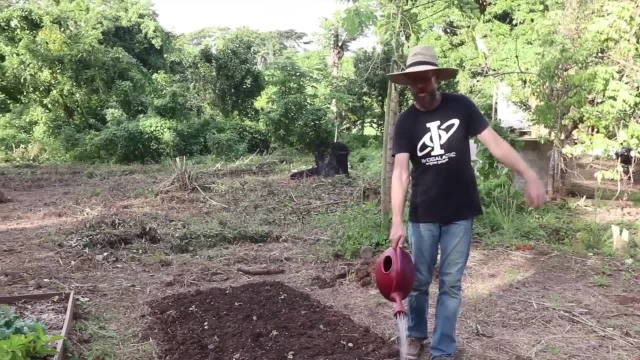 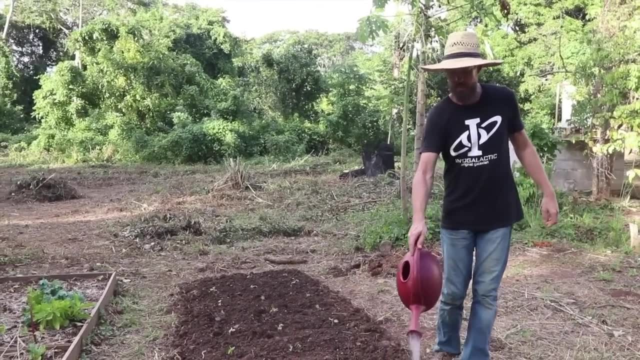 I like to come out when I have a few garden beds and just spray water them as I go. That is fun. It's nice because I get a chance to go out there and see what each garden bed is doing and go Sometimes like right here where my garden hose doesn't reach. I'll just take one of. 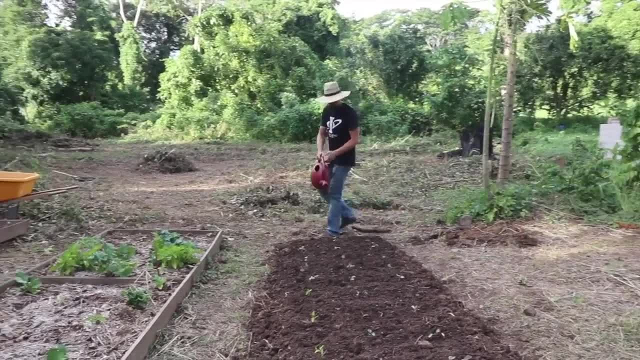 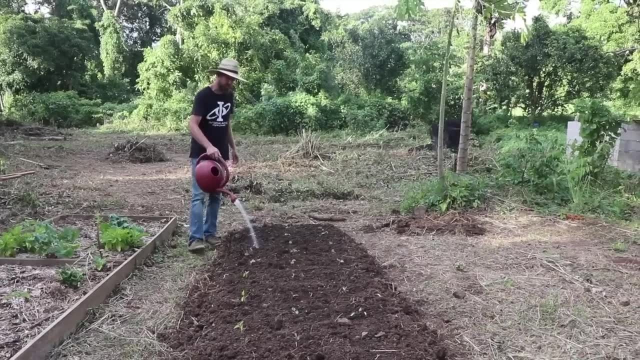 these two gallon watering cans and I'll just walk along and I'll just give everybody some care And it gives me an idea. okay, do we have any bugs? do we have any issues? is anything gnawing on the plants? does any of them look like they're getting yellow, like they're? 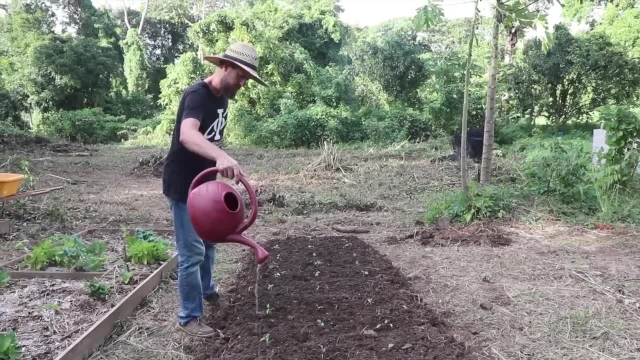 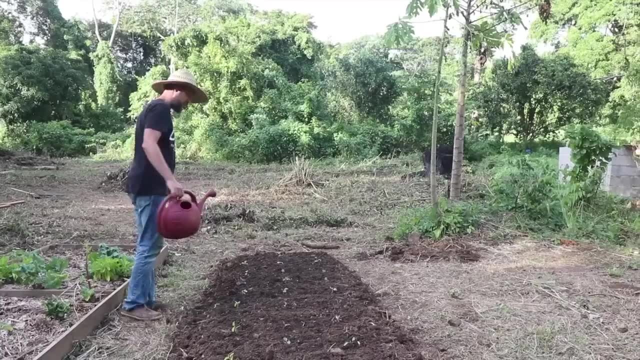 hungry, You know, And then I can just take care of them as I go, And that's it. Thanks for watching. Here we go. But the argument comes with: what do you do? do you put sprinklers in? A lot of people will say, oh, don't use sprinklers. 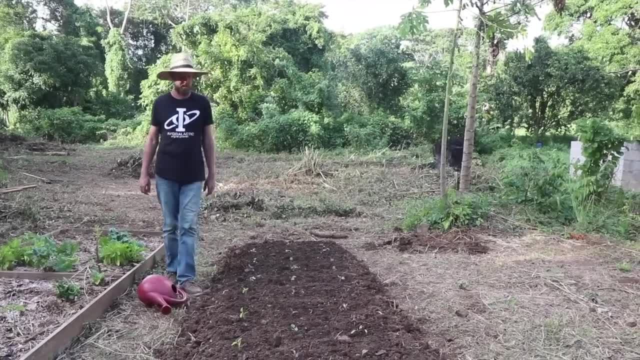 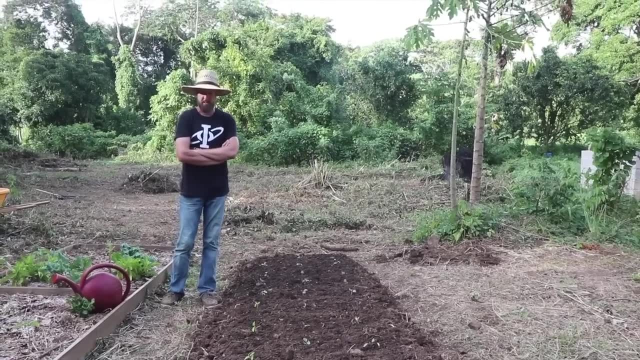 You want a drip irrigation system. you want to get some soaker hoses or something like that. I actually don't like doing that. The reason I don't like doing that is because in Florida the squirrels will bite holes in the soaker hoses for one. 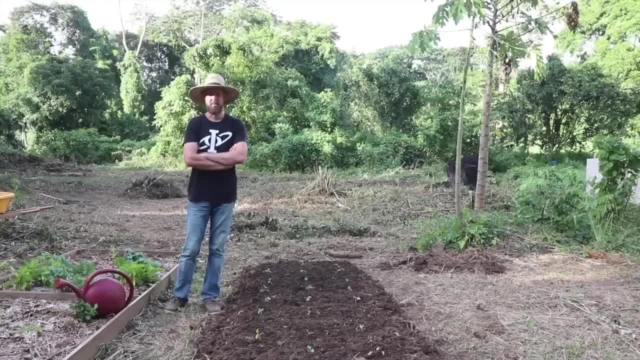 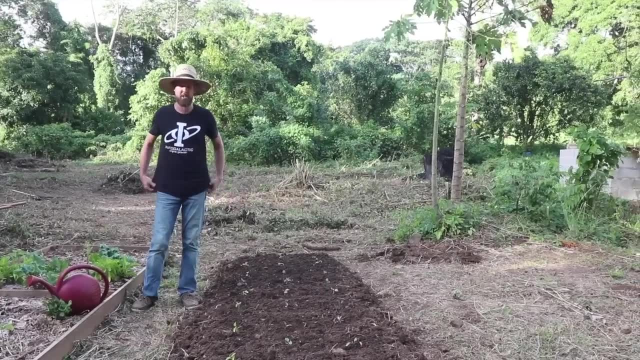 But also I don't like plumbing. I don't like plumbing. I don't like to have to haul these things around and I'm always changing the configurations of my beds and digging things in different places and planting trees and stuff. So having a bunch of bits of plastic soaker hose 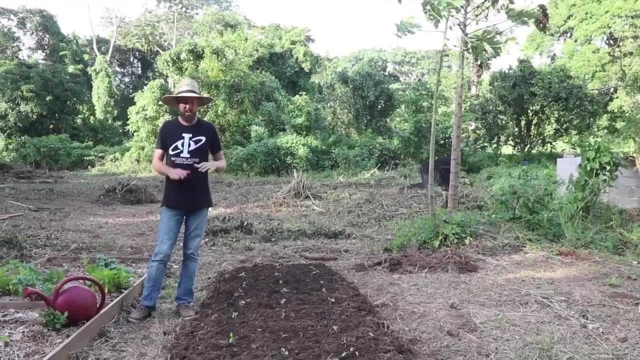 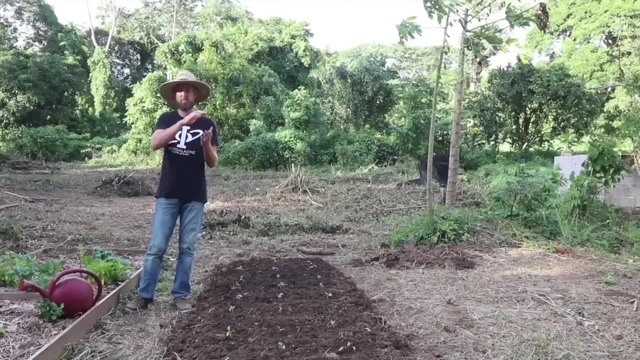 on the ground. I just really don't like it. So when I had a plant nursery and I had about 20 garden beds going, what I did is one day I had a friend of mine come over we bought some Rain Bird sprinkler heads. 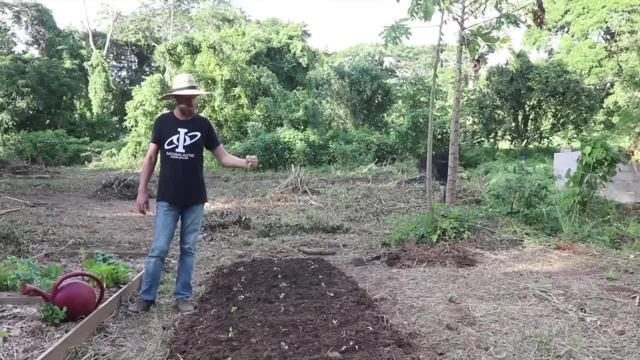 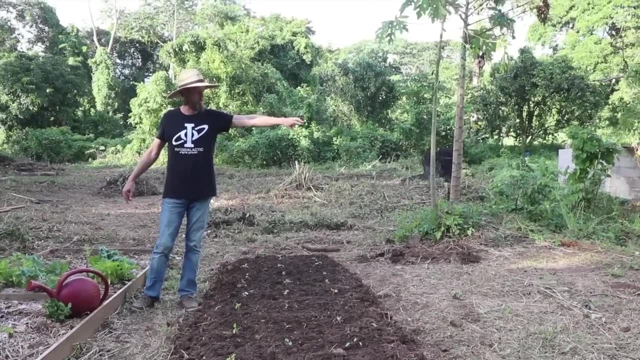 and we made stand pipes. So we stuck some pieces of rebar or something in the ground like this high, tied the PVC up to them and just ran PVC pipes to a little on nozzle and just boom, we turn that thing on. the whole area rains. 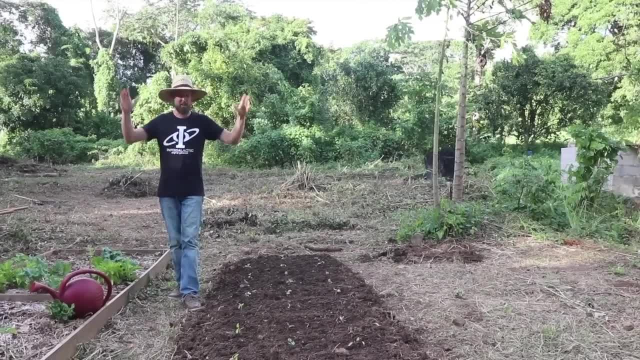 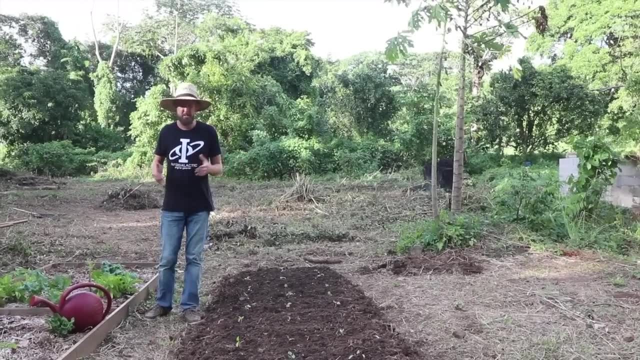 So you get it to the Rain. Birds overlap each other and it acts like rain. It just comes down and waters the area and people will say, well, you're losing a lot to evaporation. Yes, that's true, But I really hate having to deal. 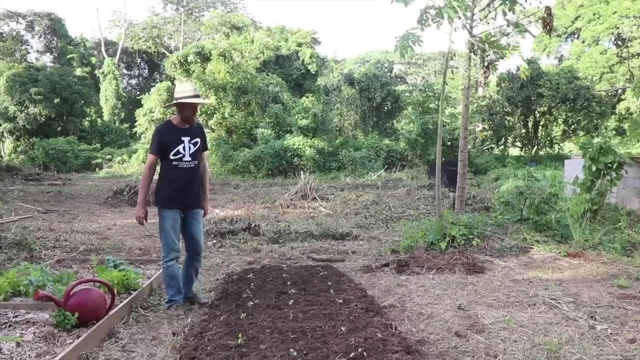 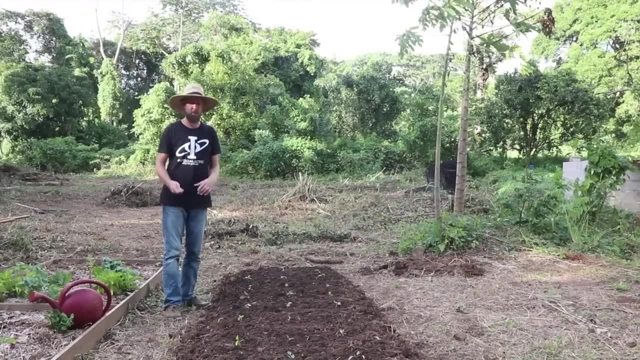 with all the little fiddly bits of a drip system. I just don't like to deal with it Now. if you want to do it, if you want a drip system, go ahead and do it. If it gets any more complicated than a few beds. 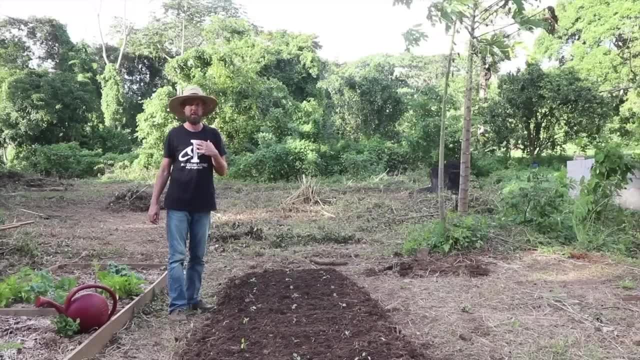 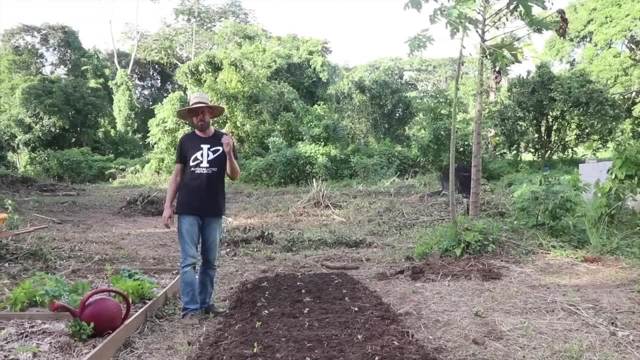 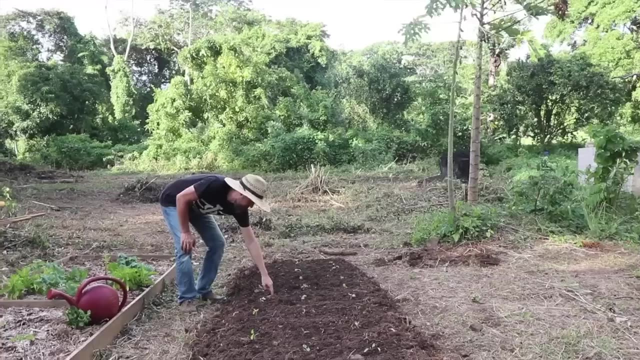 that you water with a hose. I just prefer to put stand pipes up. Eventually, I might just put stand pipes over this whole area, or I might not. I might just garden with the rain, which is the simplest option of them all. So the important thing is if it starts to get dry. 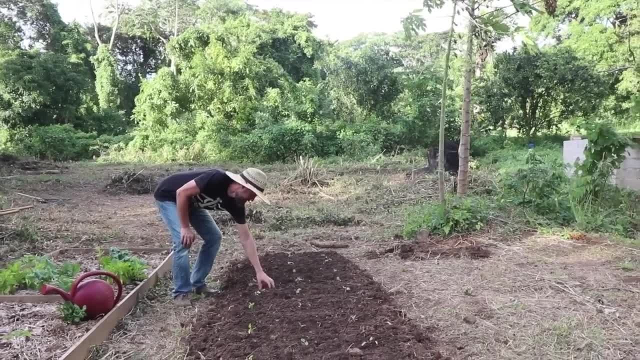 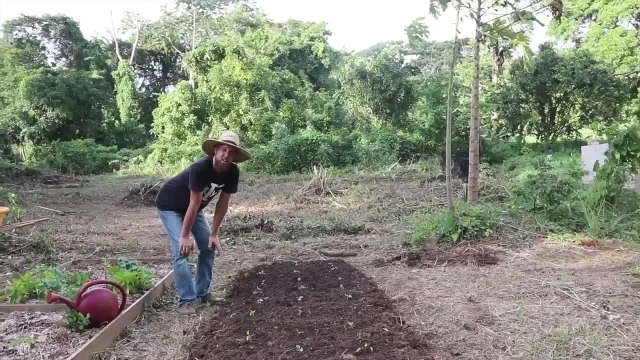 in the ground you stick your finger in and it's still dry underneath there, then you got a problem. You're going to have to water, So pretty much going to water every couple of days in the summer, When it's in the spring and fall and it's a little cooler. 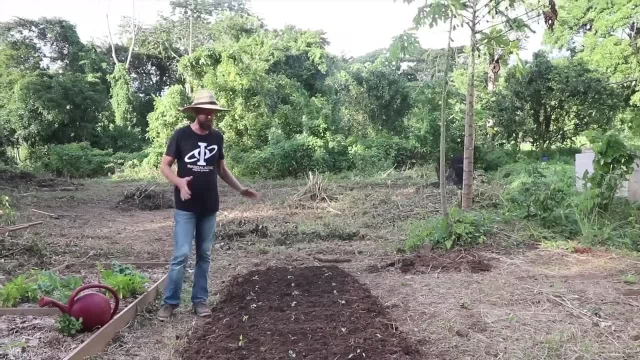 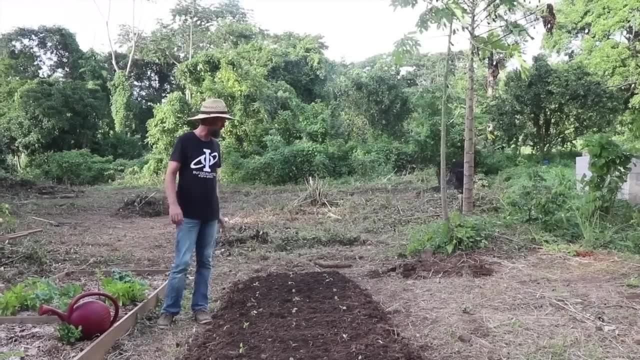 generally you can get away with watering once or twice a week. If your plants are closer together, you have to water more. If they're a little further apart, you generally have to water less. So important thing is just make sure they get water. 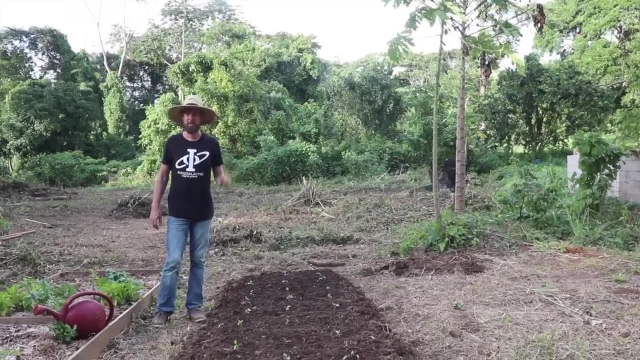 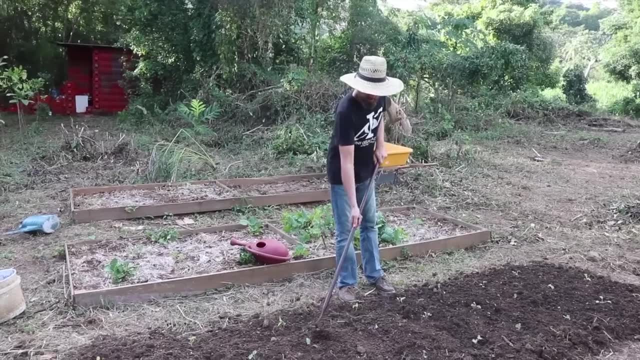 because that is the big limiting factor. The plants will die first without water, faster than they would die without any kind of food. Now, within a week or so after you plant your bed, you're going to have to start weeding. So, like I said, you get your hoe really sharp. 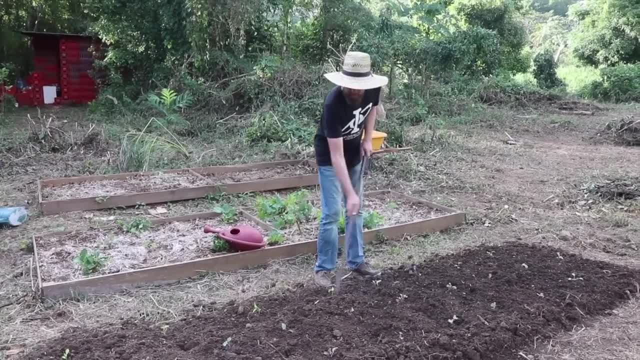 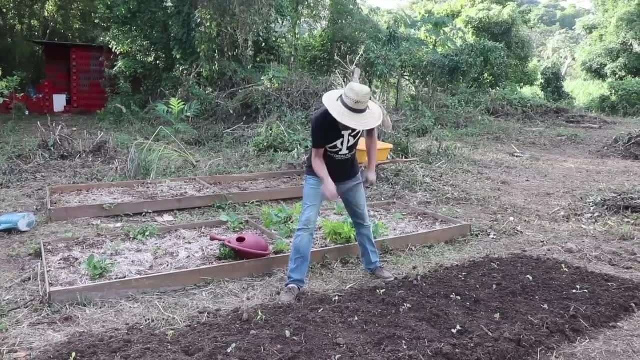 You just kind of go around the plants like this And the idea is is, if you get the weeds when they're small and knock them down, they don't get big. When they get big, you're going to be like die, die, die. I hate you, I hate you, die. But when they're small you're just kind of: oh let's see, I'm just going to kill a whole bunch of little babies, no big deal, so easy, right. So you just go in between, you know, taking them out. 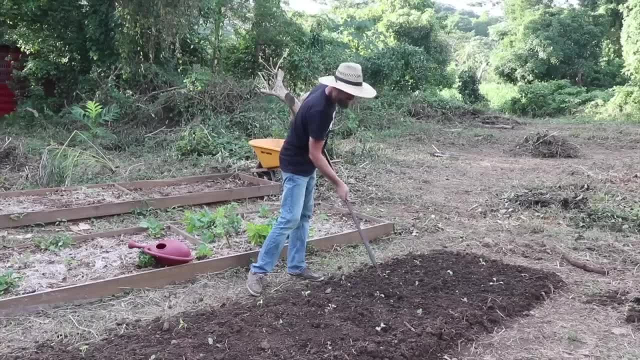 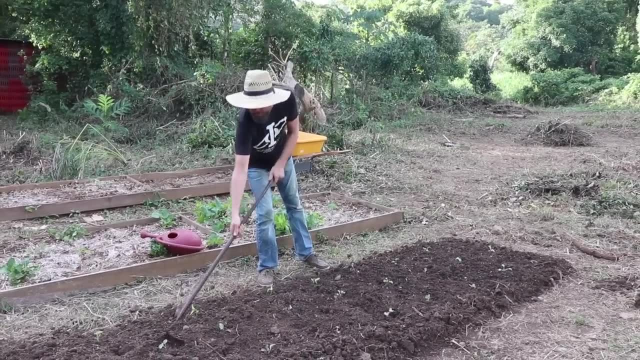 as you go And it's a nice task, But if you let it go very long it gets to be ridiculous. It's really easy when they're small. You're like there we go gotcha, there we go gotcha. 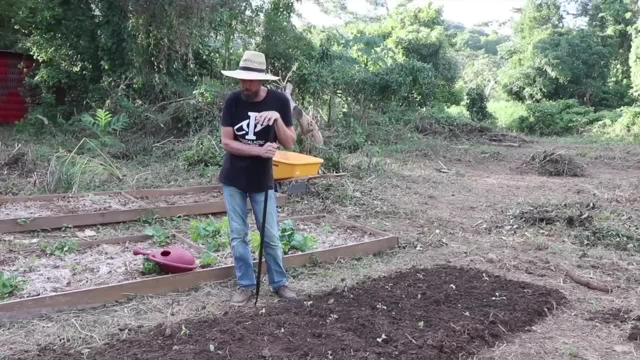 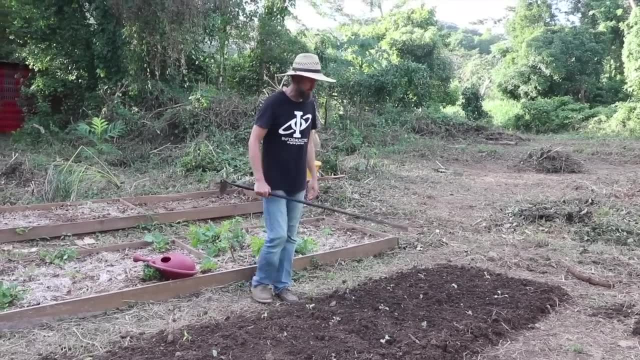 Just stay on top of it through the growing season because it will get away from you and then it gets to be a major pain in the neck. As for pests, when you see something you know, when you see a plant that looks kind of sick and weak. 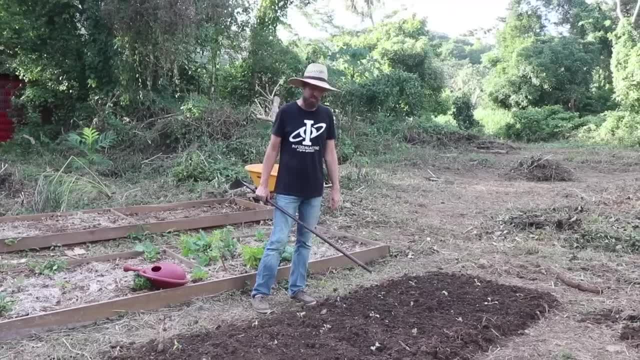 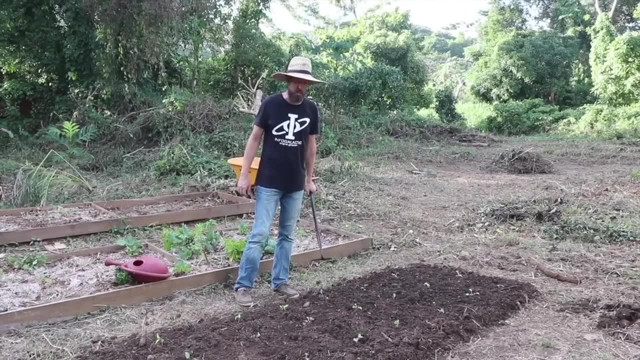 and it's got bugs all over it. I generally just let the bugs eat it because I figure they're distracted by that sick ugly plant. I don't mind if I lose a few, It's fine, And generally the ladybugs are coming up from behind. 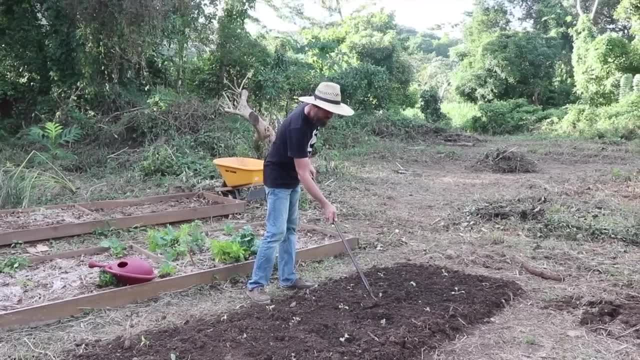 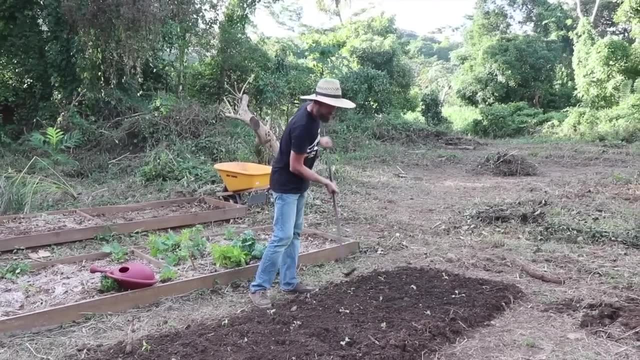 somewhere to come and get those pests. But if you get an infestation where multiple of your plants are all getting taken out at once or something, I just recommend you go around with a little bowl of soap water and you just knock all the pests into it. 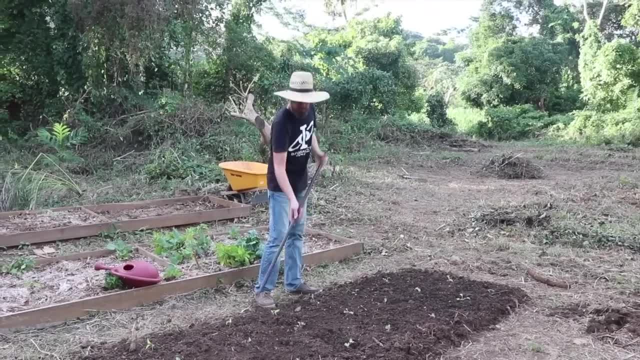 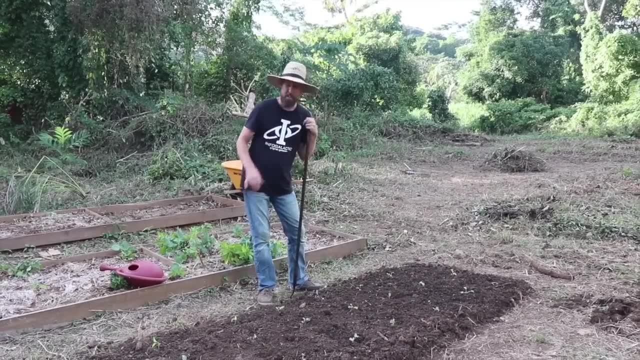 squish them with your hands, knock them into the bowl, let them drown, and then throw the whole bowl of soapy water and dead insects into your compost pile. Pick them up, Take them off as they go, though, and keep an eye on it. 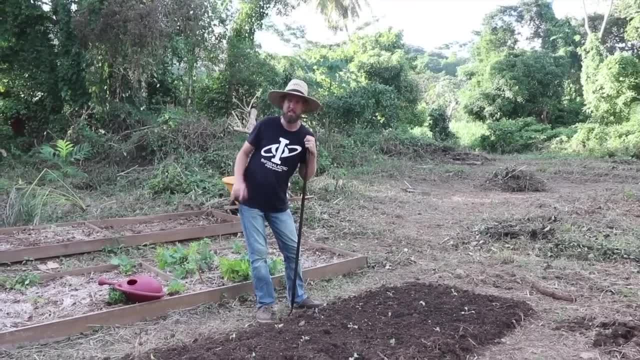 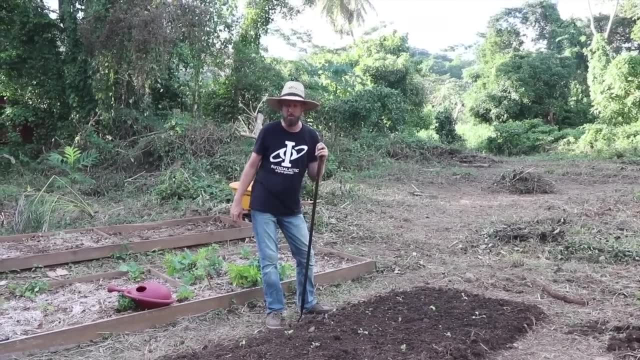 Put your garden bed too far away from your house, You're not going to keep your eye on it. It's important to put it in a place where you're going to see it and check on it, because something like hornworms, which are a big, terrifying green worm that grow on tomato plants. 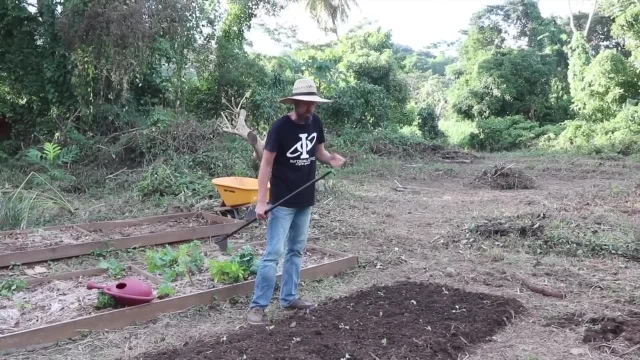 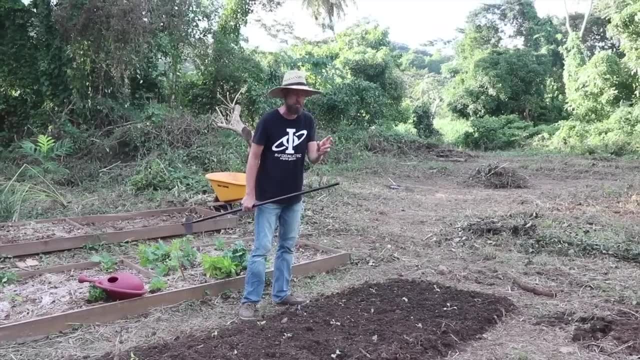 and tobacco plants. they could just completely defoliate a plant in a couple of days, So you want to catch them when they're small and get rid of them, instead of coming out and finding a worm this big on a big stick. that used to be your pride. 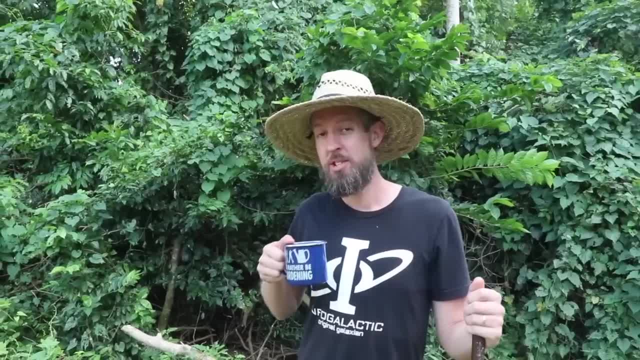 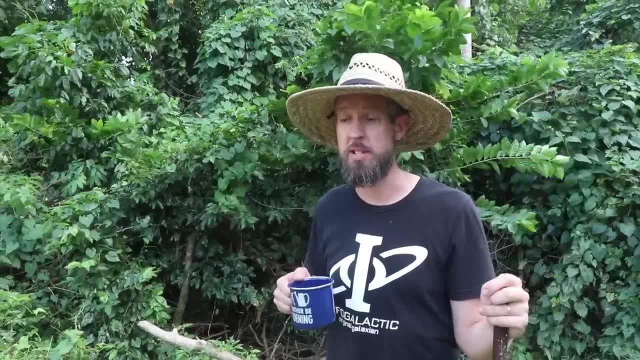 and joy. Cherokee purple. Generally throwing a little bit of compost, maybe a quarter inch over the bed right at the beginning, is enough to feed your plants throughout the season. But sometimes you maybe have some more depleted soil or some more hungry plants, so they 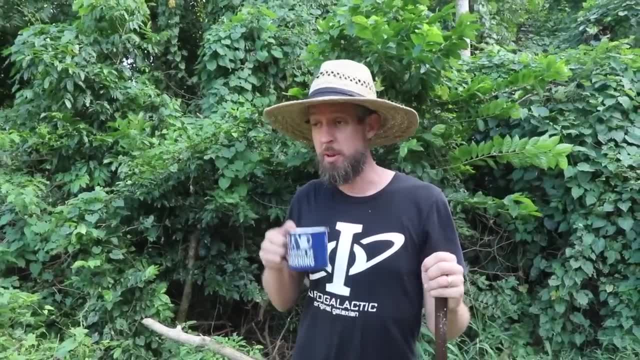 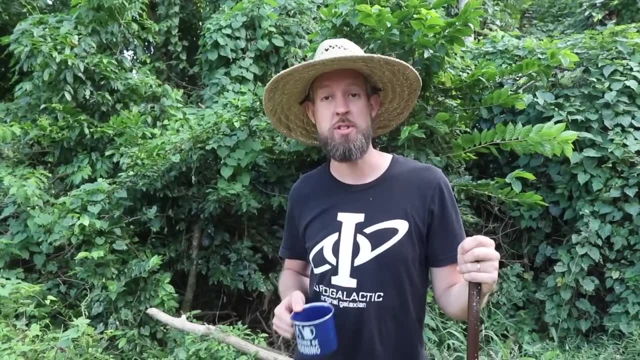 start to look a little yellow. They look like they need a little more love. If you're interested in a full presentation on feeding your garden, I'm not going to sell you one. I'm going to send you to YouTube because I posted an entire video. called Seven Ways to Feed Your Garden. I'm going to send you to YouTube because I posted an entire video called Seven Ways to Feed Your Garden. I'm going to send you to YouTube because I posted an entire video called Seven Ways to Feed Your Garden. 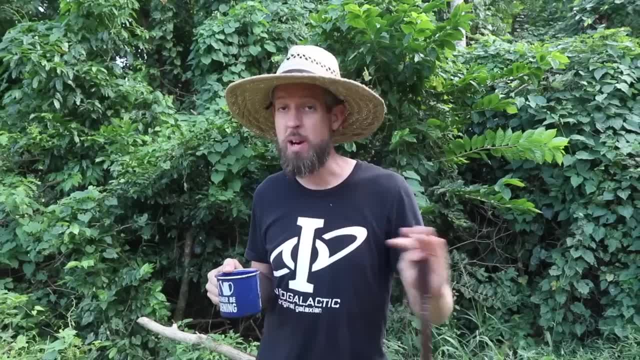 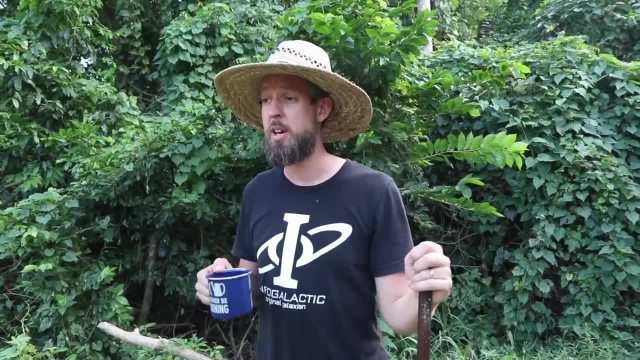 for free, which covers a whole bunch of things that you probably already have or have access to that you can use to feed and fertilize your gardens and your fruit trees for free. I told you I like to do things as frugally as possible. 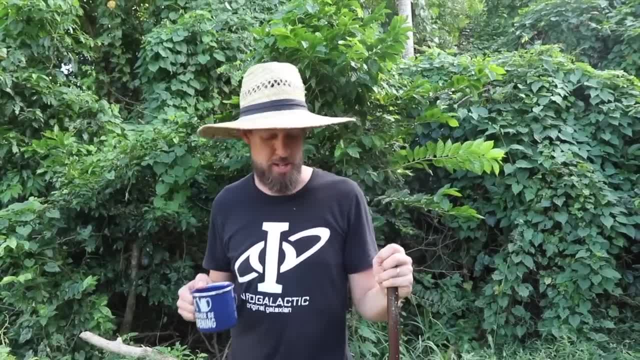 I like to make my own compost. I like to hunt down fertilizers that I can use- you know, ashes and seaweed and all kinds of other things. But you'll see it in the video. Seven Ways to Feed Your Garden for Free. 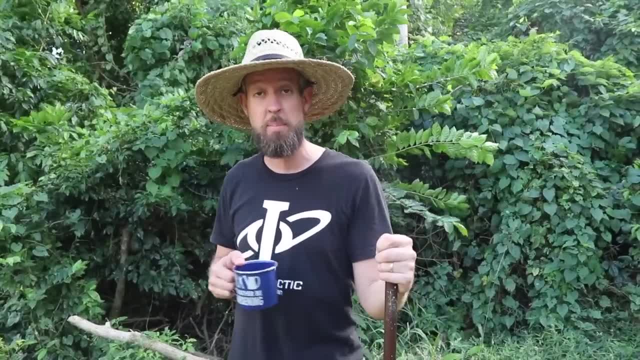 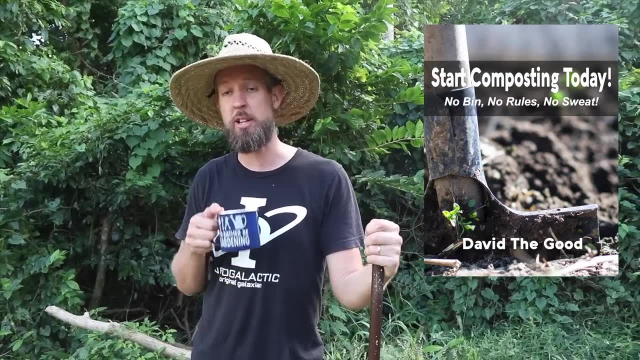 Just look it up on YouTube. And also, if you want to start composting, I have a guide on composting- super easy composting- which you can download for free. There will be a link next to this video. You can also check me out on my daily website. 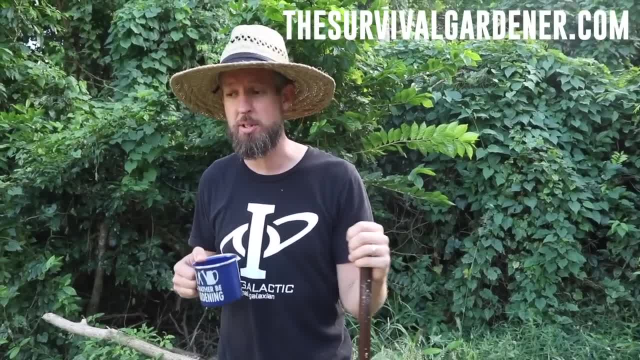 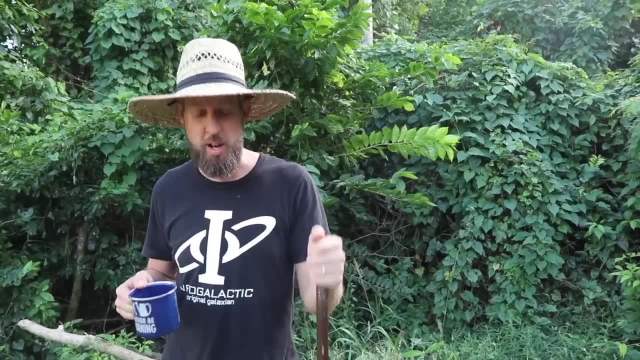 thesurvivalgardenercom, where I post a lot of articles on gardening. There's over 2,500 there. You can drop me an email, ask me questions. You can also find me on my YouTube channel, David the Good.